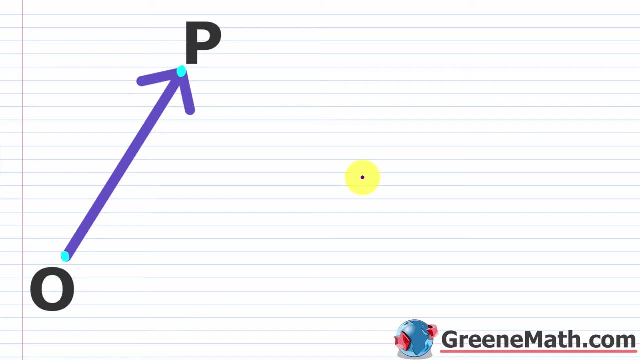 the arrowhead. Now, the way you would notate this would vary by textbook. but I would take my initial point here of o- Okay, and I would list that first. That tells me it's the initial point. Then I would take my terminal, point p, and I would list that second. Okay, that tells me that's the. 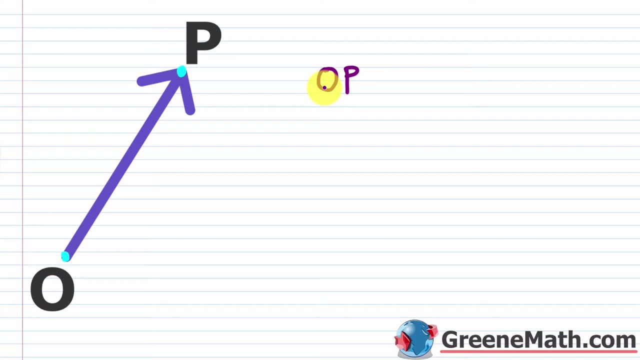 terminal point. So the order here, when you're using two letters, is going to matter, Okay, and then I want to put a little arrow on top, Okay. so this is the typical way that you will see this notated. Now you could also use a lowercase letter, Okay, something like. 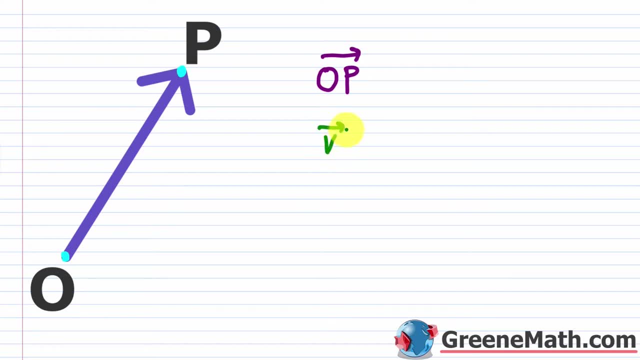 let's say v, Okay, something like that, and do the same thing, Right, but this one is going to give you the information about hey. o is the initial point and p is the terminal point. This guy just tells you you have a vector. Okay, now let's erase this for a moment. I want to show you a few other. 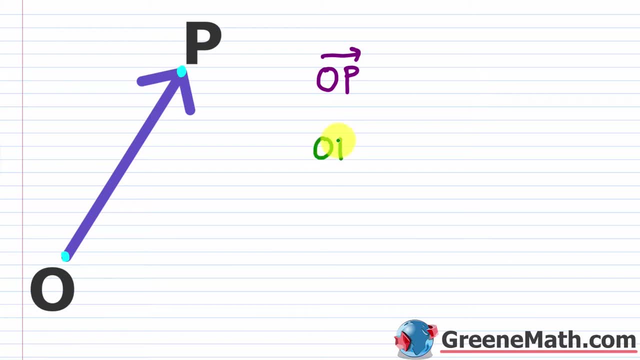 ways that you might see this notated. So in your book you might see this, Okay, where they just put that guy like that. Okay, you also might see this listed with a bar on top, And then, lastly, you might see them just use a boldface font, Okay, so you might see them just do. 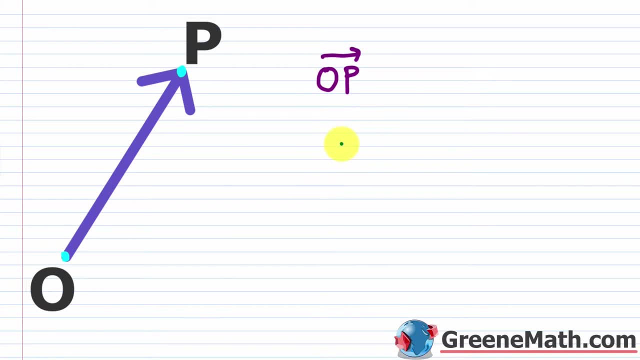 that Now I'm going to stick with this for this tutorial. In a few minutes I'm going to start talking about the magnitude or the length of this guy, Okay, and the notation for that is basically where we're going to use these vertical bars. So the magnitude of this vector op, I could put it in. 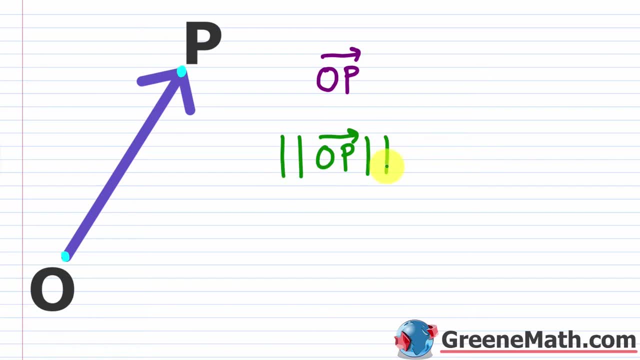 vertical bars to show that. Or sometimes the textbook will use two. Okay, two vertical bars, Okay. so go with whatever your textbook goes with. I'm going to use single bars here because that's what my textbook uses. Now, if we look at these two, 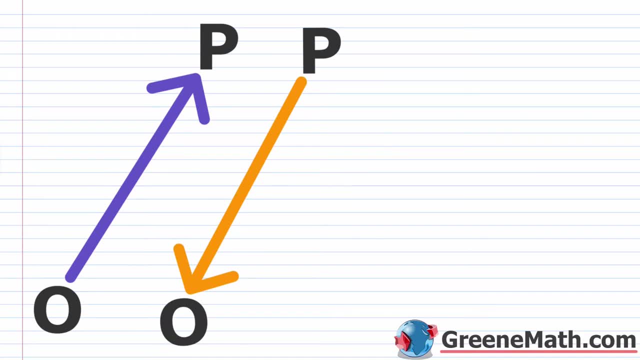 directed line segments or these two vectors. The first thing is, if I'm using the two capital letters to name them, This guy would be named op. Okay, that vector op. Here is going to be your initial point and here's going to be your terminal point. Right? so this guy would be the vector op. like this Now. 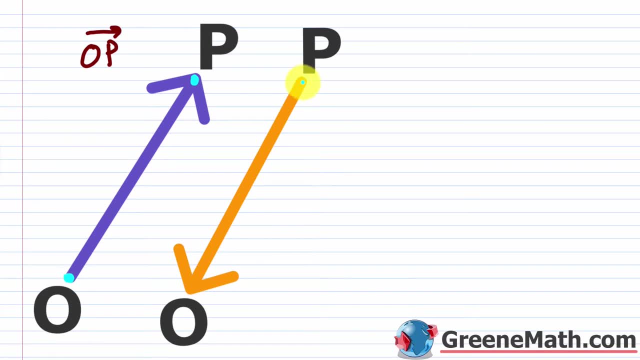 this guy is not going to be the vector op. Okay, because the initial point is here now and the second point is going to be the vector op. Right, these have different directions. Look at the way the arrowheads are facing. Okay, this one is facing this way. This one is facing this way, Okay, so 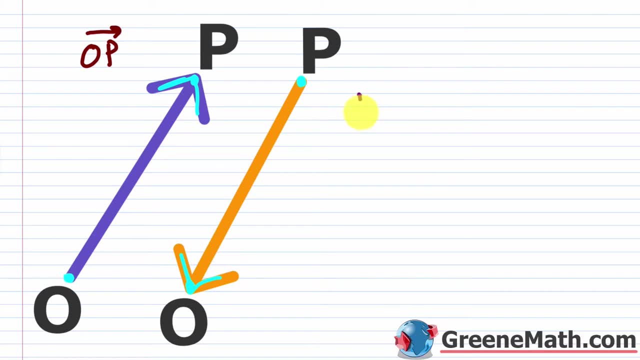 different direction, same magnitude, But this one's going to be called po, So this will be vector po. Okay, let me get rid of this and make that a little bit better. Now I can say right here that this vector op is not equal to this vector po, And the reason they're not equal is because for two 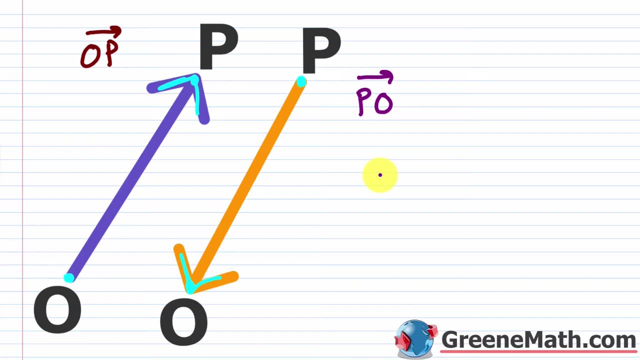 vectors to be equal they have to have the same magnitude or the same length, And also they have the same direction. These do not have the same direction, even though they do have the same length. So I can say this vector op is not equal to this vector po. All right, so now let's think a. 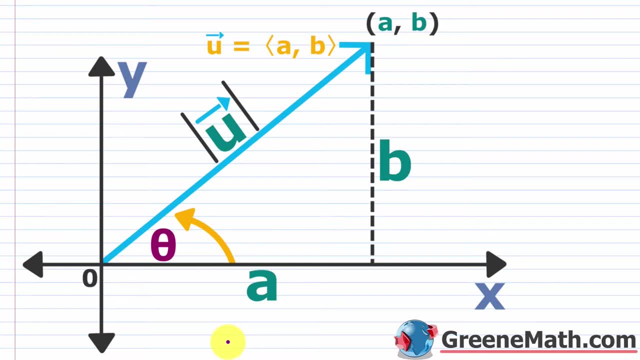 little bit about the magnitude and how we find that, Also something called the direction angle and then the component form. Okay, so let me start with the component form, because I think everything kind of builds off that. So, first and foremost, you see on this sketch the way this is drawn. 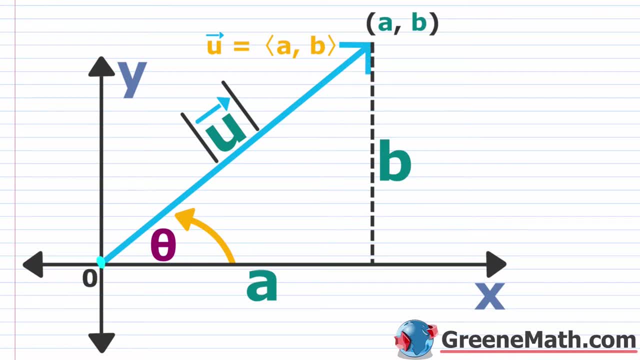 we have our initial point at zero comma zero, or the origin. Okay, so let me label this: This is zero comma zero. Then we have our terminal point. Our terminal point at this a comma b. Okay. so because this guy has an initial point at zero comma zero, we call this a position vector, Okay, or we say it's. 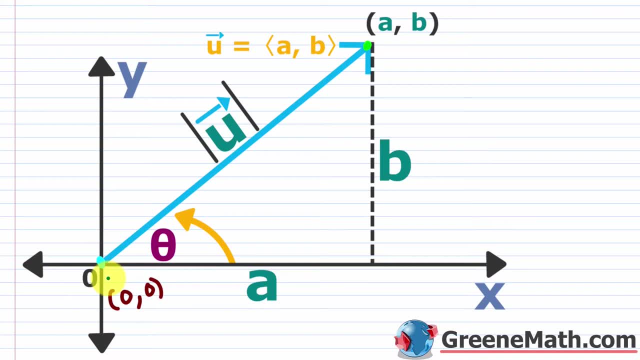 in standard position. Now, when you have a position vector or when it's in standard position, you can just list the coordinates for the terminal point. That's all you need, because you know the initial point is at the origin. Okay, you don't need any more information. So the way we list this is called. 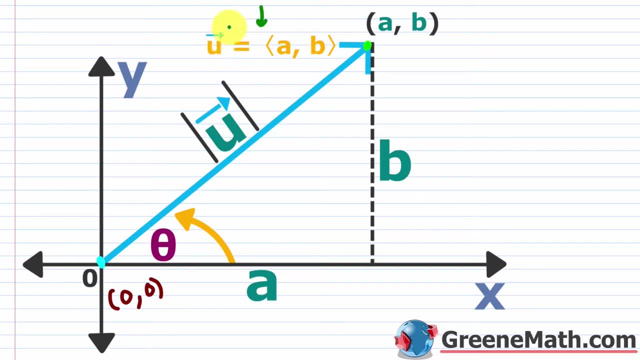 component form. So the way we list this is called component form. The way we list this is called component form. Okay, so here I've named my vector u, So the vector u is equal to. you'll see, we have these angle brackets here and we're just listing the a and the b. All this is is the x and the y. Okay, from the. 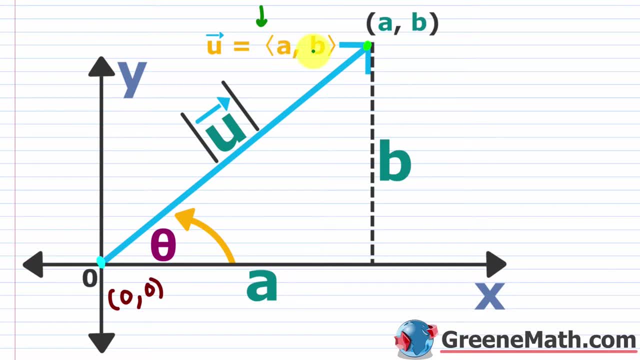 ordered pair. We're just listing it inside of those angle brackets. So if I said that I had a vector, u, okay is equal to, let's say, I had three comma four. Well, I know- and I didn't make those brackets very well- I know that the x location is three and the y location is four. in terms of the point, Okay, the 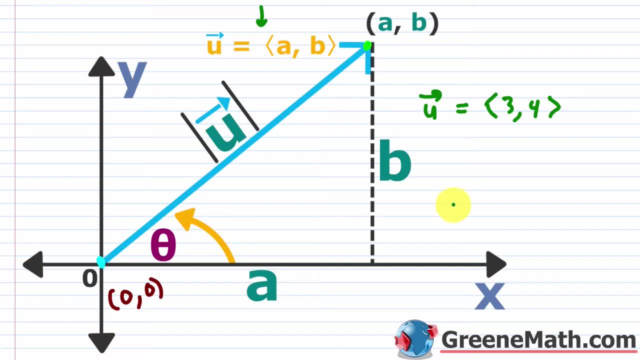 vector u is equal to zero comma zero, and then I would draw a terminal point at three comma four, Okay, and I would just draw a directed line segment. That's all I'm doing, Okay. so, additionally, we also have something called. let me just erase all this. We don't need this anymore. We also have something. 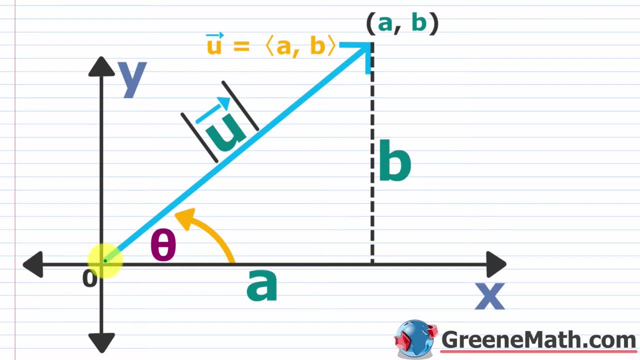 called the magnitude of the vector, which we already talked about. It's the length of this guy, Right? so if I said what is the length of this guy right here? So if I just drew this line right here, What is the length of that? Well, again, normally if we form a right triangle, Okay. 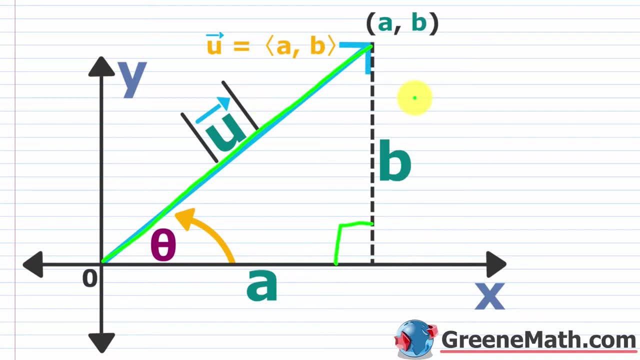 we can do this with the distance formula. Let me just call this side c for a moment. So I'll say c, which is the hypotenuse typically. Okay, so c, I'll say c squared is equal to this: a squared plus b squared. So we know if we want c by itself, we say c is equal to the principal square root. 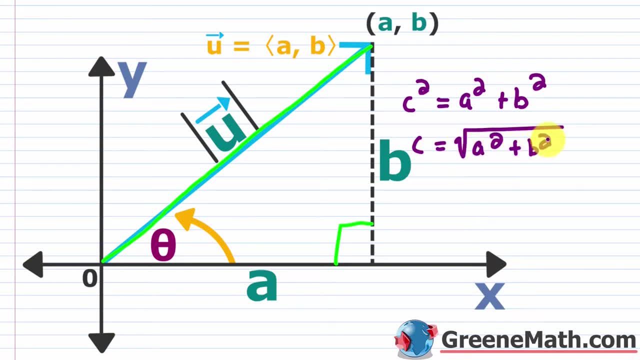 We don't need the negative one of a squared plus b squared, Okay, well, now instead of c, I just have the magnitude of u, So I'm just going to replace that. Okay, that's all I'm doing. So the magnitude of a squared plus b squared. Now, in the case where you're not given a position vector: Okay. 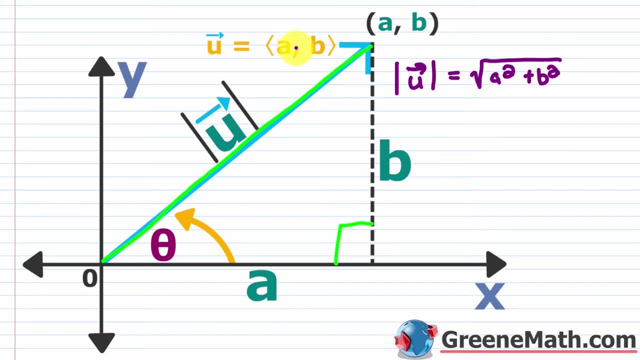 you're going to either have to put it into component form or use your original distance formula. Right, remember, the distance is equal to. you have the square root of. you have the quantity x sub 2 minus x sub 1 squared, plus the quantity y sub 2 minus y sub 1 squared. Okay, in this, 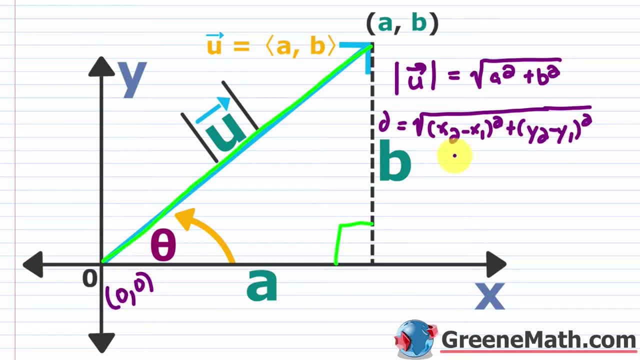 particular case, your point down here is 0 comma 0. So if you do this, it just becomes a. this is going to be a right for the x location: a minus 0, which is a being squared then plus this would be b minus 0.. 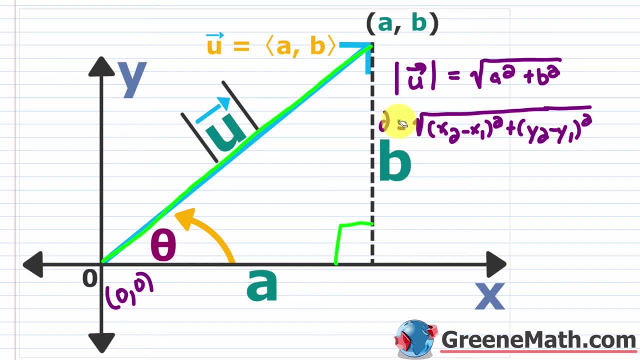 Okay, so it would be b just being squared. Okay, so that's all it is. So let's get rid of this and we see how to find the magnitude. Now let's talk about how to find the direction angle, because this one's quite confusing. Okay, so, basically, the direction angle is going to be this positive angle. 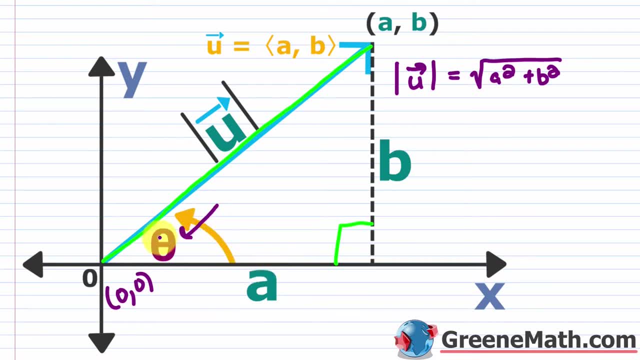 theta here between the x axis, Okay, and our position vector. Now it turns out that it's pretty easy to find this overall. Okay. need to do is some basic trigonometry In these problems, if you're given a and you're given b. so 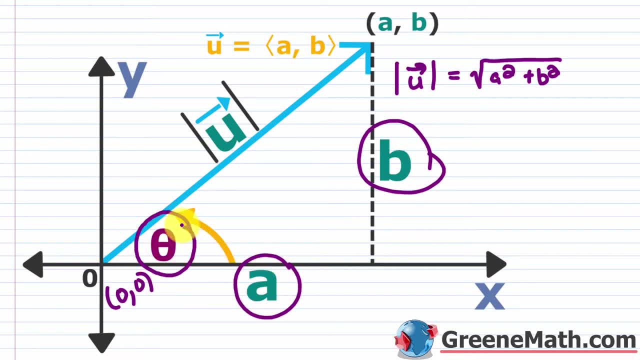 if you're given this and you're given this and you're trying to find this angle here, what can you do? Well, remember, the tangent is y over x. okay, in this case, it would be b over a. so the tangent okay, of this angle, theta, is going to be equal to b over a, and you could say specifically where a 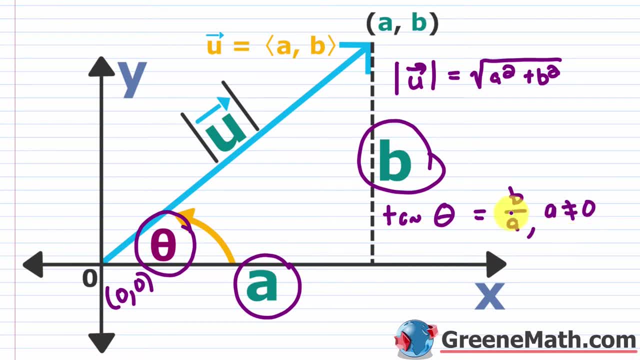 does not equal zero. okay, but you're going to have to do more work than this because, again, if you involve the inverse tangent function, remember that guy is going to only return something from quadrants one or four. okay, so you have to basically think about this by getting a reference angle in 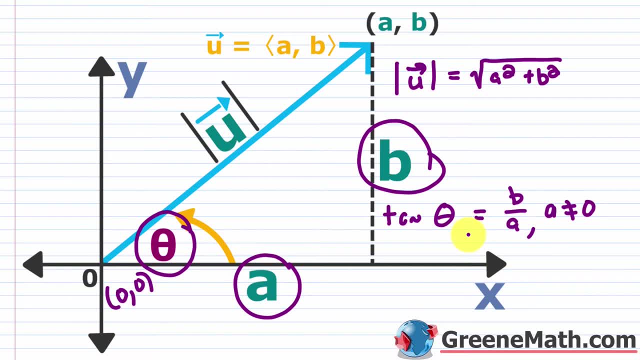 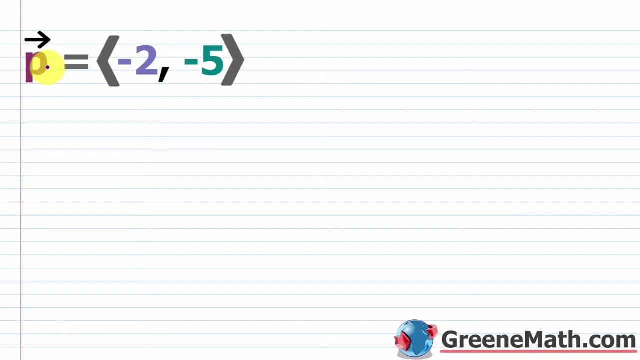 most cases, and then figure out what quadrants are in. so you're going to have to do a bit of detective work. Okay, let's go ahead and take a look at a simple problem. so I'm given a vector p, okay, and the component form gives me a horizontal component of negative two and a vertical component. 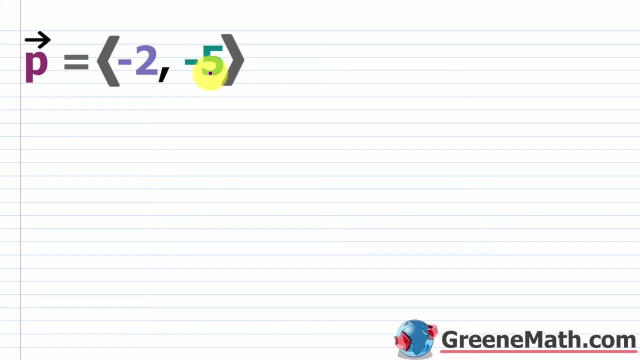 of negative five. okay, so if you wanted to sketch this guy, you would have one of these two and you would have a horizontal component of negative two and a vertical component. one point at the origin, okay, at 0 comma 0,. okay, that's your initial point, and then you'd have a. 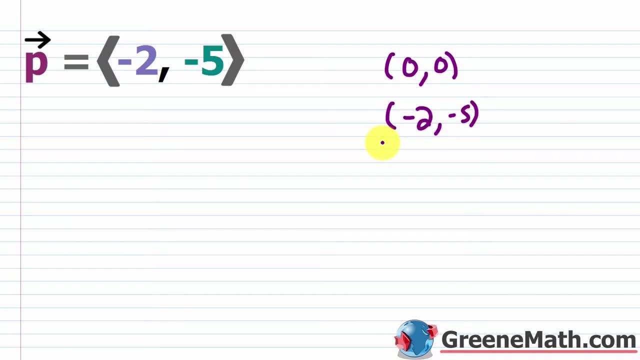 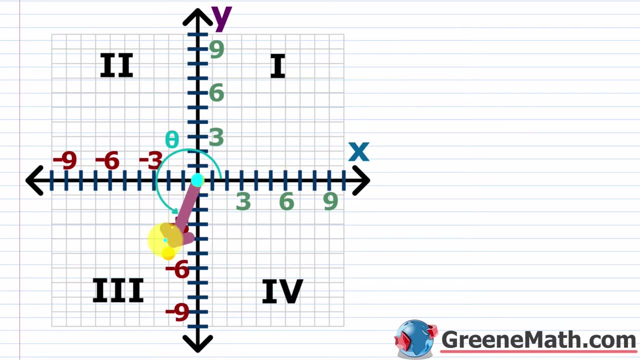 terminal point at negative 2 comma negative 5.. Let's just look at the graph real quick. So you see your initial point is here at 0 comma 0, okay, and your terminal point: you're going two units to the left and five units down. so it's at negative 2 comma negative 5, okay, it's just a directed. 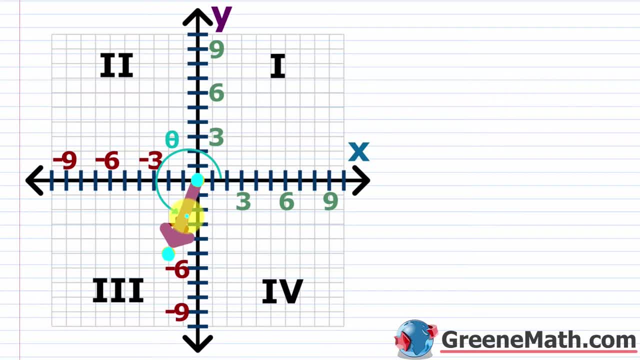 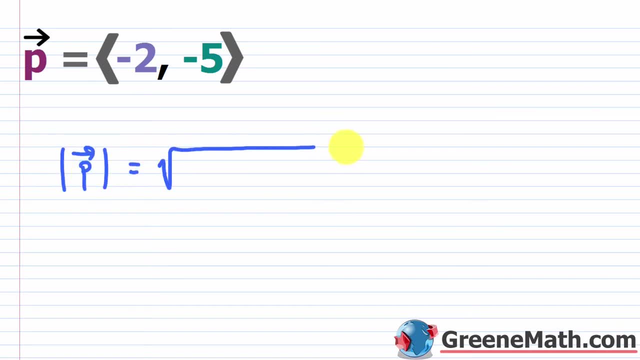 line segment. that's all it is. So if we think about the magnitude of this guy, again that's pretty simple. The magnitude of this vector p is going to be equal to the square root of. again, you're going to square each one and then sum the results, So I'd have negative 2 squared, okay. 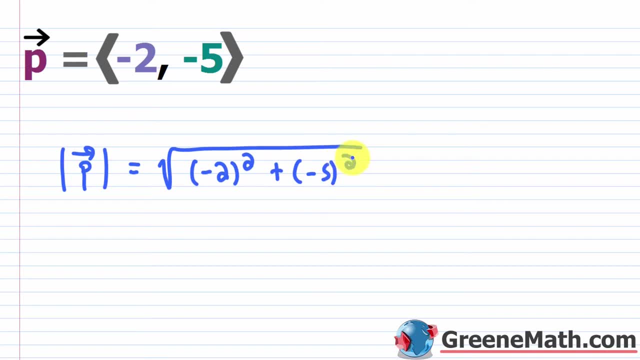 make sure you put in parentheses. then, plus, you'd have negative 5 squared, okay. so you want the negative and the 5 being squared and the negative and the 2 being squared. Make sure you use parentheses, Okay. so what I'm going to do here is I'm going to say that the magnitude of this vector 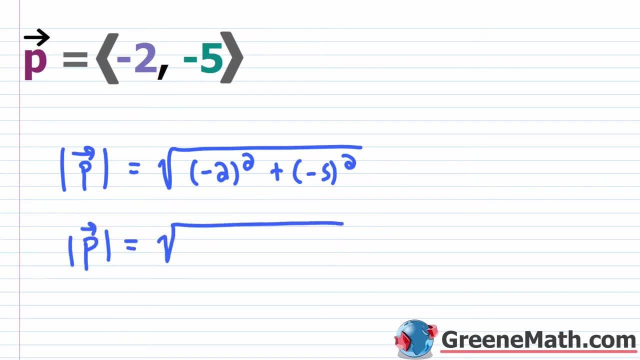 p is going to be equal to the square root of. let's go ahead and say negative 2 squared is 4,. okay, plus, if you do, negative 5 squared, that's 25,. so that would be 4 plus 25 or 29,. okay, So this. 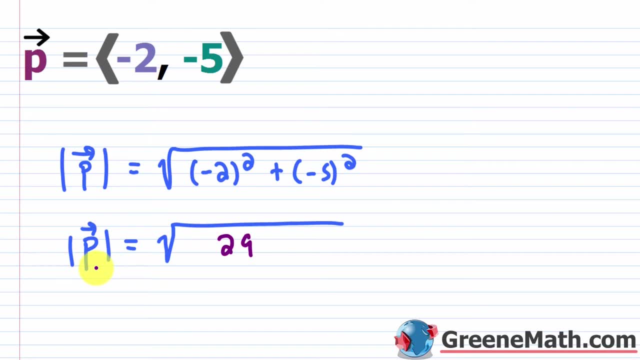 is the magnitude of this vector p? okay, nothing more than just the distance form. Now, if we think about the direction angle, this is where things get a little bit more tricky. Let me get this out of the way. okay, If I go back, I want you to observe a few things and I can just erase this. 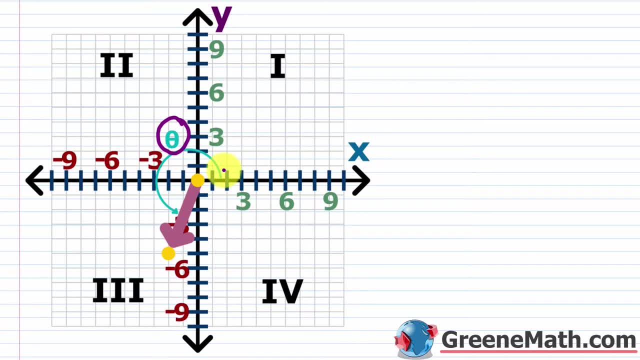 We're trying to find this angle theta here. okay, If we think about this, if we swing this around, we see that this guy is in quadrant 3, okay, So in quadrant 3, if we think about tangent, it's going to be positive, right? Remember? 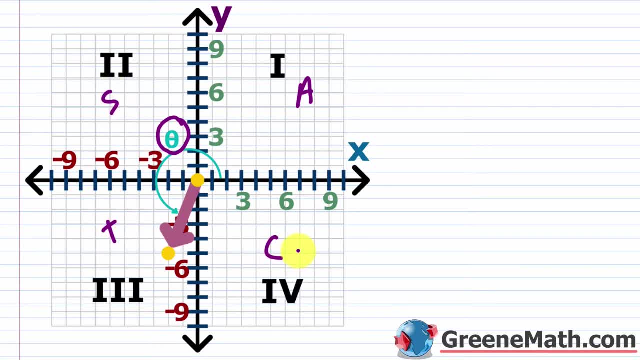 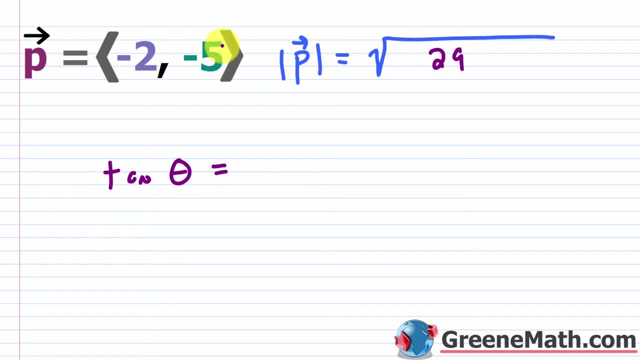 this. all students take calculus, okay, But if I use my inverse tangent function, I'm not going to get something in quadrant 3, I'm going to get something in quadrant 1.. So if I go back and I think about this guy, remember that tangent of theta is equal to you. take your y value or your. 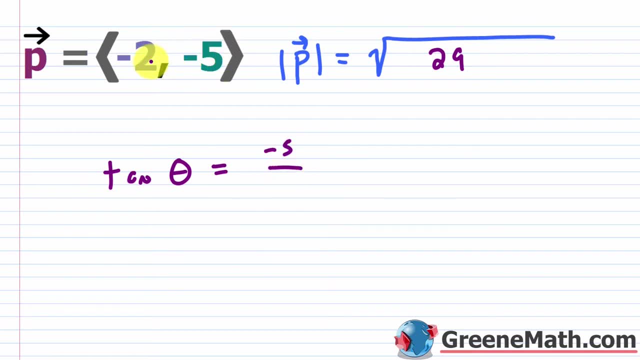 vertical component, which is negative 5, over. you take your x value or your horizontal component, which is negative 2.. And so basically I could say the tangent of theta is really equal to 5, halves right. So if you do the inverse tangent on this, so you do tangent inverse of. 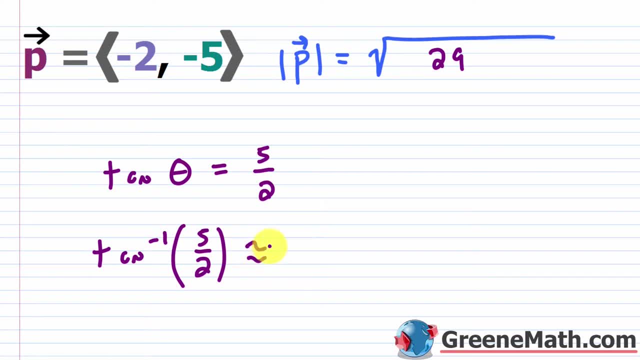 this 5 halves, you're going to get something. let's say it's approximately, I'll go with 68.2 degrees. okay, So 68.2 degrees, And again I'm just rounding. So if I know that, this guy right. 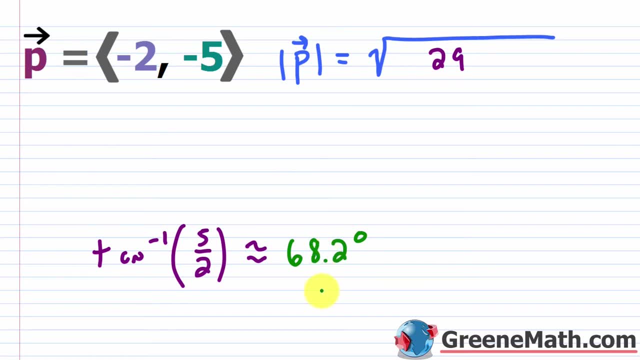 here is a result of the inverse tangent function. well, again, if I'm in quadrant 3, this is not my angle, okay, So people mess up all the time and say, okay, well, theta is going to be 68.2 degrees. 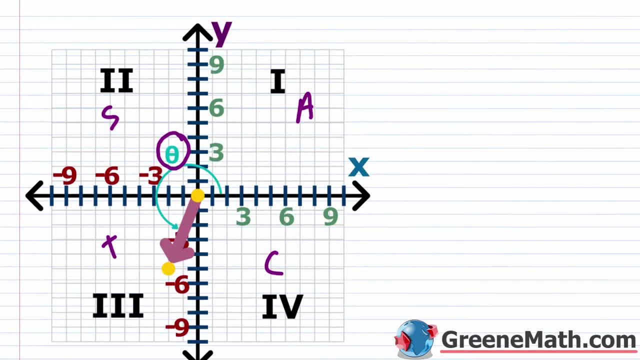 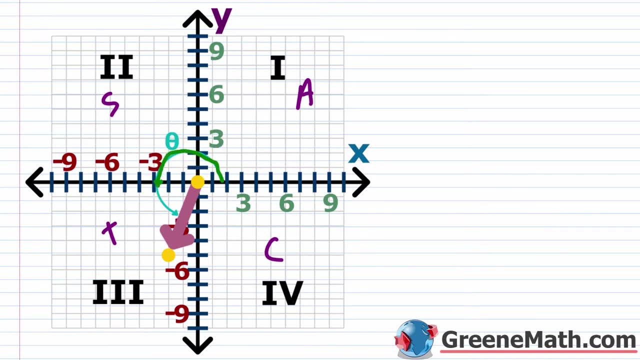 that's wrong, because I'm in quadrant 3.. So if I go back, you can visualize what's going to have to happen here. okay, I've got to go 180 degrees first, okay, And then I also need to add on top of: 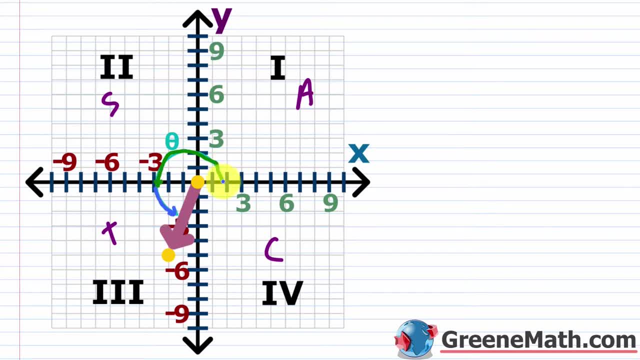 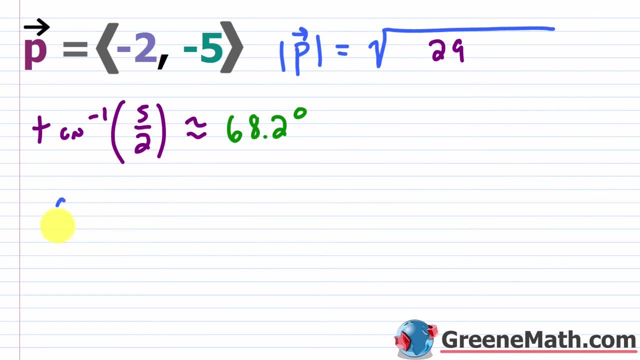 that, that reference angle to get the rest of the way. okay. So I need 180 degrees plus the reference angle to get this angle here, theta. So if I go back, all I want to do is say theta is going to be. 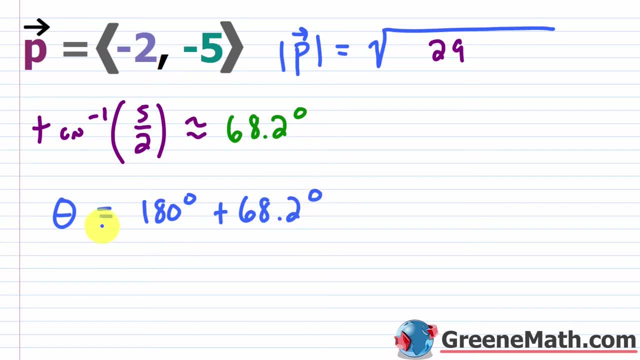 degrees plus 68.2 degrees, And you can put approximately here. let's just leave the equals for a moment. I'll just go ahead and change it in the end. So this is going to be what It's going to be: 248, 248.2 degrees. okay, So let me erase this. we don't need this anymore, So that's our. 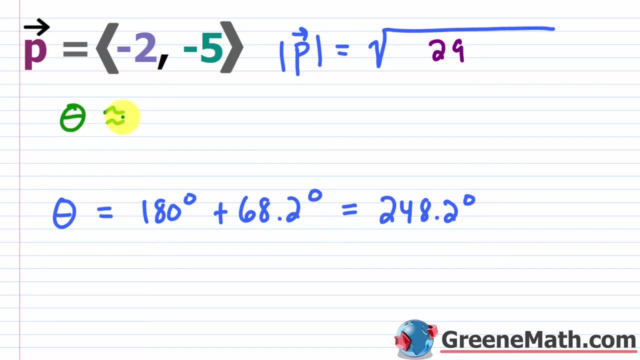 direction angle. It can be a little bit confusing. Just make sure you understand what quadrants you're going to be in and that when you're working with the inverse tangent function, you're getting something in quadrant 1 or 4 only. okay, So let's go ahead and put this as: 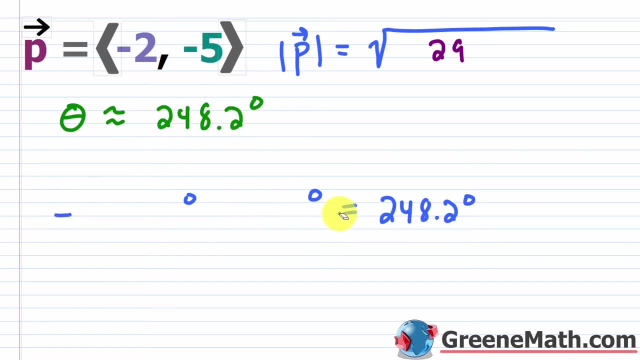 248.2 degrees. okay. Also, I should note that if you get something in quadrant 4 from the inverse tangent function, remember it rotates clockwise to get that. okay, So that's not going to be your angle either. okay, So you got to do a lot of detective work when you're doing these, Okay. 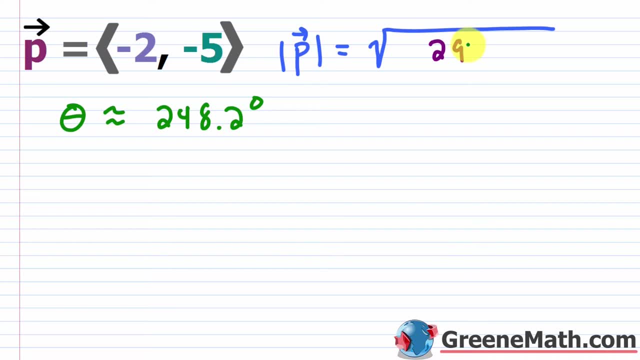 so we found that the magnitude of our vector P is a square root of 29, and the direction angle is approximately 248.2 degrees. All right, let's look at another easy one, and then I'll show you something that's a little bit harder. So we have this vector V here, okay, and the whole thing is: 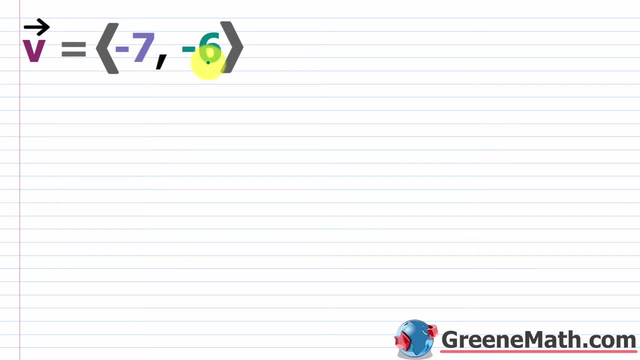 horizontal component is negative 7, the vertical component is negative 6.. So again, if I wanted to find the magnitude, so the magnitude of this vector V, this is equal to the square root of. you could say negative 7 squared plus negative 6 squared. okay, like this. So the magnitude of 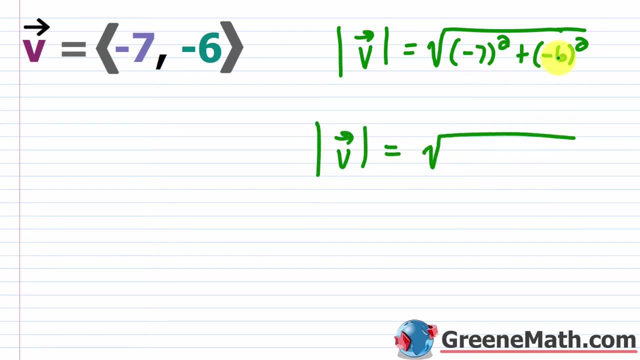 this vector V is equal to. let's go ahead and say: this is 49 plus 36, so that's going to be 85 in here. So basically the square root of 85, really can't do anything to simplify that, so that's. 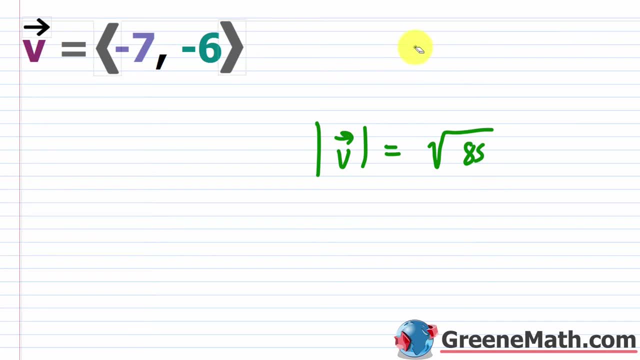 going to be our answer. okay, Let's get rid of this and let's just drag this up here And again. finding the direction angle usually takes a little bit longer because you got to plug some stuff in. Now, if I think about this again, the tangent of theta is equal to. again, it's going to be the 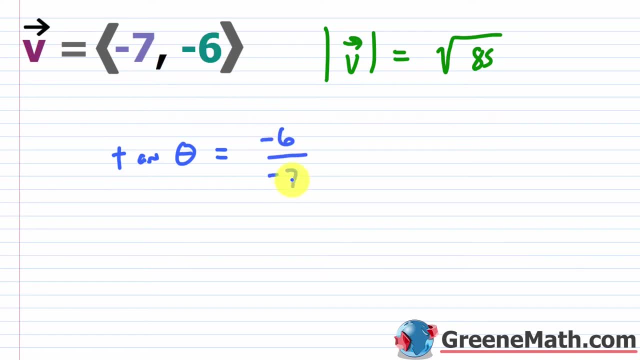 vertical component, negative 6, over the horizontal component, negative 7.. Might as well just say this is 6 sevenths. But again, if I do the tangent inverse of this guy right here, I'm going to end up with something in quadrant one. Where is this guy at? If I graph it again, my 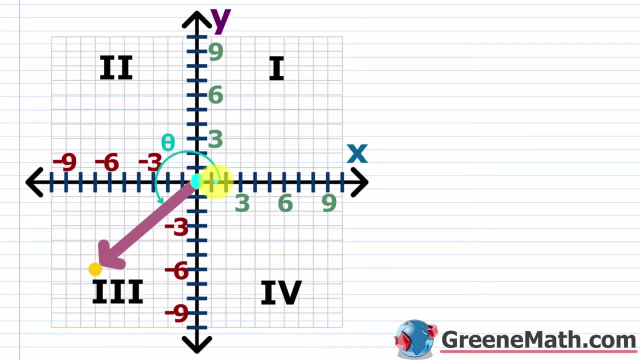 initial point is here, at 0 comma 0. My terminal point. I go 7 units to the left and 6 units down, So it's at negative 7 comma, negative 6, okay. So if I look at this guy, I'm going to be in quadrant. 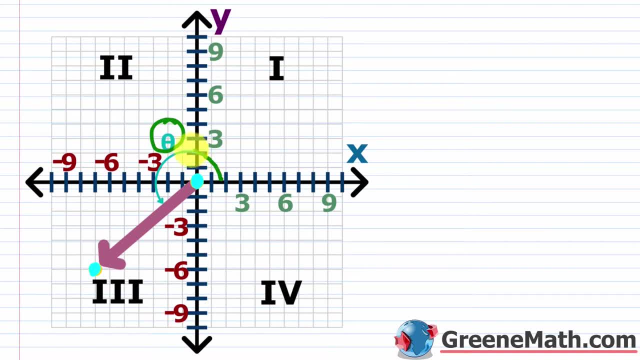 3, right, This is the angle theta that I'm trying to find, So I've got to swing all the way around here. So remember what we have to do. We've got to go 180 degrees and then plus that reference. 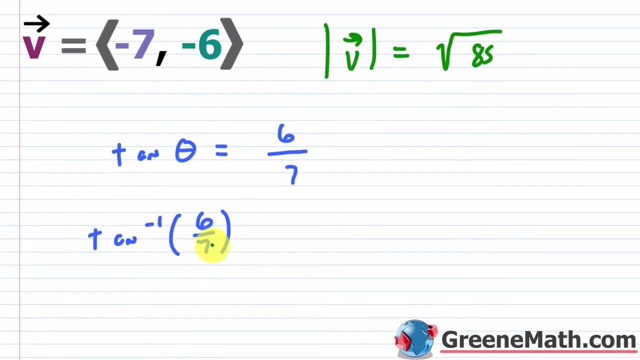 angle to get there. So let's go back and let's punch this into the calculator and that's going to give me the vector, vector V. I'm going to go 180 degrees. So again, when you think about this, I'm going to say that my direction, angle, theta, I'll just put approximately here: I'll go 180. 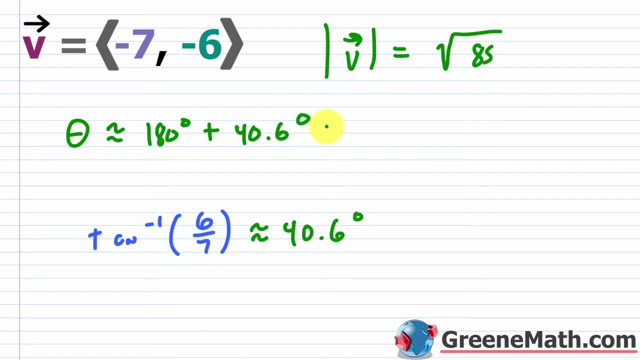 degrees plus I'll go 40.6 degrees. okay, So what is this going to give me? It's going to give me 220.6 degrees. So let me erase all of this and let's just put our answer here. So: 220.6 degrees. 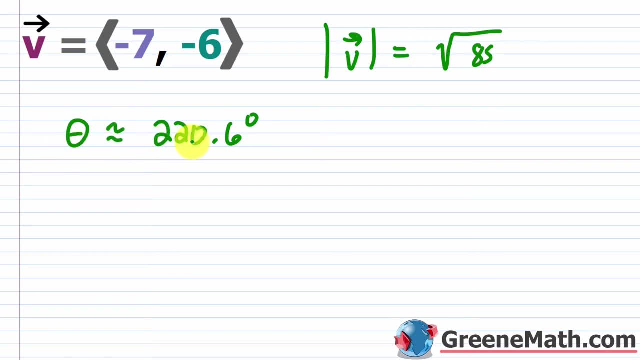 So, again, the magnitude of this vector V is square root of 85.. The direction angle is approximately 220.6 degrees. all right, let's take a look at another example. so this one involves a little bit more work. so we have this vector pq. okay, so we know, because of the way this is listed, right. 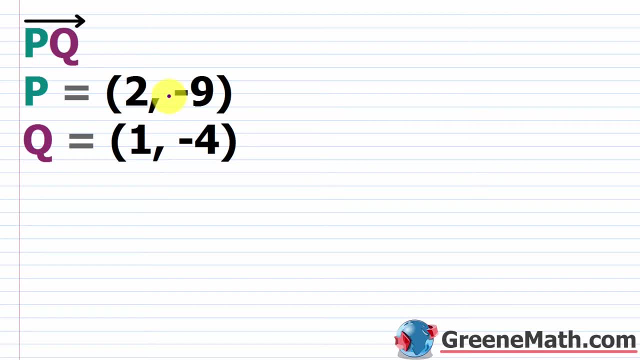 from the beginning of the lesson we said that the first letter here, p, is the initial point, right, so the coordinates are 2 comma negative 9. the second letter, q, is the terminal point, so the coordinates 1 comma negative 4. okay, let's go ahead and sketch this real quick. so if we look at this guy, we go. 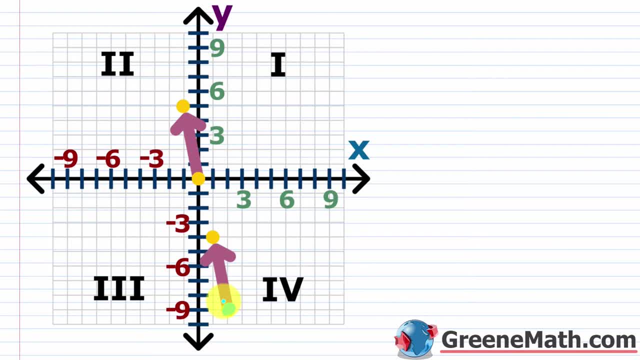 2 units to the right and 9 units down. so that's right here. this is going to be your p, or your initial point. again, this is 2 comma negative 9, and then the other one. here, if we go 1 unit to the right and 4 units down, we're going to be right there. so that's going to be q. okay, that's our. 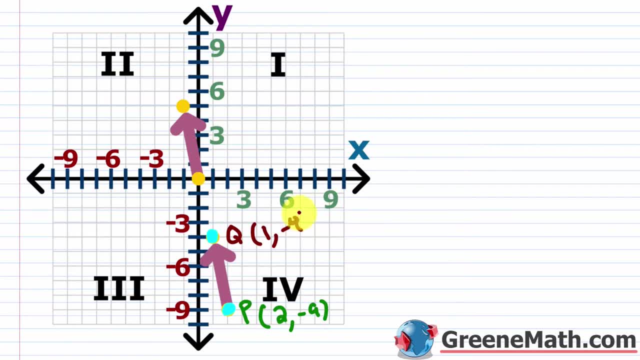 terminal point. so again, this is 1 comma negative 4. so the first thing you want to do if you have a problem like this, you want to put it in the component form again. this is where the coordinates for the terminal point are given only because the initial point is the terminal point. 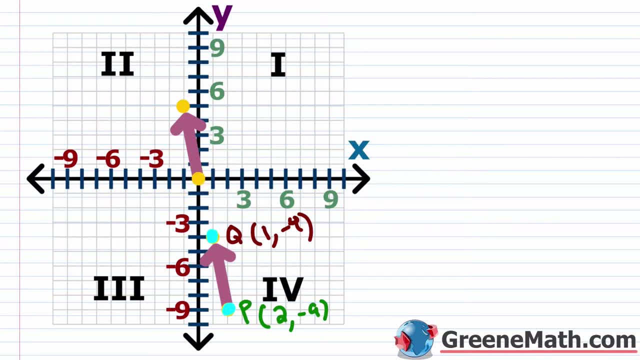 is at 0 comma 0 or the origin. okay, so you'll see that i already have this graph right. so this is 0 comma 0, or the initial point, and then you'll see the terminal point is at negative 1 comma 5. so where does this come from? how did i get that? well, if you go back here, it's a simple little. 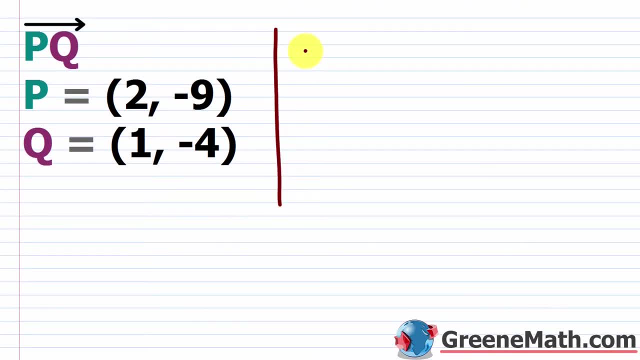 formula. all you really want to do. let me come over here and say for this vector, pq, okay. and sometimes books will rename this with a lowercase letter once it's in component form. that's up to you. if you want to do that, okay, i'm going to keep it as it is. 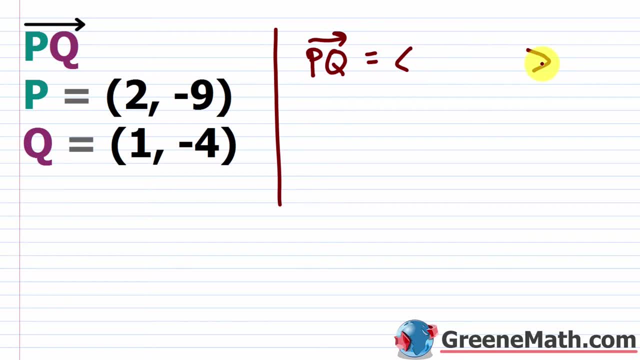 so i'm going to say this is equal to. i'm going to put my little angle brackets there and basically to get this position here, you go with the x value from your terminal point, okay. so i'm going to take this one right here, okay, and then i'm going to subtract away the x value from your initial point. 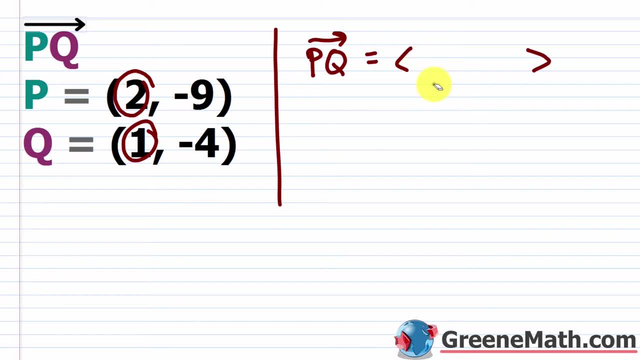 so minus 2. okay, so 1 minus 2 gives us negative 1. now you want to go in that order. i know sometimes when you work with these formulas, if you reverse them they come out fine. but in this case you want to go from the terminal point. okay, you want to start with that, and then you want to go from the 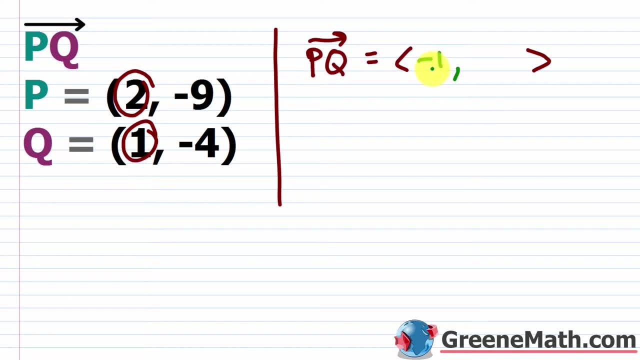 initial point. okay, so the same thing with x's and y's. so with this guy i'm going to take this one minus this one. okay, this is from the terminal, this is from the initial. so i want to go negative 4 minus a negative 9, which is negative. 4 plus 9, which equals 5. okay, so that's where that terminal. 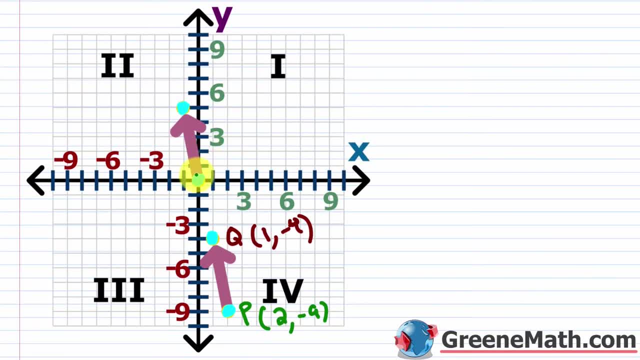 point of negative 1 comma 5 came from. you go back, you see this is one unit to the left and five units up. so this is negative 1 comma 5 and you can call this the point q. okay, now the point p is at the origin. okay, and because of this, a lot of books again will just rename this as the vector v or u or 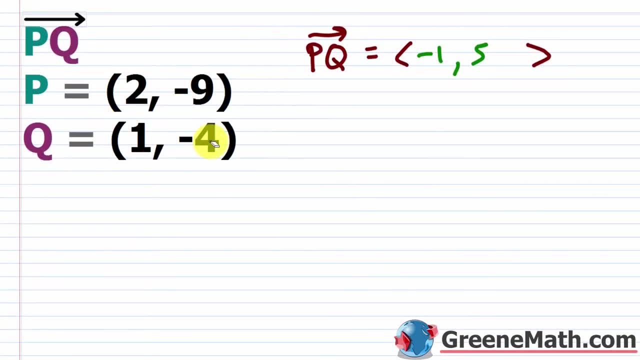 whatever they want to do, i'm just going to keep it like this. now, if you want to find the magnitude- okay, and make a little little border here- of this vector pq, okay, what i'm going to do is just take the square root of i'll take this first guy, negative, 1 squared, plus the second guy, 5 being. 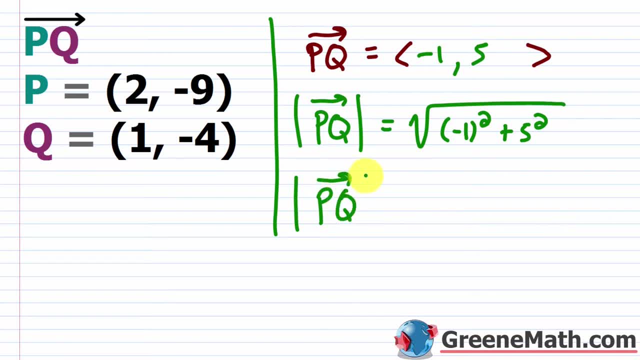 squared. okay. so the magnitude of pq- okay, like this is going to be the square root of negative. 1 squared is 1 plus 5 squared is 25, so this can be 26. so it's just a square root of 26. now, if you wanted to come over here and use these points, 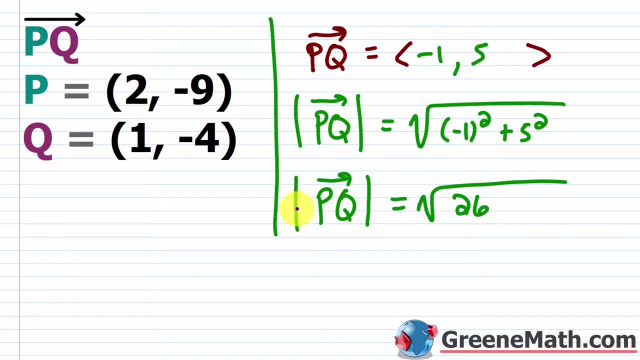 again, you could plug into the traditional distance formula. you could say: and i'm just going to label this as the magnitude of this pq guy, okay, i'll show you, it's the same. basically, you're going to subtract this guy minus this guy, so x sub 2 minus x sub 1, so it's going to be 1 minus 2. let me let 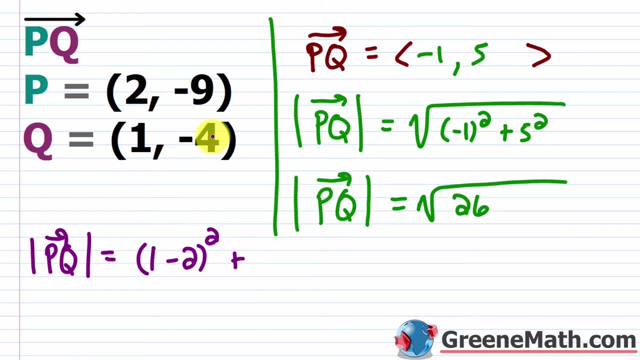 me write this out. so 1 minus 2, this is squared. then plus- you're going to do this guy that minus this guy. so negative 4 minus the negative 9 is plus 9. okay, this is going to be squared and we want the square root of this guy, okay, so notice that we already did this to find these. 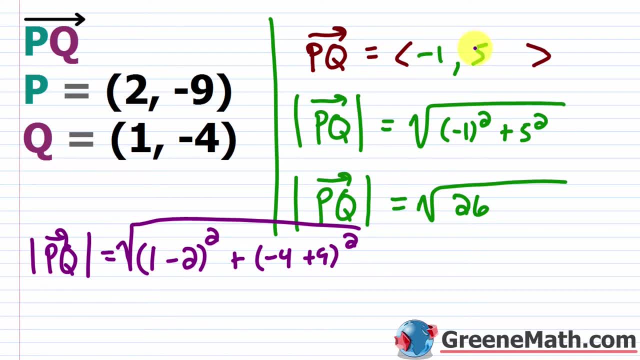 guys right here. okay, so we're a step ahead, right? so that's why we do this first and then we don't have to do all this, okay, so 1 minus 2 is going to be negative 1, so it's negative 1 squared, which. 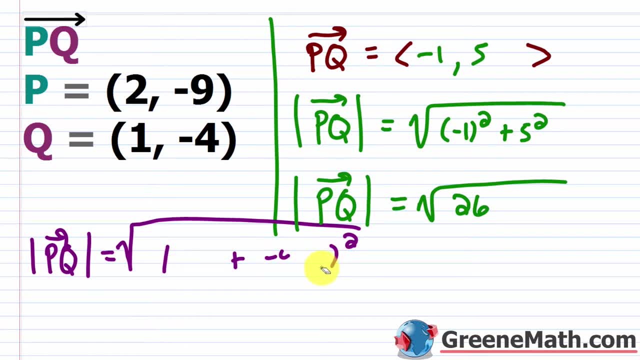 you know, is 1, and then negative. 4 plus 9 is 5. 5 squared is 25. so this becomes square root of 26. okay, just like it is over here. okay, so you see, it's the same magnitude in each case. now let's. 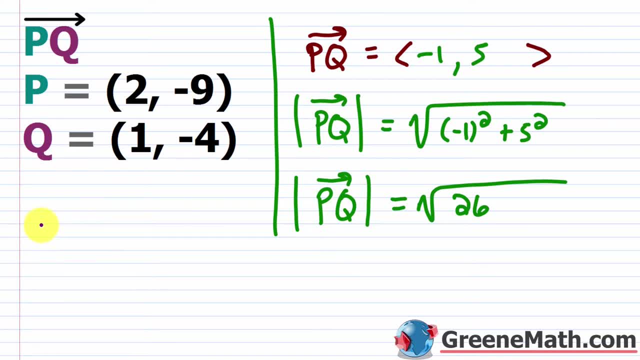 do that. well, again, let me actually erase this. let me just say that the inverse tangent- i think we can kind of skip ahead a bit- the inverse tangent of what well, i'm going to take the vertical component, which is 5, over the horizontal component, which is negative, 1, which really i could just 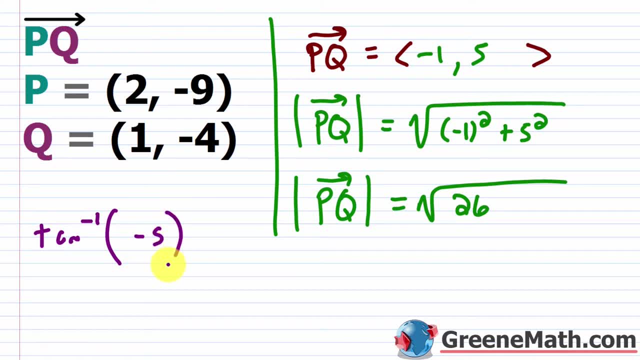 write as negative 5. okay, like this: now, when you talk about putting a negative as the argument for this inverse tangent function, you're going to get something in quadrant 4, okay, so in this particular case, if we think about this, this horizontal component is negative, this vertical component. 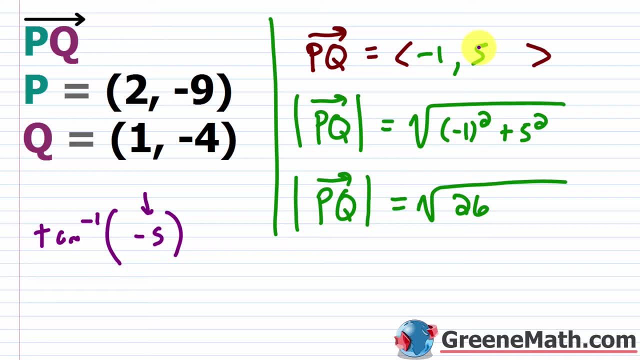 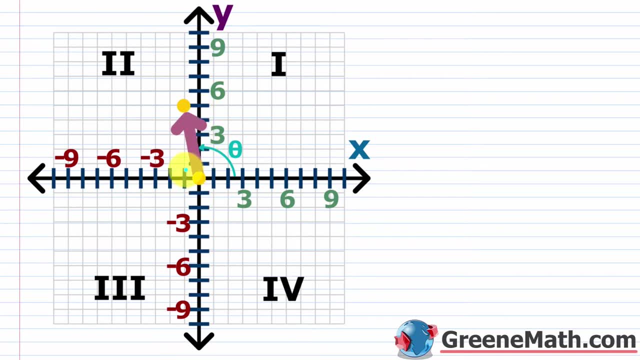 is positive if i think about it. where am i going to be? i'm going to the left and i'm going up, so i'm going to be in quadrant 2. if you want to see this graph on its own, you'll see again. my terminal point here is that we go one unit to the left and we go five units up, and you see, i'm in quadrant. 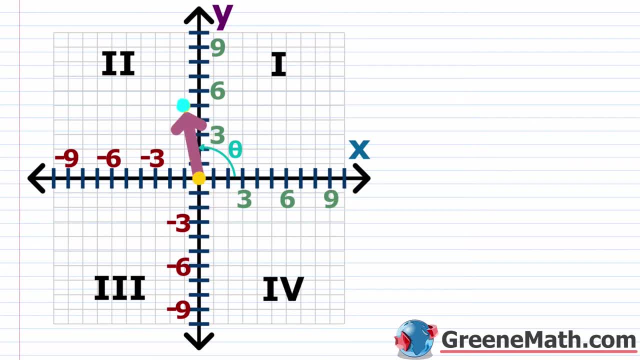 2 here. okay. so basically, when i do my inverse tangent function, i'm going to end up with something in quadrant 4 and also i'm going to be rotating clockwise, okay. so i want to just take the absolute value of that and think about that as my reference angle and then what i want to do. 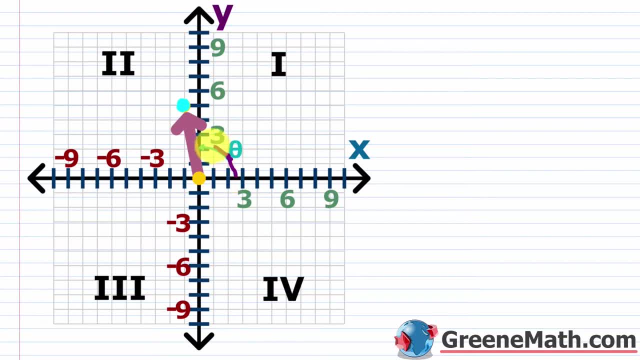 is. i'm going to take the absolute value of that and think about that as my reference angle in this particular case. i would think about the fact that, okay, if i had an angle of 180 degrees, i want to subtract off and go back by the amount of the reference angle. right, so i want 180 degrees. 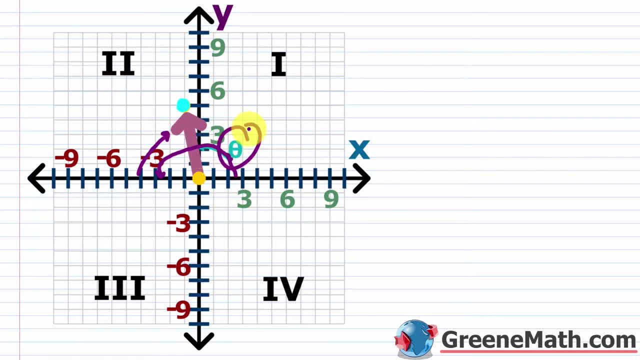 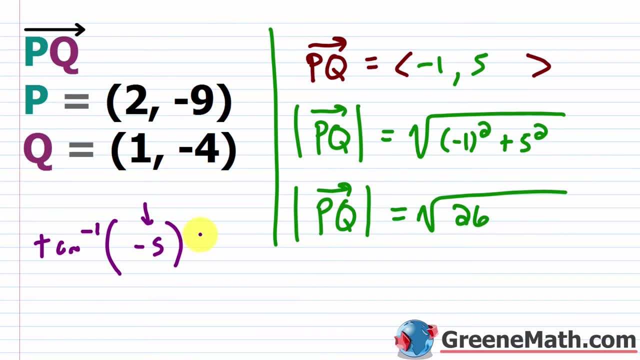 minus the reference angle to get this angle theta here. okay, this angle theta here. now let's go back. so i'm going to get about negative 78, point, let's say 69. so let me kind of slide this down because i don't think it's going to fit. so i'll put it's approximately negative 78.69 degrees, now again. 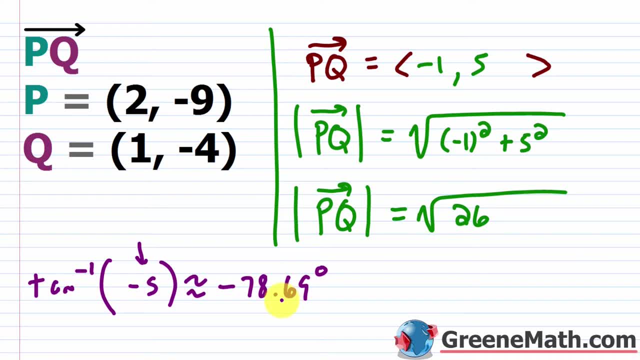 what i want to do is i want to put this angle here. and i'm going to put this angle here, and i'm going to do is i want to think about this in terms of absolute value. so in quadrant 2, i want an angle with a reference angle of 78.69 degrees. so all i'm going to do get rid of the negative sign. i'm going 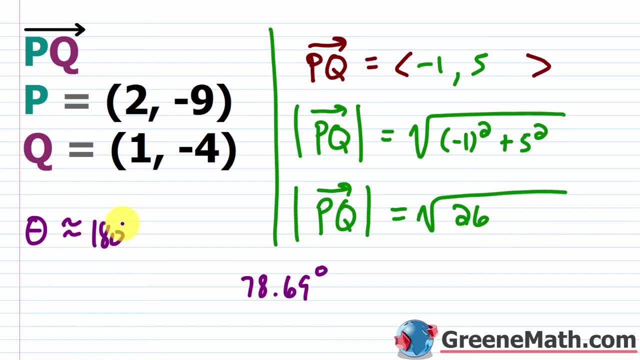 to say, theta is approximately 180 degrees minus this 78.69 degrees, and that's going to be about 101.31 degrees. so let's just erase this and put it's about, or approximately, 101.31 degrees. all right, for the last two examples we're basically going to reverse things. so now we're going to be given the 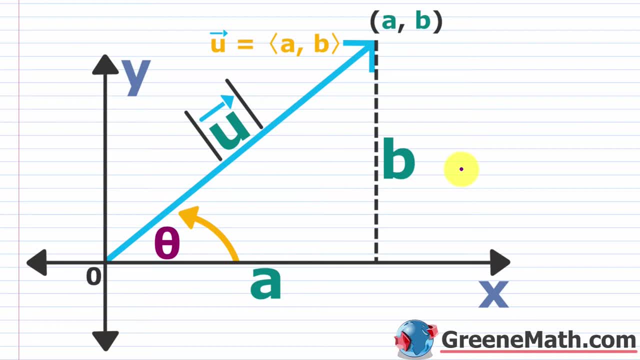 magnitude of a given vector and we're also going to be given the direction angle and we have to come up with the component form, okay, so let's think a little bit about this angle, theta, and let's think about if i had this guy b and i had this guy a. let's think about some relationships. 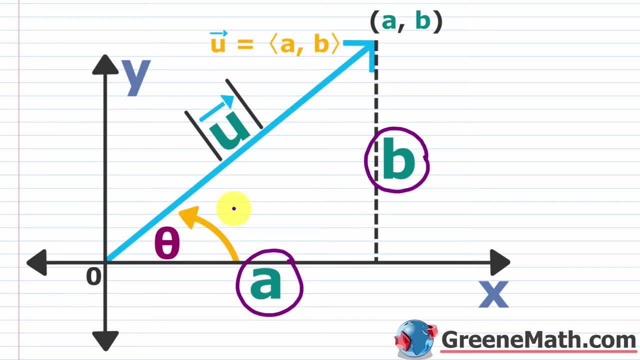 here. i know that the sine of this angle theta is opposite. okay, over the hypotenuse, which in this case would be the magnitude of this vector u. okay, so i can say that the sine of this angle theta is equal to- we'll go ahead and say this b here, which is the vertical component, over the magnitude. 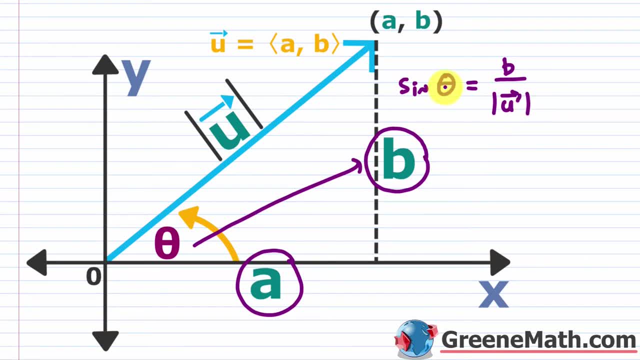 of this vector u. okay, so i'm going to be given the angle theta and i'm going to be given the magnitude of this vector u, so i should be able to plug in there and figure out what b is. okay then, also, if i think about the cosine, so the 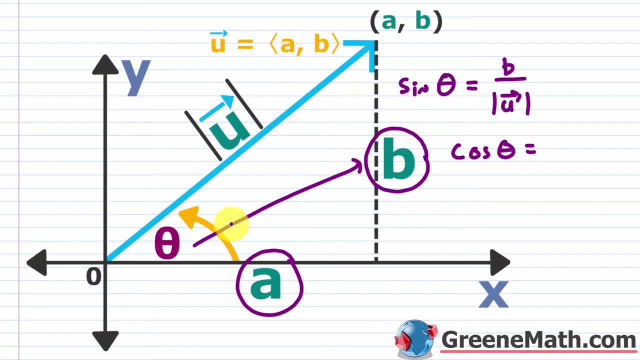 cosine of theta. what is that? well, that's now adjacent. so the agent- let me erase this- that's the adjacent over the hypotenuse. so this would be a over the magnitude of this, u guy. okay, so we can use these two. we'll just basically solve them for a and b, okay, and then we'll plug in and we'll have. 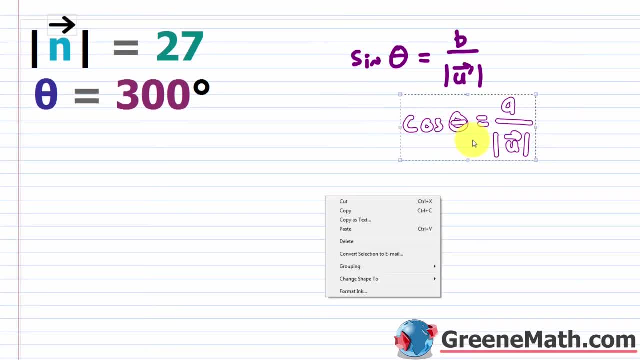 our answers. so let me just paste this in here and let me drag this over a little bit. we can solve this for a and b to come up with a nice little formula to use here. so basically, if i multiply both sides here by the magnitude of this vector u, you're going to see that b is equal to. you would have the magnitude. 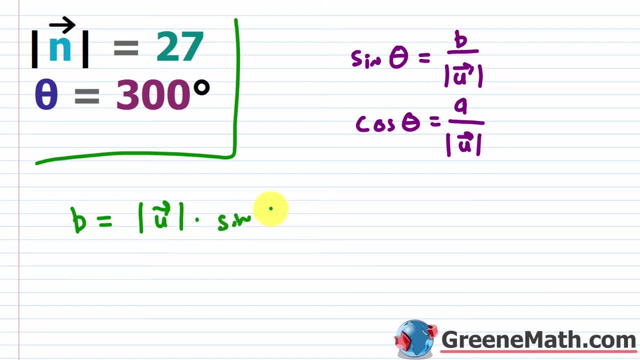 of this vector u and then times the sine of this direction, angle, theta. okay, then here, a is equal to the magnitude of this vector u times the cosine of theta. okay, let's get rid of this. now we have a little formula to use, so i'm given the magnitude of some vector n. okay, so i want to find the. 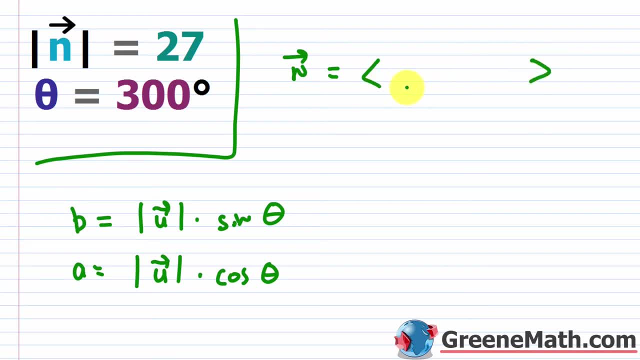 component form and basically all i'm going to do is think about this and this. so i want the a and the b, so the a goes here, the b goes here. okay, that's all we're doing. so the first one: for the a, you're going to think about going down here. the magnitude in this case of our vector n is 27, so i'm going to 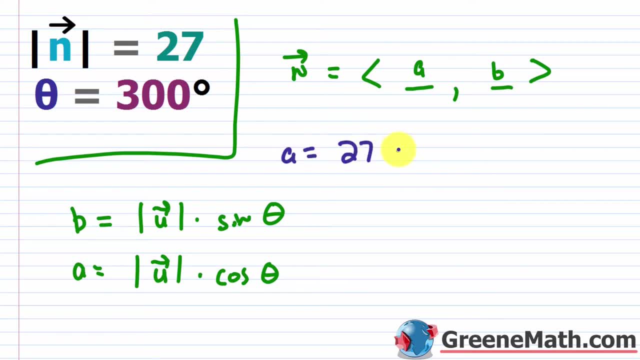 have 27. let's put a equals this, so 27 times the cosine of the direction angle. theta in this case is 300 degrees. now, first off, a 300 degree angle is in quadrant 4. cosine is positive in quadrants 1 and 4. okay, so we know that this guy's going to be positive. 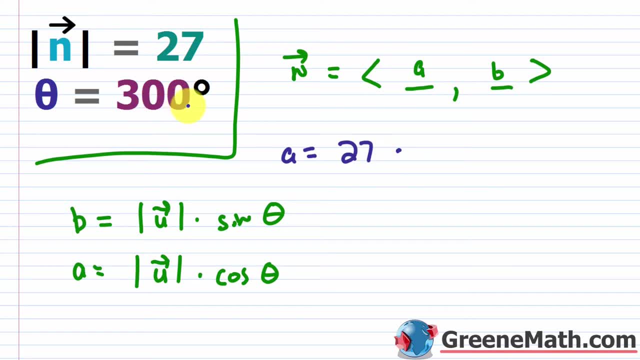 now 300 degrees, has a reference angle of 60 degrees and cosine of 60 degrees is going to be a half, so i can just put times a half here, and this is basically 27 over 2. okay, so 27 over 2, okay, then for b. for b it's equal to what, so in this case again, the magnitude of this vector n is 27. 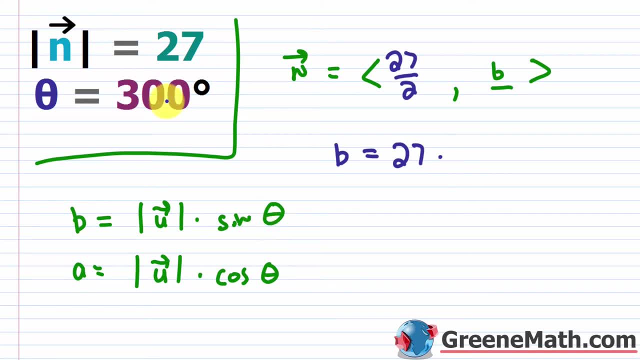 and times the sine of this guy 300 degrees. so again, think about the fact that in quadrant 4 your sine is going to be negative. right sine is positive in quadrants 1 and 2 only, so in quadrant 4 it's going to be negative. okay, so i'm going to put negative and then the reference angle is 60. 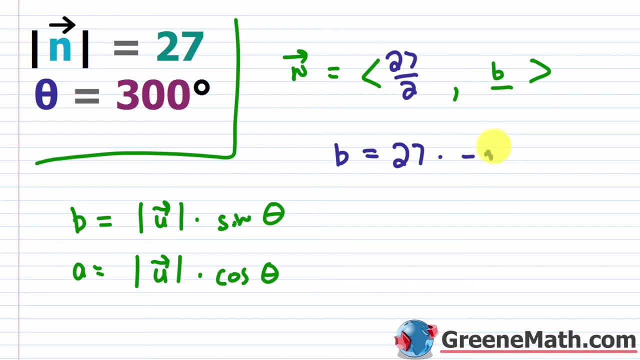 degrees. so sine of 60 degrees is square root of 3, square root of 3 over 2. okay, so all this is- you're not going to be able to really simplify this too much. you're going to say this is negative. let me put this out in front. so the negative of 27 times the square root of 3 over 2. let me close my. 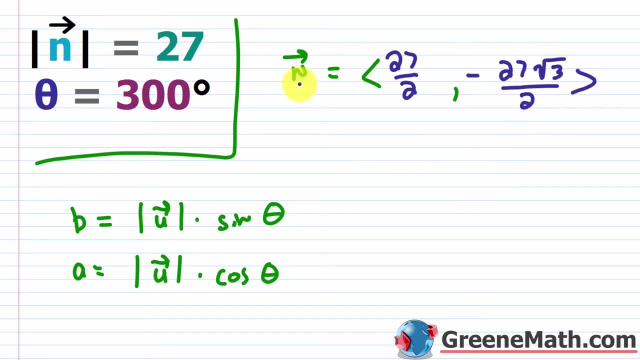 brackets down. so this would be your component of the square root of 3 over 2. so you're going to put this in front of the square root of 3 over 2 and then you're going to put this in front of the square root of 3 over 2. 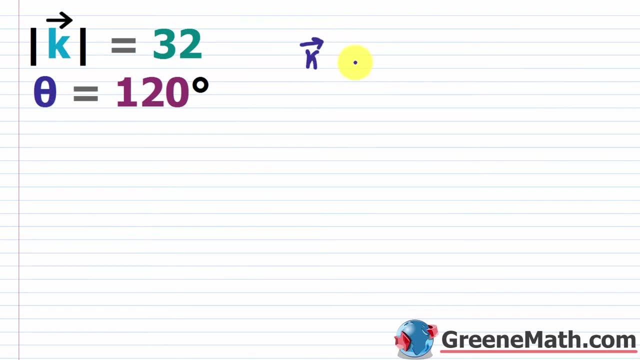 so, again, all i'm going to do here, let's go ahead and write this vector k like this is equal to. i'm going to set up my brackets and again, this is a comma b, so a is equal to, again, with the horizontal. you're thinking about cosine, right? so all it is is this guy right here times the cosine of this. 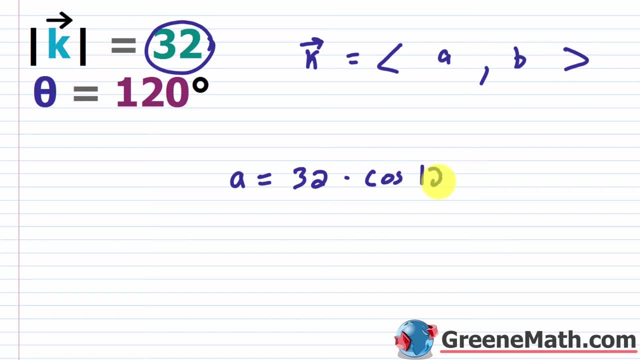 right here, so 32 times the cosine of 120 degrees. now this again has a 60 degree reference angle. but now i'm in quadrant 2 and cosine of this right here, so 32 times the cosine of 120 degrees, is negative in quadrant 2. so this is going to be negative half, right? so negative one half. 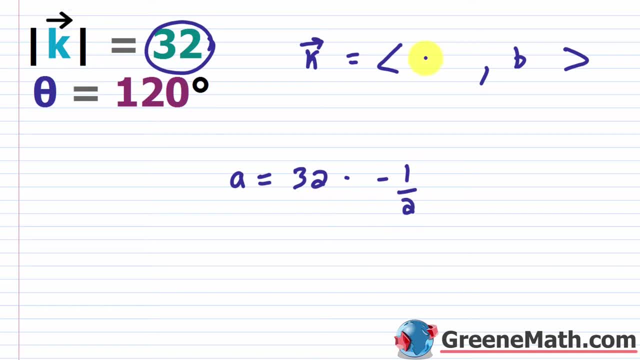 so this ended up being negative 16, right? so if we put this in here as negative 16- because this will cancel with this and give you 16, okay, and obviously this is times negative one, so that's where the negative comes from. okay, let's get rid of this. let's think about b now. so b is equal to. 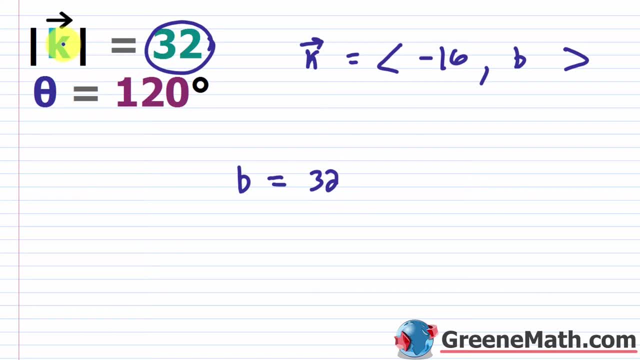 you're going to take the same 32, the magnitude of this vector, k times now the sine. okay, the sine of this: 120 degrees. while i'm in quadrant 2, okay, i have that same 60 degree reference angle, but now sine is positive. okay, so this is going to be times. 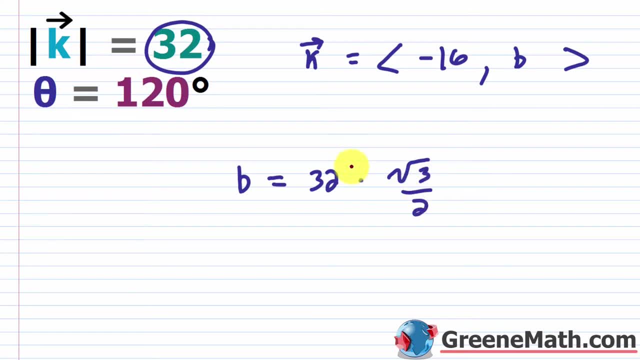 square root of 3 over 2, and so this is going to cancel with this and give me 16. so this is 16 times the square root of 3. okay, so 16 times the square root of 3. so that's going to be our component. 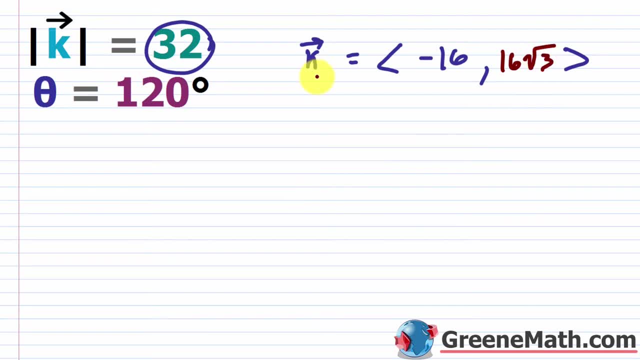 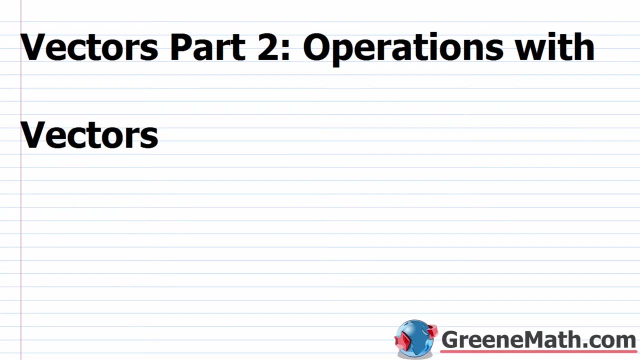 form and maybe i should make that 3 a little bit better. okay, for this vector k again, your horizontal component is negative 16. your vertical component is 16 times the square root of 3. in this lesson we want to continue to talk about the square root of 3 and we're going to talk about the. 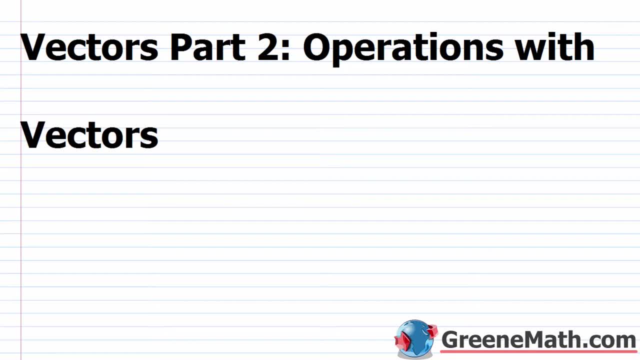 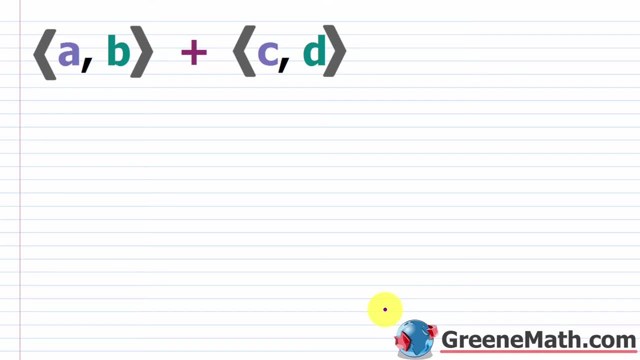 vectors, and here specifically, we're going to focus on operations with vectors. all right, so let's start out here by talking about how to add two vectors together. so the sum of two or more vectors is also a vector. this is referred to as the resultant vector, or some people will just call. 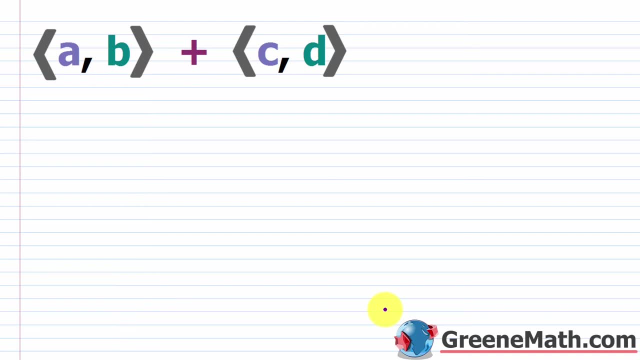 this the resultant. okay, so basically, let's say i had this simple example here, very generic, and on the left i have this vector with a horizontal component of a and a vertical component of b, and i want to add this vector to the horizontal component of a and i want to add: 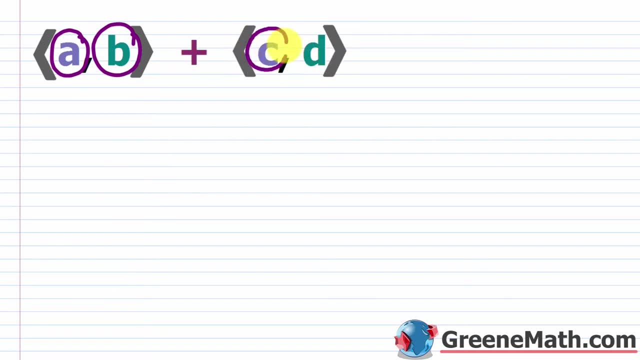 this to this vector on the right where there's a horizontal component of c and a vertical component of d. so for my resultant vector, or just the resultant, if you want to say that basically i'm going to do a plus c, so a plus c, okay, then i'll do a comma and then i'm going to do b plus d, so b. 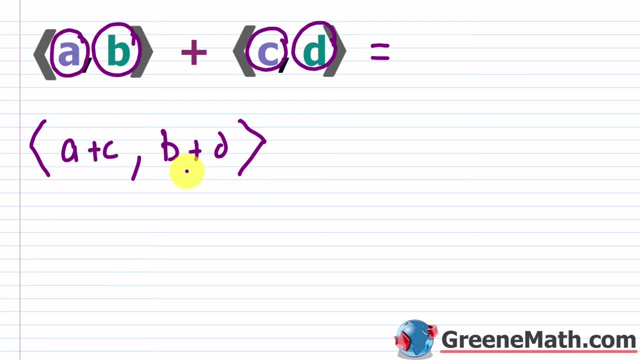 plus d. okay, that's all it is. it's very, very simple. you're going to sum these horizontal components so a plus c. that's going to give me the horizontal component for my resultant vector. then i'm going to sum these vertical components so b plus d. that's going to give me my vertical component for my. 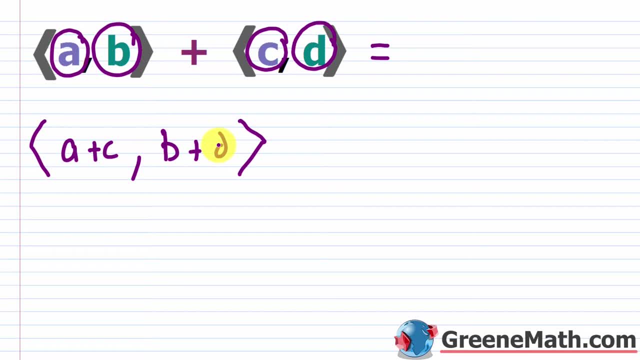 resultant vector, and you can do this with more than two. let's say, for example, i had something like two and then three here, okay, and then let's say: plus, we'll do maybe four and then five here, and let's say we do plus, let's say we do six, and then you can even do like negative, so negative. 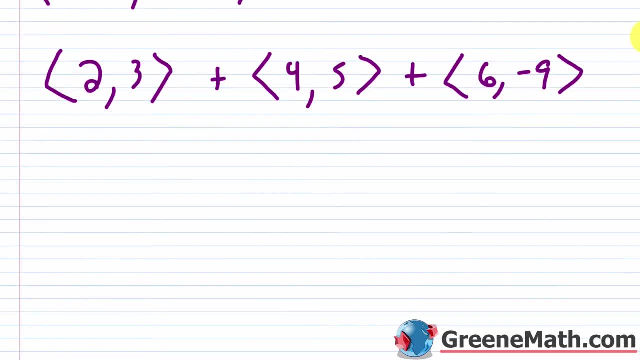 nine. okay, so something like this. so all we would do if we wanted to find the sum here, you would say: plus four plus six. so two plus four is six, six plus six is twelve. okay, so that's the horizontal component for this resultant vector, and then for the vertical component, you're going to do three. 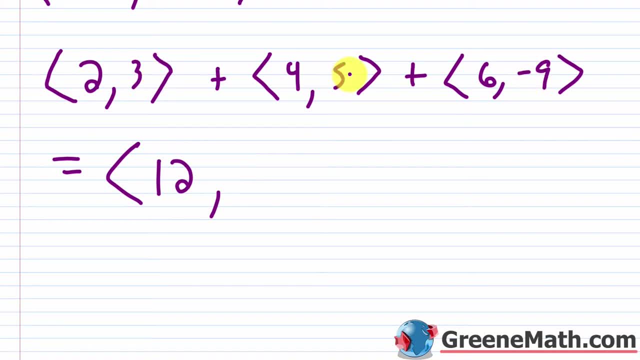 plus five plus negative nine. so three plus five is eight. eight plus negative nine is going to be negative one. okay, so this resultant vector, the horizontal component, is 12 and the vertical component is negative one. all right, let's also talk about how to show this geometrically. we can. 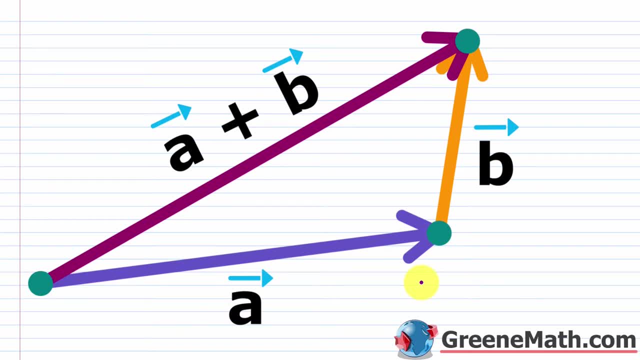 do this with a triangle, and we can also do it with a parallelogram. so, using the triangle method, let's think about this: we have this vector a and this vector b. they're being added together. so let's say, i started by just sketching vector a, so this is the initial. 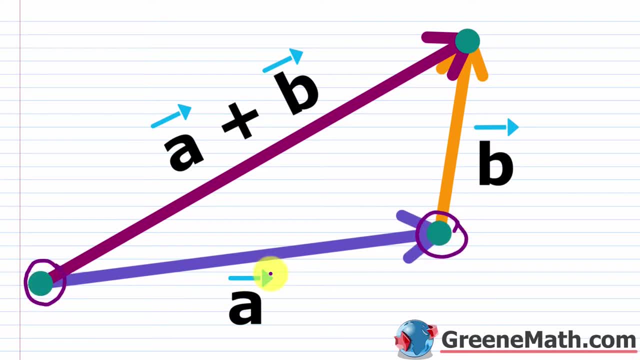 point, and this is the terminal point. so i've just sketched vector a. then for vector b i'm going to use my horizontal and vertical components to sketch this guy again. the initial points here. your terminal point would be here, let's say okay, and then your resultant vector, or basically the 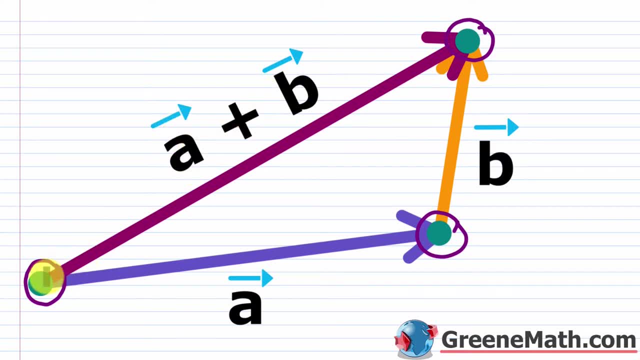 vector a plus the vector b is going to be this guy right here, so this vector right here. so you'll notice that the initial point for this vector is going to be the same as the initial point from the vector a. then the terminal point from this vector is going to be the same as the terminal point from this vector b. okay, so? 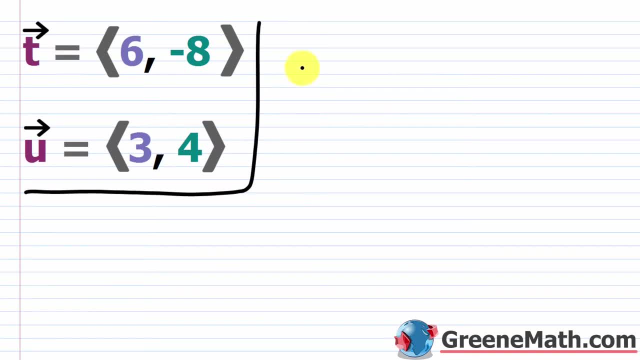 that's all you're doing. so for this example, let's go ahead and say we have the vector t, okay, we're going to add to this our vector u, our vector u. so what is this going to give us? so, for the vector t, we're going to add a horizontal component, which is going to be this 6, and a vertical component of. 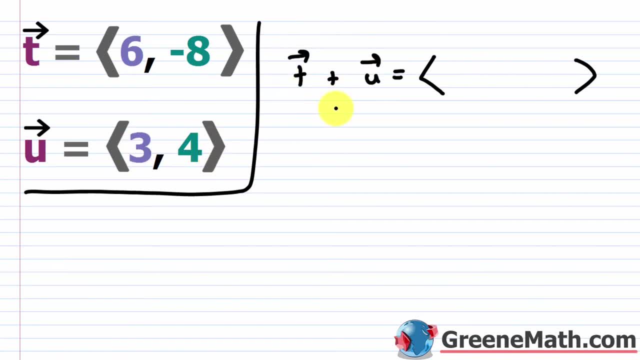 negative 8.. for the vector u, you have a horizontal component of 3 and vertical component of 4.. so in this resultant vector here to get the horizontal component, i'm going to take this 6 and add it to this 3, right? so just sum the horizontal components. so 6 plus 3 is 9. okay for the vertical component. 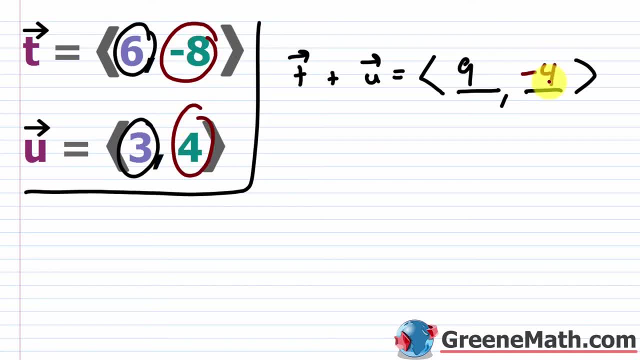 i'm basically going to sum the vertical components here. so negative 8 plus 4 is going to be negative 4, okay, so this guy basically would have an initial point at the origin- okay, here's the resultant one- and we have a terminal point at 9, negative 4.. 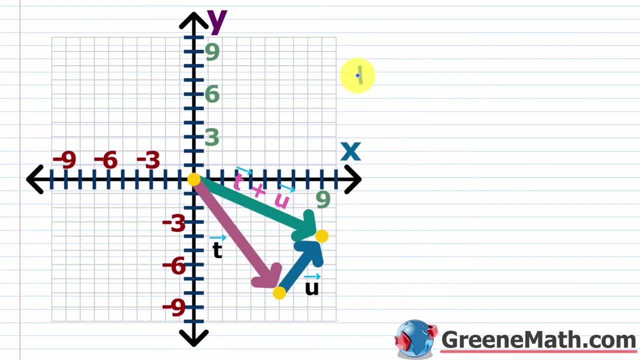 So let's look at this graphically. Let's start out by just redefining things. So we have this vector t. okay, In component form this was 6, negative 8.. So we had a horizontal component of 6, a vertical component of negative 8.. 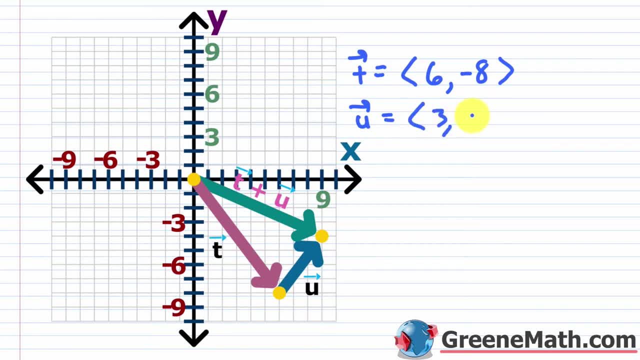 Then for the vector u, we had a horizontal component of 3, and a vertical component of 4.. Then for this resultant vector, so the vector t plus the vector u, we basically what We said, 6 plus 3 was 9.. 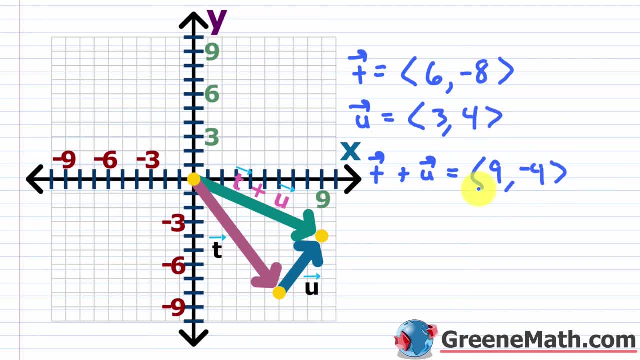 We said negative 8 plus 4 is negative 4, right, So a horizontal component of 9 and a vertical component of negative 4.. Okay, so, looking at the graph, here you see, for vector t, we started with an initial point here, at the origin right. 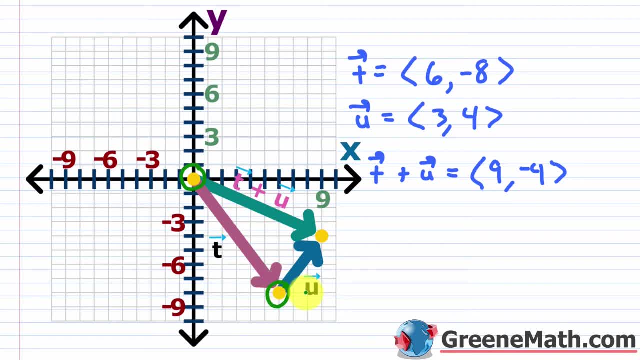 It's just in standard position, So the terminal point is going to be right here, which is at 6, negative 8,. okay, So we want 6 units to the right and we want 8 units down. So that's as expected. 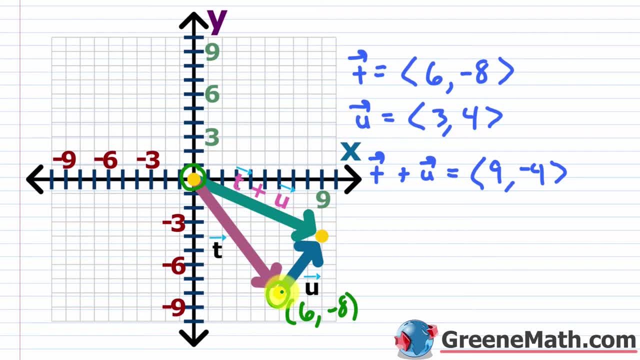 This vector u. when you try to sketch that now, the initial point has to be at 6, negative 8.. So you're using the 3 as the horizontal movement, right. So I'm just going 3 units to the right. 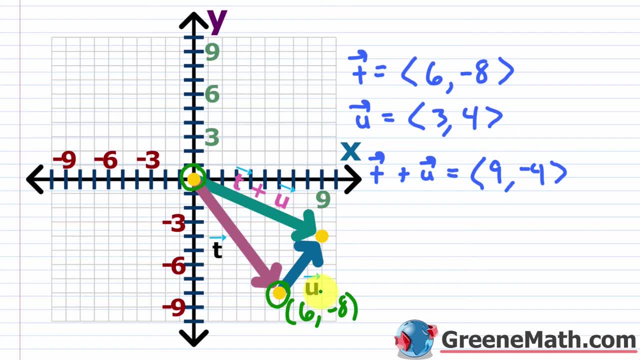 and then I'm using the 4 as a vertical movement. So now I'm going 4 units up, So 1,, 2, 3 units to the right- that puts me at 9 on the x-axis, and then 4 units up- 1,, 2,, 3,, 4, that puts me at negative 4 on the y-axis. 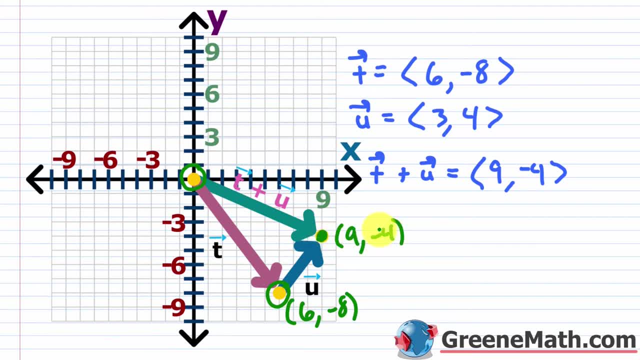 So this point right here would be 9, negative 4,. okay, And this is consistent with what we said, right? So basically, this vector right here, this resultant vector, has the same initial point, okay, as this vector t. 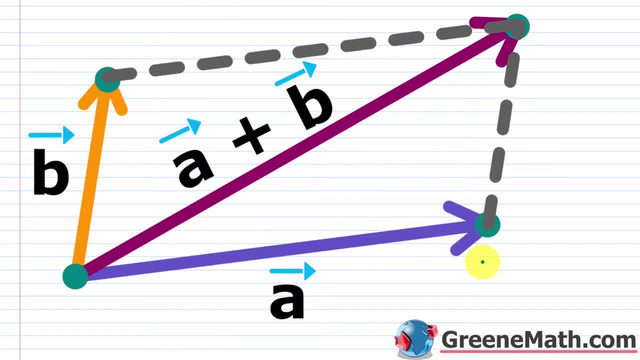 and has the same terminal point as this vector u. All right, now let's think a little bit about this parallelogram method. This one's a little bit harder to draw, especially if you're not working on a coordinate plane, But essentially what you want to do here. 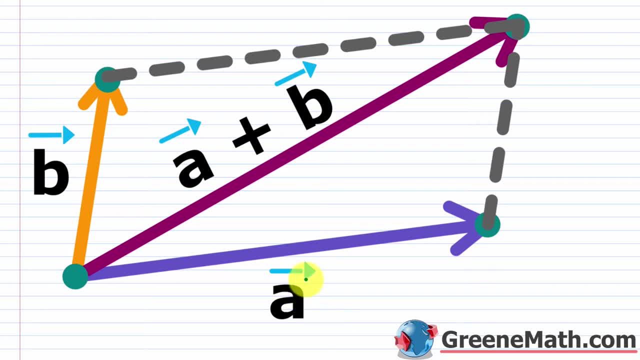 is, have the initial point for the vector a and for the vector b to be the same, okay, So everything's going to have the same initial point. Then you'd have your normal terminal point, your normal terminal point. So these are easy to draw, especially if we're on the coordinate plane. 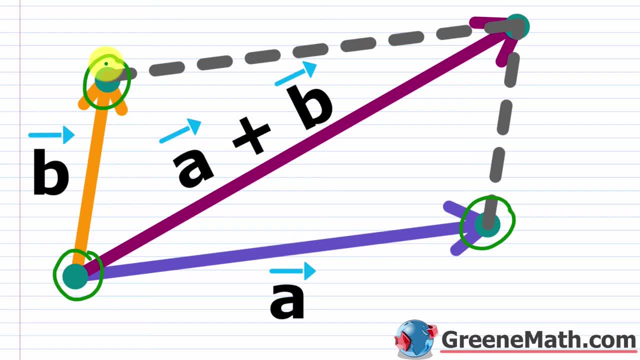 The next part is a little bit more challenging. You're going to complete a parallelogram. Essentially, what you're going to do is you're going to take this side right here and just slide it down. okay, So you would have it like that, okay. 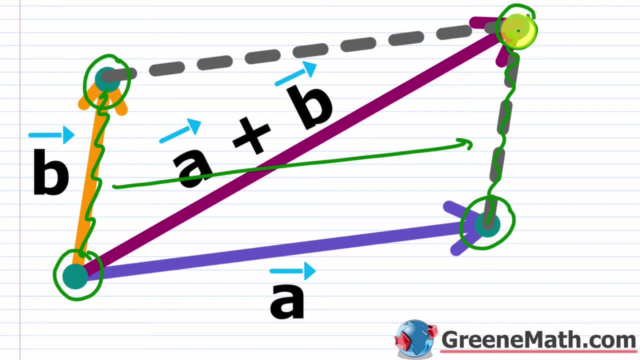 And then, basically, this point right here is going to help you set up this diagonal, So this is going to be your resultant vector. okay, Now you could also do it this way, okay, Where you take this side right here and basically copy it and slide it down. 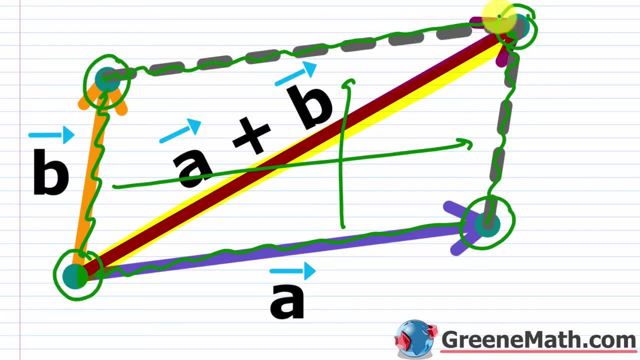 And if you want to form the full parallelogram, you need to do that right. So, basically, with the parallelogram. okay, in case you're unfamiliar with this, you're going to have opposite sides that are going to be equal in length. 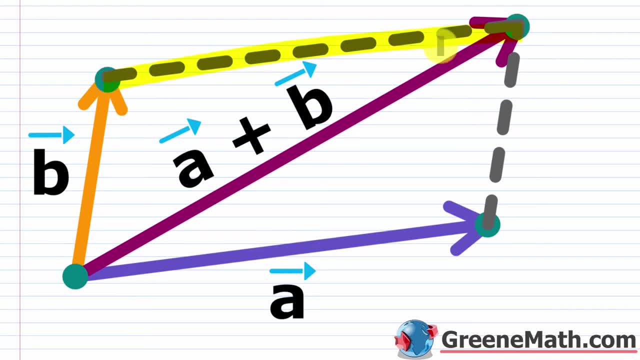 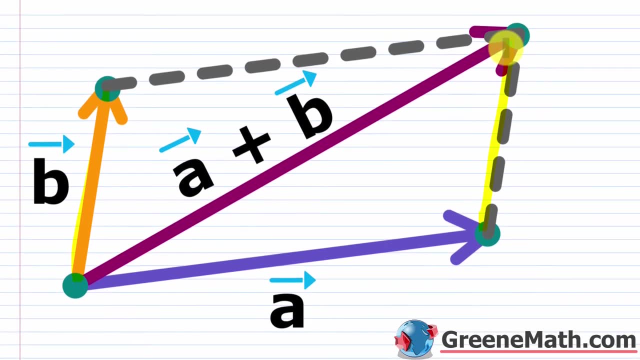 and they're also going to be parallel, right. So this side and this side right here are the same length and they're parallel. and then this side and this side are the same length and they're also parallel. Now let's take a look at this with an example. 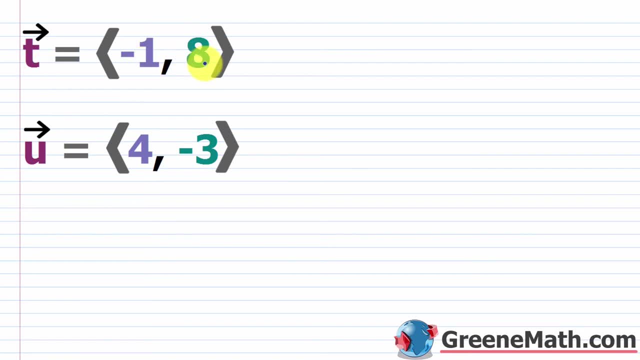 We have this vector t, which is a horizontal component of negative 1, and a vertical component of 8.. We have this vector u, which is a horizontal component of 4, and a vertical component of negative 3.. So, if I did, the vector t plus the vector u, 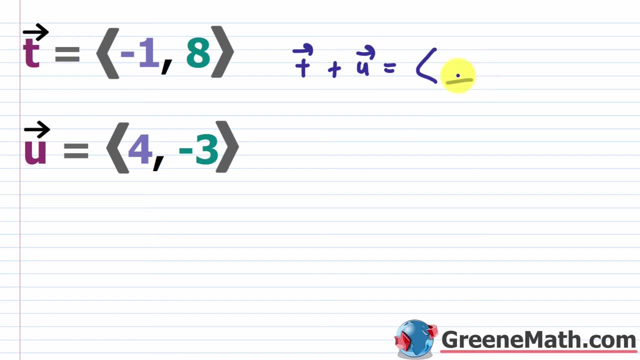 again. all I need to do is for this guy right here. for the horizontal component, I'm going to do negative 1 plus 4.. That's just going to give me 3, okay. For the vertical component, I'm going to do 8 plus negative 3,. 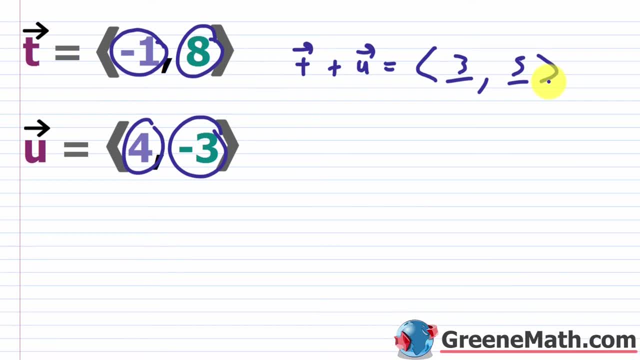 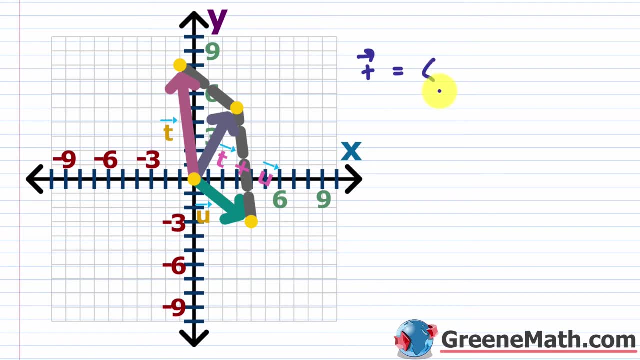 which is going to give me 5, okay, So all I want to do is sketch this. Alright, so let's write this out again. So the vector t is going to be with a horizontal component of negative 1 and a vertical component of 8.. 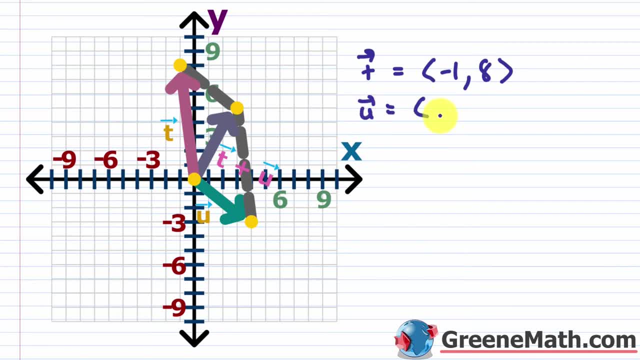 Then the vector u is going to have a horizontal component of 4 and a vertical component of negative 3.. So the resultant vector, when you do this vector t plus this vector u, this is going to be negative 1 plus 4, which is 3,. 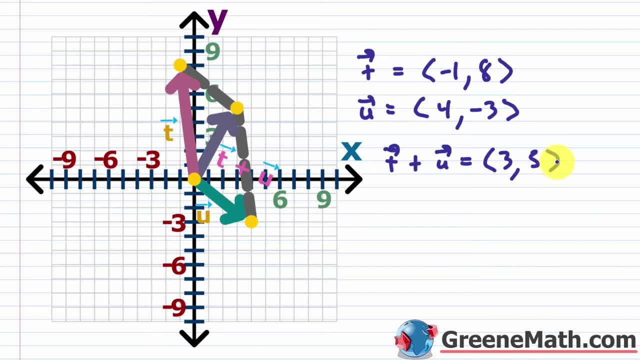 and then 8 plus negative 3, which is 5, okay, So you can see this graphically. It's a little bit more busy than the triangle drawing, but it's still there. So if you look at the first guy, so the vector t. 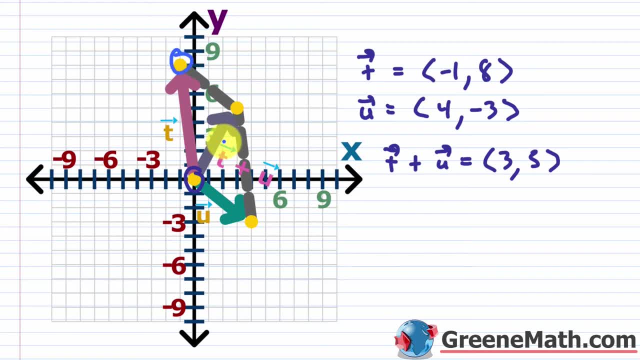 here's the initial point at the origin, and then the terminal point right here is going to be at negative 1 comma 8.. So this is negative 1 comma 8.. Then if you look at your vector u, okay, your initial point is also at the origin. 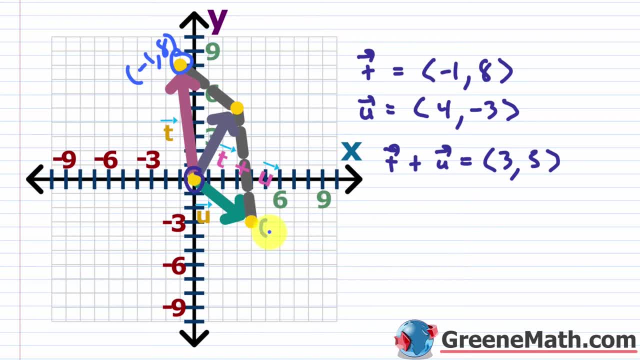 The terminal point here, okay, would be at this point, 4 comma, negative 3, okay, So 4 units to the right, 3 units down, And then basically, if you wanted to draw this, you already know the terminal point. 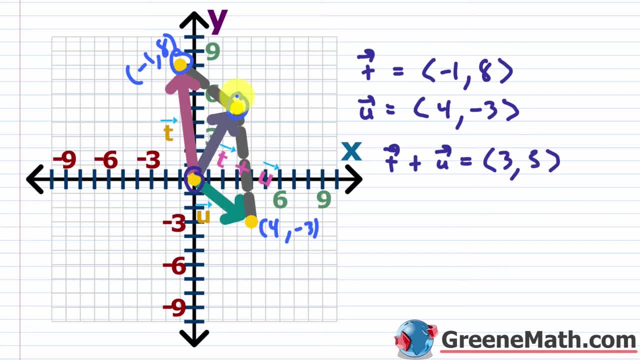 of this resultant vector is here, okay, which is at 3 comma 5.. And you could basically sketch: this guy right here, okay, and this guy right here, Those sides there again, this side right here, okay, is going to be the same length and parallel. 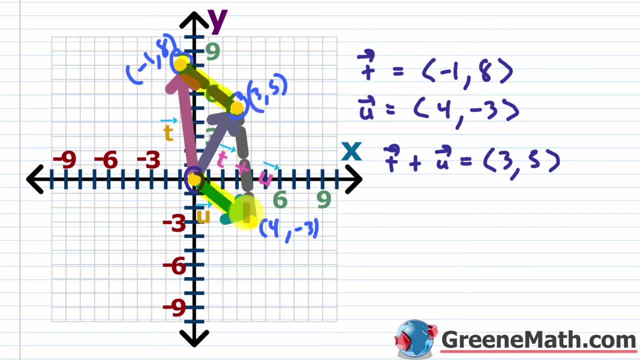 to this side right here, Then the other one's the same thing. So this side right here and this side right here, same length, and then are also parallel, okay, So when you look at this guy, you would then draw this vector here, okay. 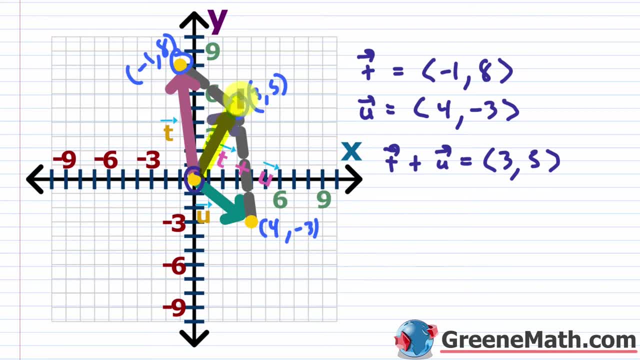 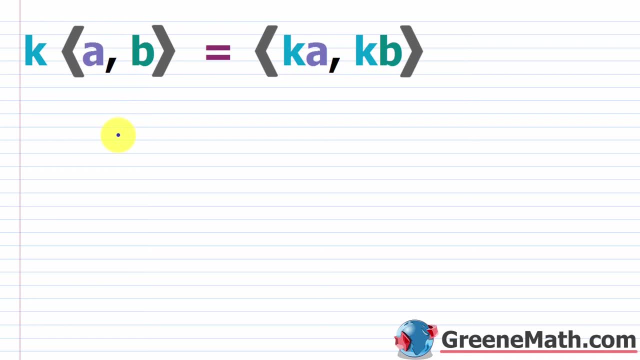 where, basically, the initial point is the same as the other two vectors and your terminal point is right there. okay, So it's then going to be at that, 3 comma 5.. Okay, let's talk about this: multiplying a vector by a scalar. 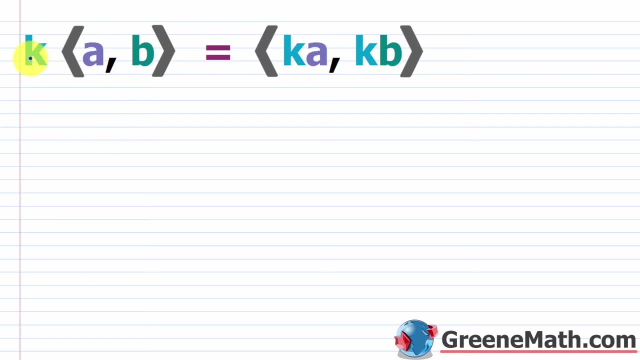 also very easy. So let's say you had some real number, k multiplied by this vector, with a horizontal component of a and a vertical component of b. Well, the result of this is going to be a vector with a horizontal component of k times a. 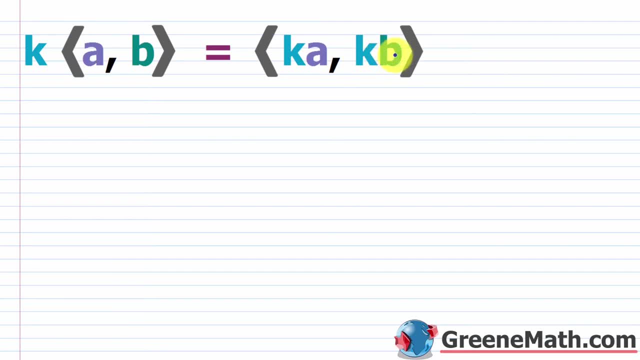 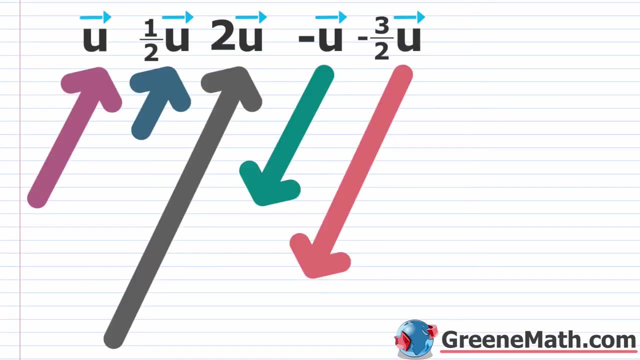 and a vertical component of k times b. okay, So the reason they call it a scalar is: you can think about this as scaling your vector. okay, So graphically you can think about it like this: Let's say, we had some vector u- okay, 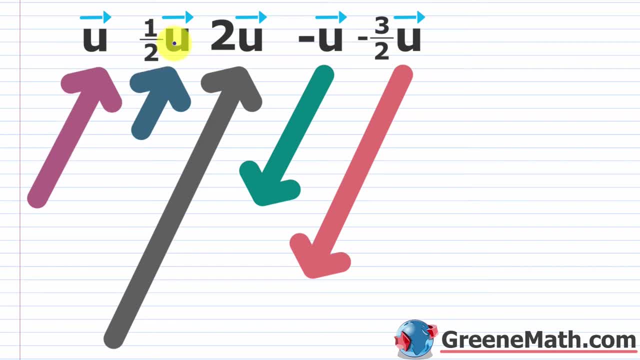 So this is u to start. If you add half times this vector u, we can see that it's half as long, okay. If you add 2 times this vector u now, it's twice as long, okay, compared to this original vector u. 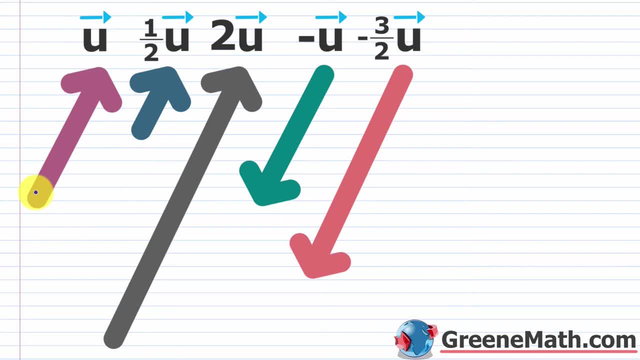 Now, when you get a negative involved, what it's going to do is it's going to give you an opposite direction, okay, So basically, if I had the negative of this vector u, it's going to flip the direction right. So it's the same length. 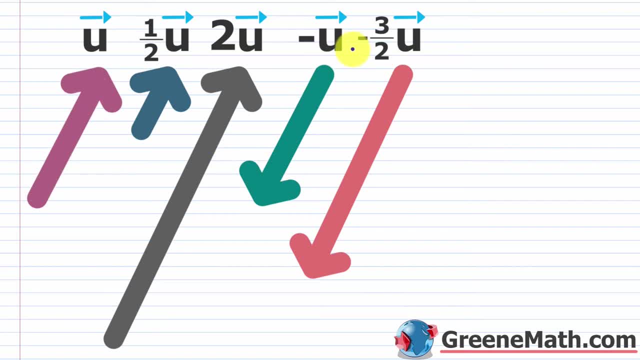 but the direction is flipped right, It's the opposite direction. Then if I had negative 3 halves times this vector u, well, now it's the opposite direction and basically, compared to this original vector u in terms of its length, it's going to have one half. 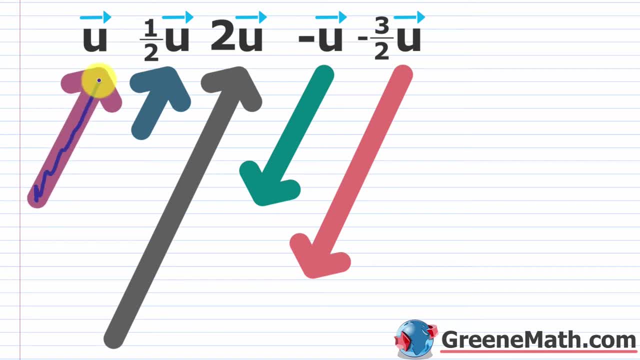 of the vector u added on right. So it's like I took this vector right here and added this vector right here onto it and then I gave it the opposite direction to form this vector here which is negative, 3 halves times the vector u. 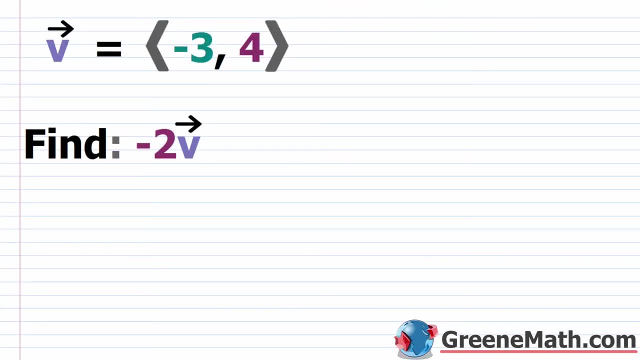 Okay, Let's find the negative 2 times the vector v and then I'll show you this graphically. So we have the vector v. horizontal component is negative 3,, vertical component is 4.. So if I wanted negative 2 times this vector v, 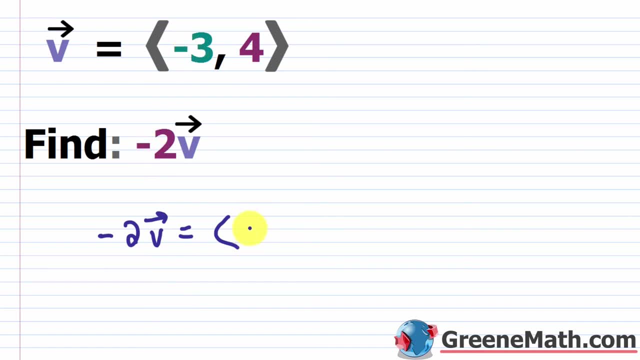 then all I would do is negative 3 times, negative 2,, which is positive 6,. and then I would do negative 2 times 4,, which is negative 8,. okay, So this guy right here, this negative 2 times this vector v. 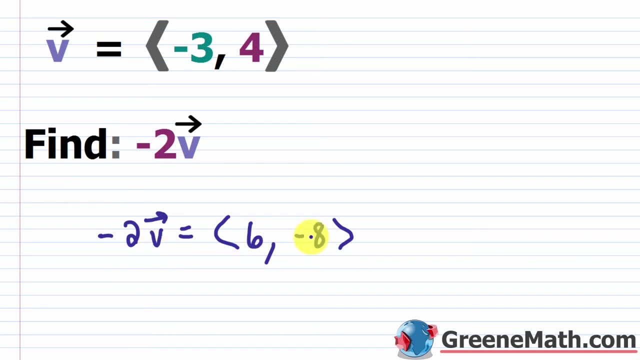 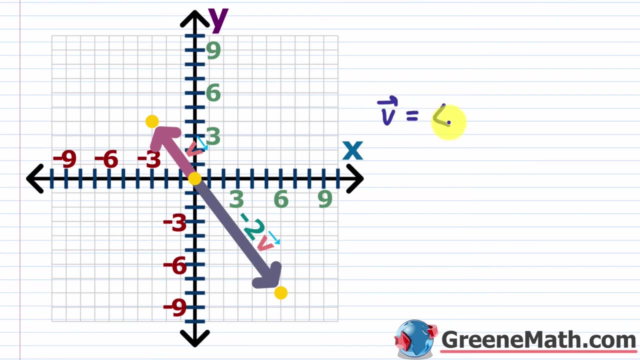 is going to be 6 for the horizontal component and negative 8 for the vertical component. Now, graphically, the original vector v- again, when we look at this- is going to have a horizontal component of negative 3 and a vertical component of 4, okay. 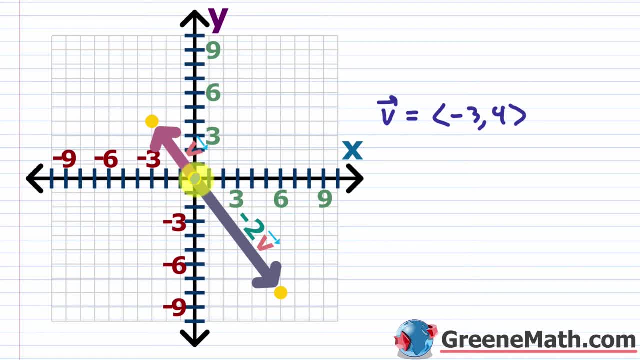 So you see, it starts at the origin. that's the initial point, and then the terminal point is right here again at negative 3 comma 4, okay, So 3 units to the left, 4 units up Now if I look at negative 2 multiplied by that vector v, 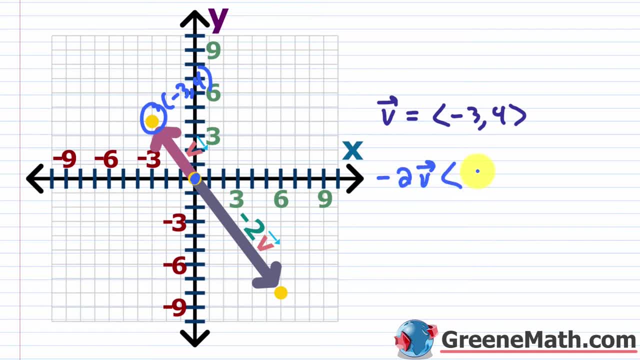 so negative 2 multiplied by this vector v- again, I'm scaling this because this guy is twice as long. okay, That's the 2 part. and then it's going in the opposite direction. that's the negative part. okay, So basically I'm multiplying everything here by negative 2,. 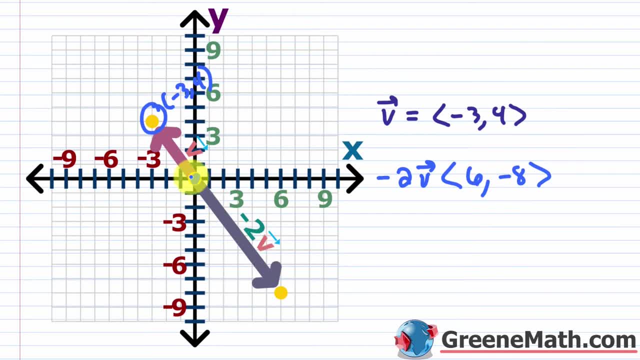 so this is 6, and this is negative 8, and you'll see that the initial point is the same. the terminal point is here. I went 6 units to the right, 8 units down. this is 6 comma negative 8, okay. 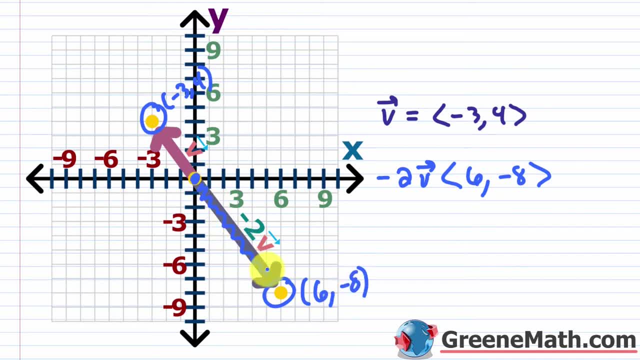 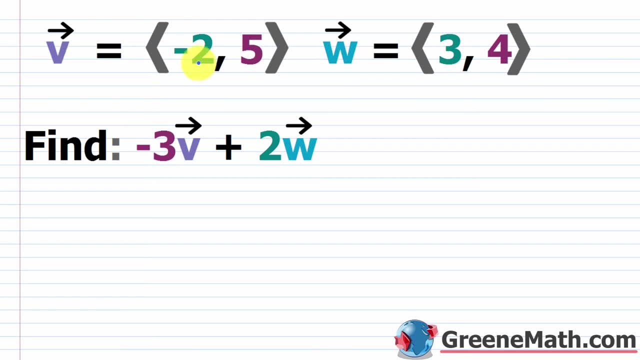 So you can see, this guy right here is twice as long and it's also going in the opposite direction. Okay, so let's combine these two concepts together. So now we have this: vector v, horizontal component of negative 2, vertical component of 5,. 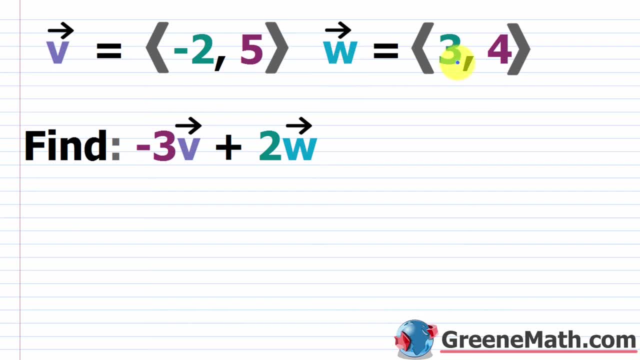 and then we have this vector w with a horizontal component of 3, and a vertical component of 4.. We want to find negative 3 times the vector v plus 2 times the vector w. okay, So all I'm going to do is set this up. 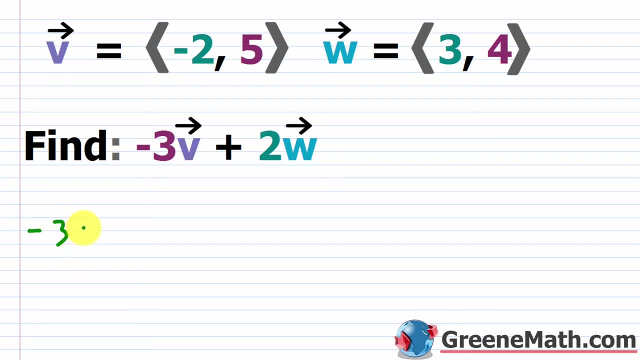 and say negative 3 times this vector v plus 2 times this vector v is equal to- I'm just going to put a negative 3, out in front of this, so negative 2, and then 5 is inside. 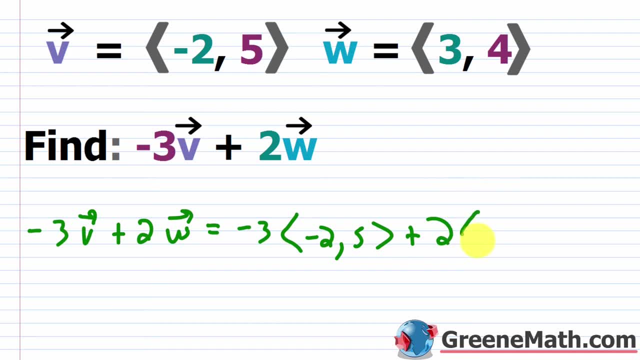 and then, plus, I'm just going to put a 2, out in front, and then I'm going to put a 3, and then a 4 inside. Okay, so that's all I'm doing, So what I'm going to do. 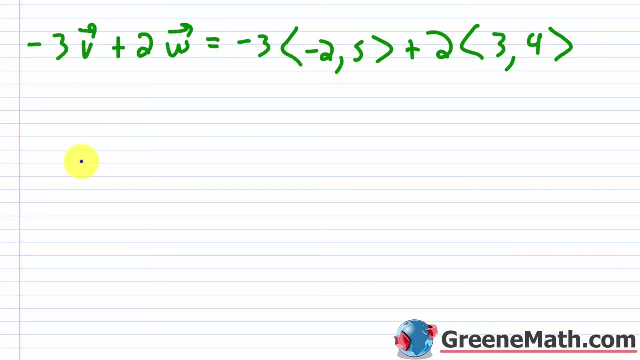 is just first multiply. so let me copy this down, or I could just put equals. to keep this going, I'll say basically: each part of this is going to get multiplied by negative 3, so this would be negative 3 times negative 2,, which is 6,. 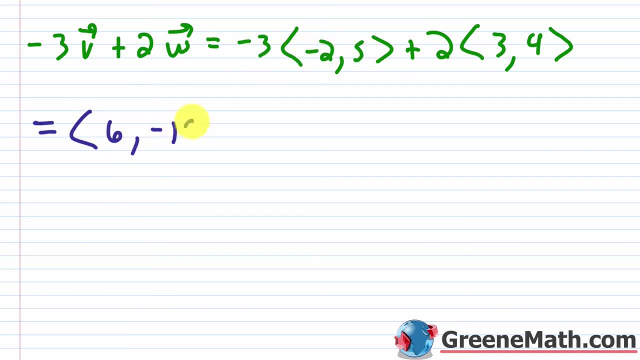 and then negative 3 times negative 2,, which is 5,, would be negative 15.. Okay, Then, plus 2 times 3 is 6, and then 2 times 4 is going to be 8.. Okay. 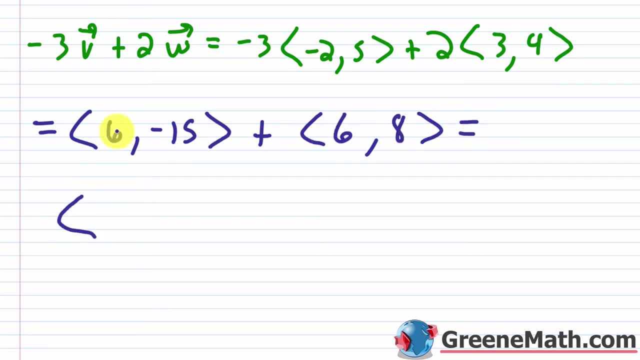 So now I just want to find the sum again, very, very easy. I'm going to add the horizontal components, so 6 plus 6 is 12, then I'm going to add the vertical components, so negative 15 plus 8 is negative 7.. 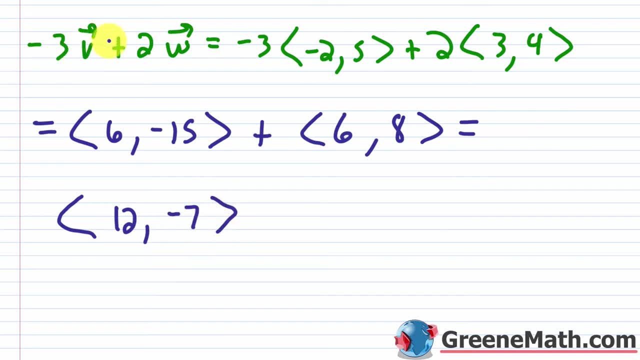 Okay. So in the end, this negative 3 times this vector v plus this 2, times this vector w gives me this vector okay with a horizontal component of 12, and a vertical component of negative 7.. 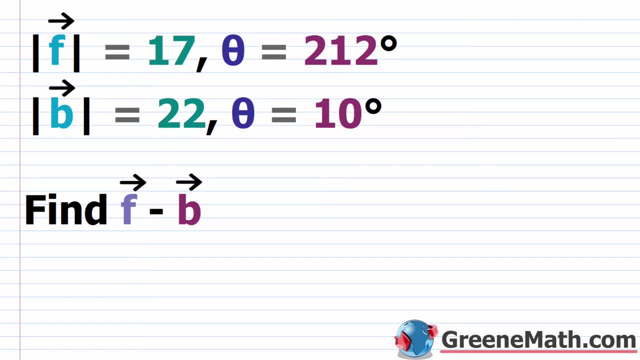 All right, let's wrap up the lesson and look at something that involves a concept from the last lesson. So we have: the magnitude of this vector f is 17,. the direction angle, theta, is 212 degrees. the magnitude of this vector b is 22,. 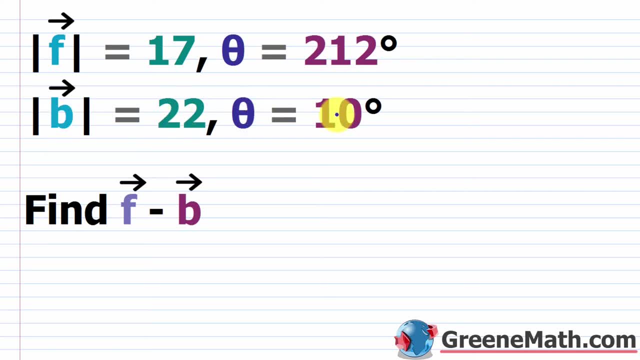 and the direction angle, theta is 10 degrees. So what if I wanted to find the vector f minus the vector b? What would I do? Well, first I need to find the horizontal and vertical components for each. So remember how to do this. 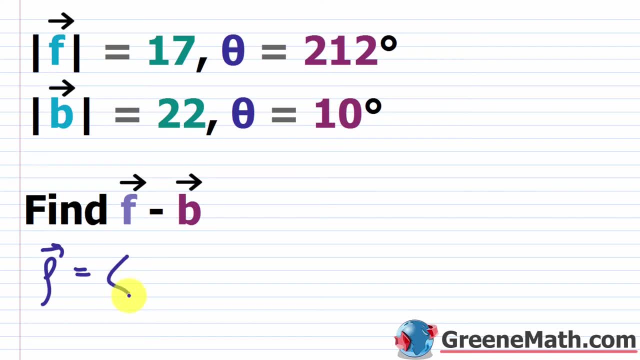 For the vector f to set this up, I would do what I would take my magnitude 17,. and for the horizontal component, I'm multiplying by the cosine of this direction angle, which is 212 degrees. And then for the other one, 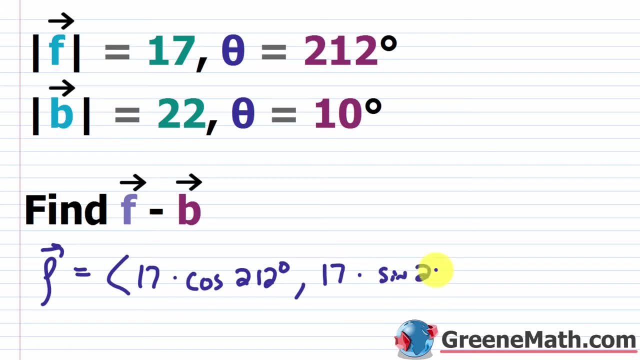 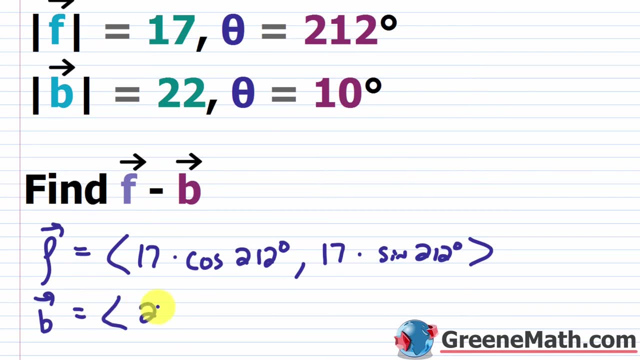 it's going to be 17 times the sine of 212 degrees. Okay, That's all I'm doing, Then, for b, this vector b, what I would do is I would do 22. now the magnitude of this guy. 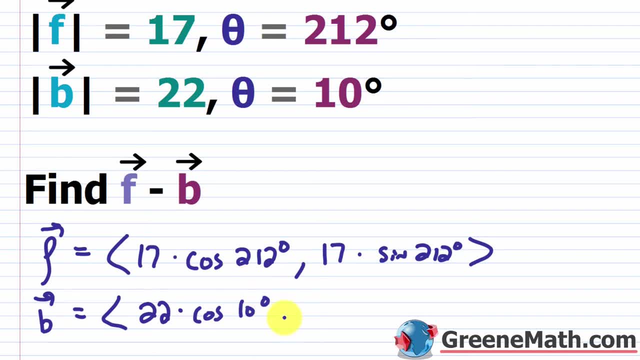 times the cosine of, in this case, 10 degrees. Okay. And then I would do 22 times the sine of this 10 degrees as well, Okay. So you can punch that up and get approximations and then set up your subtraction. 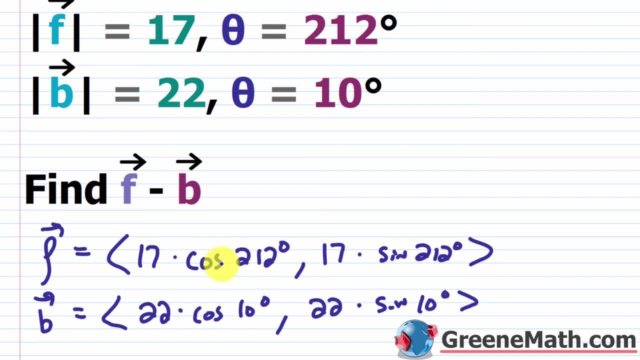 Or, if you want to, you can go ahead and do this all in one step. So we could basically say 17 times the cosine of 212 degrees minus 22 times the cosine of 10 degrees. Okay, Then, comma, you would have 17 times the sine of 212 degrees. 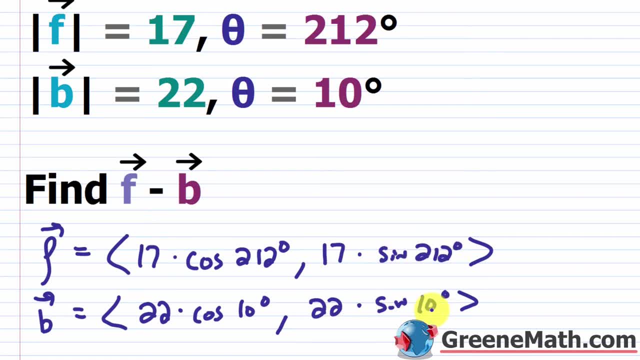 minus 22 times the sine of 10 degrees. Up to you. How do you want to do it? You get the same answer either way. Actually, the rounding might be a little bit different, but let's just go ahead and do it the long way. 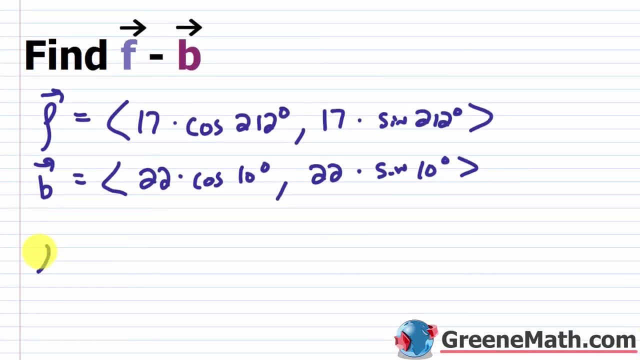 Let's get some practice. So first I'm just going to say the vector f is going to be- let me put approximately here, because I'm going to approximate this- 17 times the cosine of 212 degrees. I'll say that's about negative. 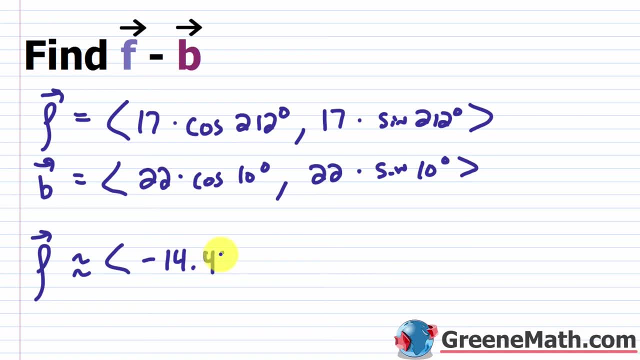 14, point, let's just go ahead and say 42. Okay, This guy, 17 times sine of 212 degrees, is going to be about negative. This is going to be about negative 9.01.. Okay, So this is my vector f. 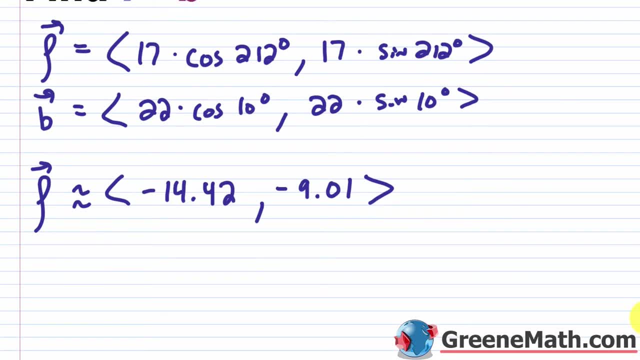 And again, this is an approximation, So let's scroll down and get a little bit more room so we can stay on the screen. I'll do my vector b now. So this is approximately. we'll go ahead and set this up and say 22 times cosine of 10 degrees. 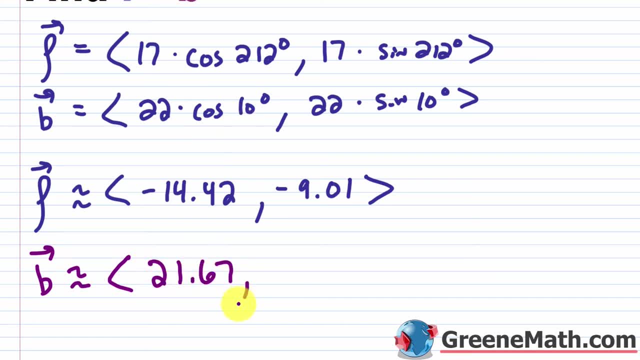 It's going to be about 21.67.. So 21.67.. And then 22 times the sine of 10 degrees, It's going to be about 3.82.. Okay, So now let me make this a little bit better. 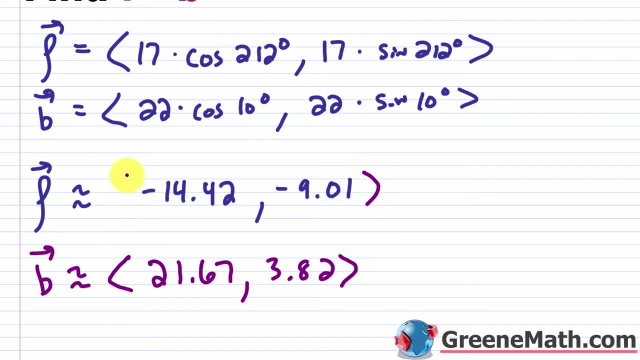 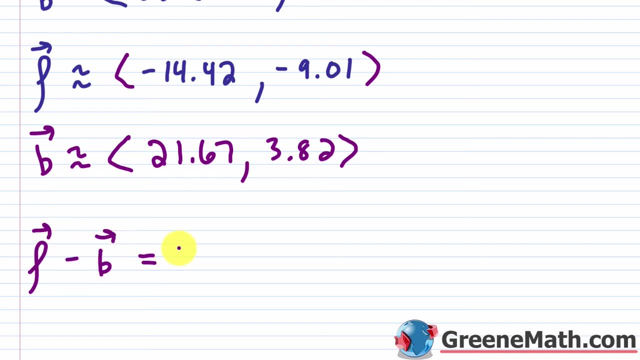 And let me change these. I'll make them a little bit better. A little bit better. Okay, So now, if I come down here, if I want to do the vector f minus the vector b, all this is going to be is negative 14,. 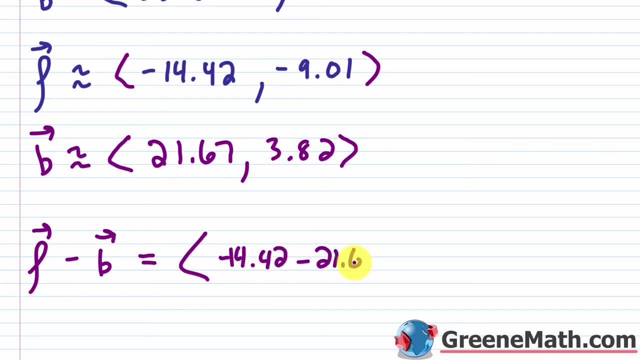 negative 14.42 minus 21.67, comma, I'm going to have negative 9.01 minus 3.82.. Okay, And I put equals. It should probably be approximately to be more precise, So let me go ahead and put that like that. 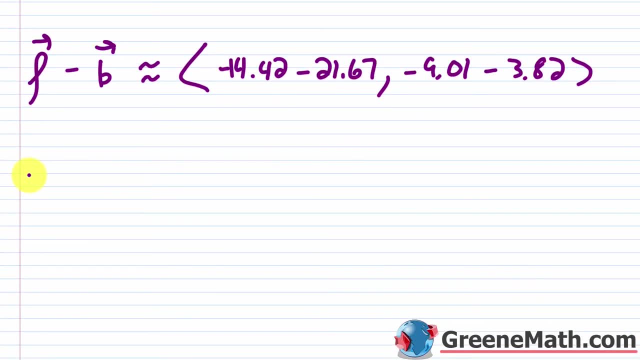 Okay, Let me make that better And let's just go ahead and crank this out. So I'll say this is approximately- and I'll put my little symbol there- say about negative 36.09, right for negative 14.42. 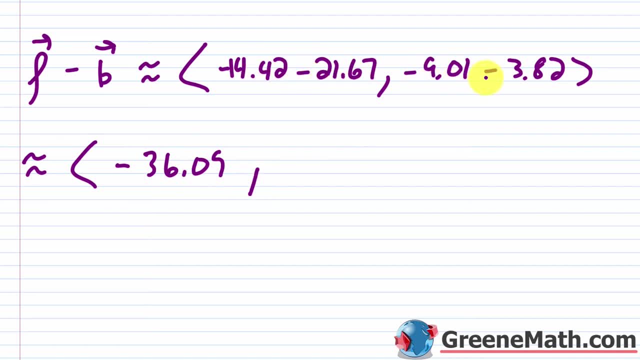 minus 21.67.. Then over here, negative 9.01 minus 3.82.. We'll say this is negative 12.83.. Again, this is an approximation. Okay, So the vector f minus the vector b, the horizontal component would be about. 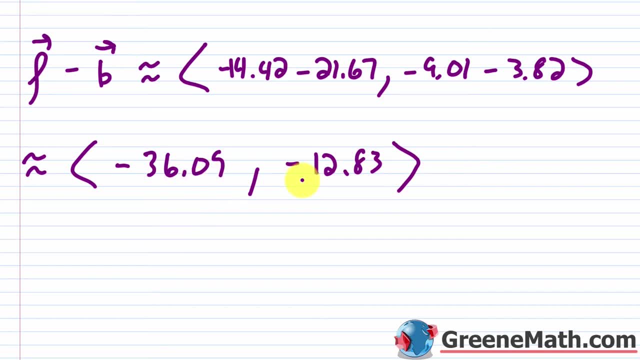 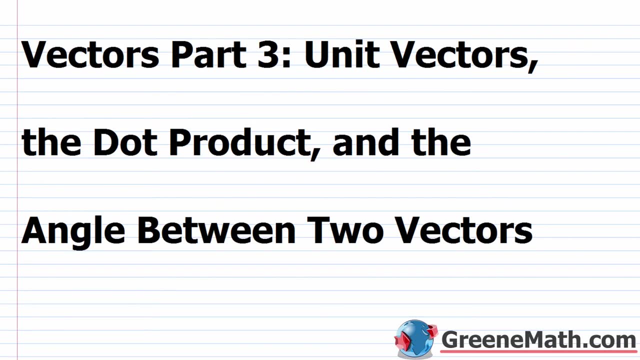 negative 36.09, and the vertical component would be about negative 12.83.. In this lesson we want to continue to talk about vectors, And here, specifically, we're going to focus on unit vectors, the dot product and then the angle between two vectors. 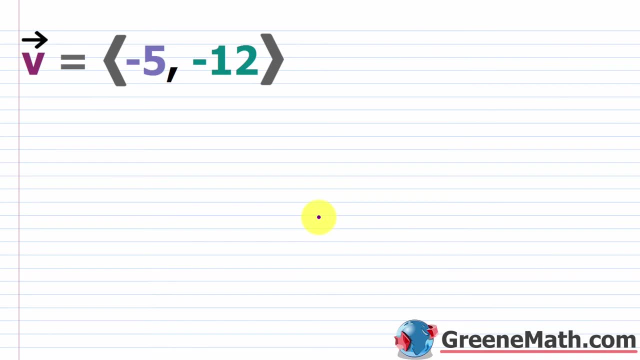 All right. So to start with the lesson, we're going to talk about something called a unit vector. So a unit vector is just a vector that has a magnitude of one. Okay, So let's say that we denote our unit vector with a U. 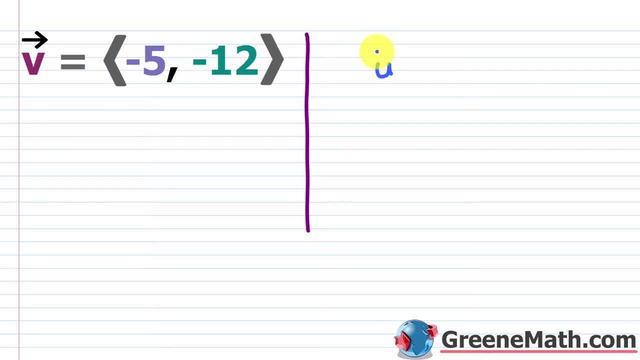 Okay, When you work with a unit vector, you're going to have a special notation. Some people call this a cap, Some people call it a hat, But basically this tells you you have a unit vector. Okay, And if you have a unit vector, 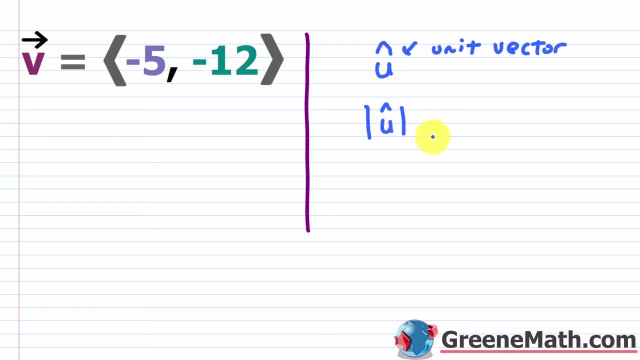 the magnitude of this unit vector- again, let's call it U- is always going to be equal to one. So for some problems you're going to be asked to find a unit vector- let's call it U- that has the same direction. 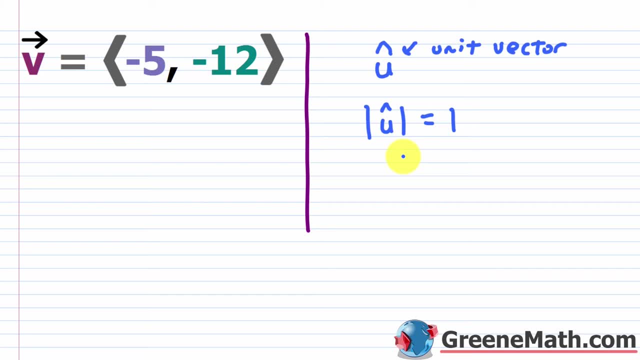 as a given non-zero vector. let's call it V. And basically, to solve this type of problem, you're just going to take your vector V and divide it by the magnitude of that vector V. Okay, And that's going to give you. 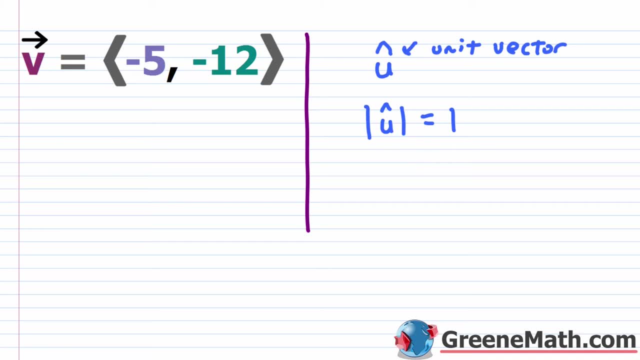 your unit vector U. Now, if you're confused by me saying it, it's okay. The formula is very, very simple. So, basically, this unit vector U is equal to the vector V. Okay, So the vector V divided by the magnitude. 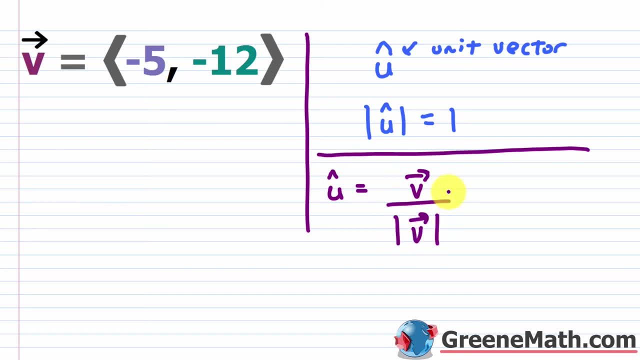 of that vector V. Okay, So you can really think about this as multiplying by a scalar one over whatever this is. So I'll further break this down and say: this is the vector V times one over whatever this result is. so the magnitude of this vector V: 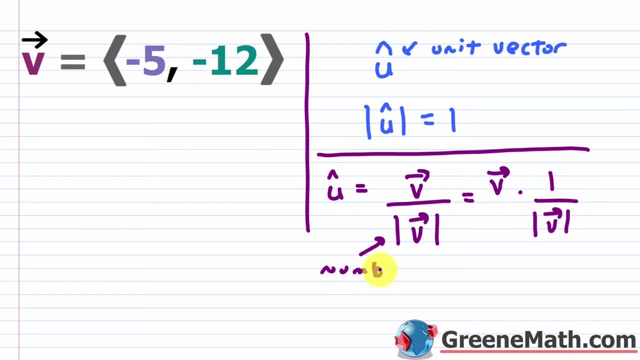 Remember, in the end, this is going to be a number, Right, This is some number, Okay. So if I wanted to practice on this one, let's say this: vector V- okay- has a horizontal component of negative 5 and a vertical component of negative 12,. 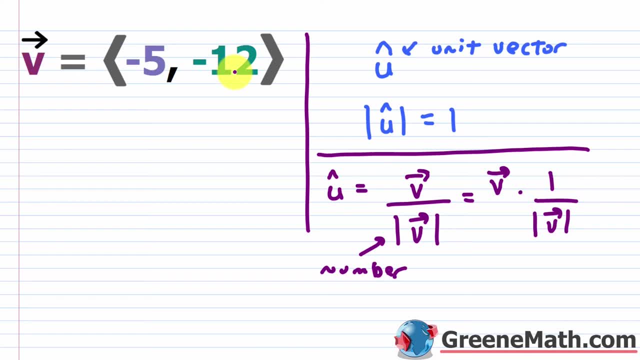 how would I find the unit vector U in the direction of V? So basically in the direction of V, but now I have a magnitude of 1.. So what I would do is I would first find the magnitude of V, so the magnitude of V. 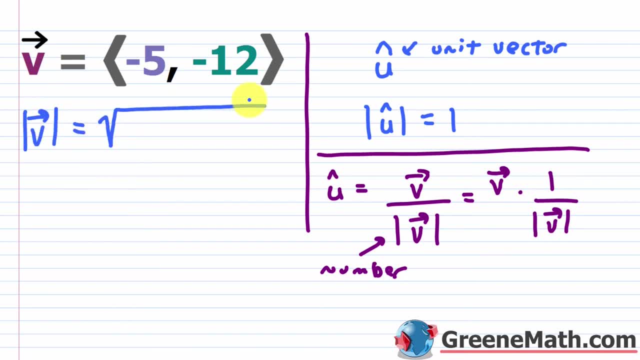 Hopefully you remember that formula. You're going to take the square root of. I'll have negative 5 being squared plus negative 12 being squared. So each one of these guys is going to be squared and you're going to find the sum of those two results. 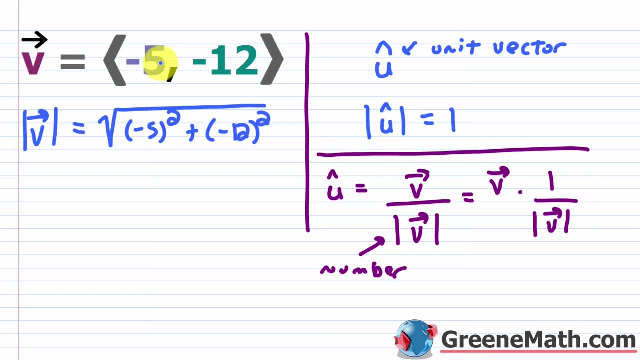 Okay, So I know negative 5 squared is 25,. negative 12 squared is 144.. So this would be my vector V. the magnitude of that guy would be: the square root of 25 plus 144 is 169, and the square root of 169 is 13.. 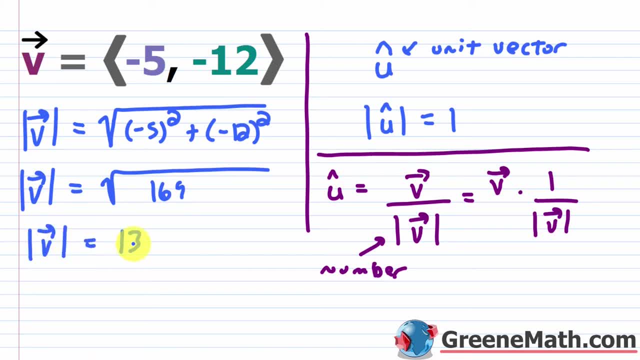 Right, So the magnitude of this vector V is going to be 13.. Okay, So that's easy enough. Once you have this result, you can basically just divide. okay, divide each one of these components by the magnitude of that vector and you're done. 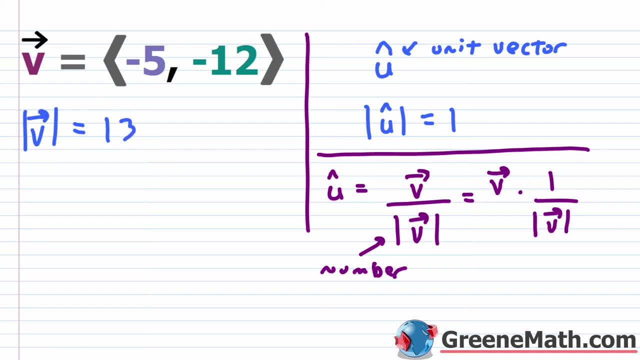 Right, You've set up your unit vector U. Okay, But if you want to kind of go about this the long way, let's just go ahead and use this formula here. So you have your vector V. I'm going to write it. 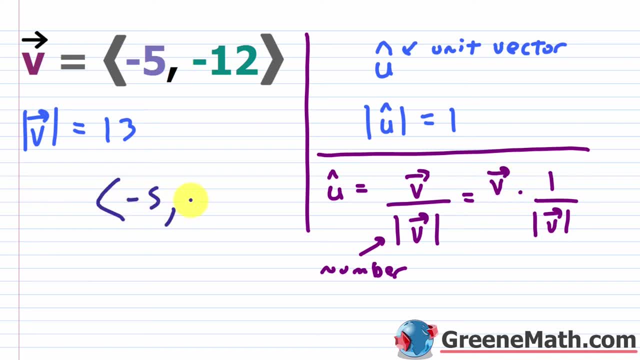 in component form. So I'm going to say this is negative 5 comma, negative 12.. Let me make these a little bit wider, Okay, So it's more consistent, So like that, And I'm going to multiply by 1 over the magnitude. 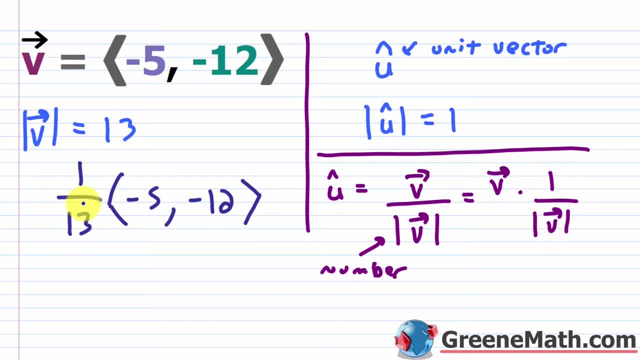 of that vector V, So 1 over 8. In this case it's 13. So you can see, this is just a scalar multiple Right. So I can either multiply by 1 over 13 or I can just divide by 13.. 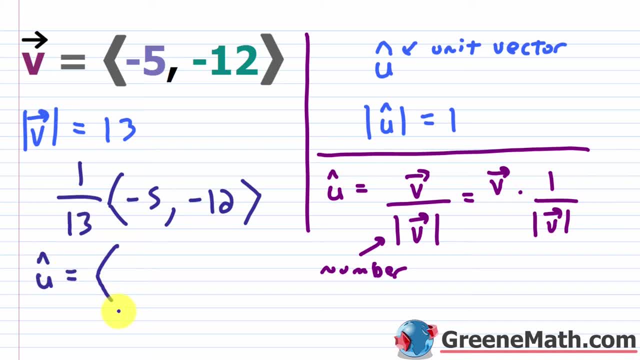 Doesn't matter, Right? So in the end, my unit vector U- okay, would be equal to in component form. you'd have negative 5 over 13 comma, negative 12 over 13.. Okay, That's all you need to do. 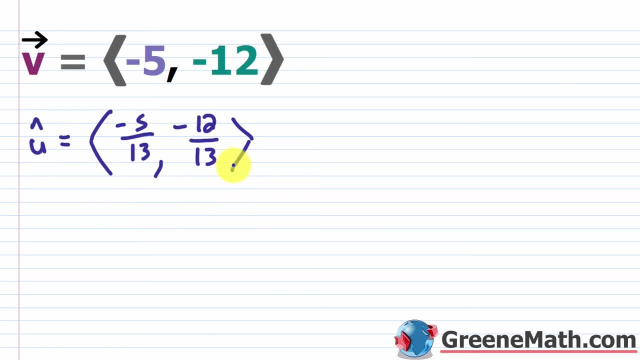 I want to prove a few things to you. One, that the magnitude of this vector U is 1, and also that the direction angle is the same. So the magnitude of this unit, vector U, is going to be the square root of. so let's go ahead. 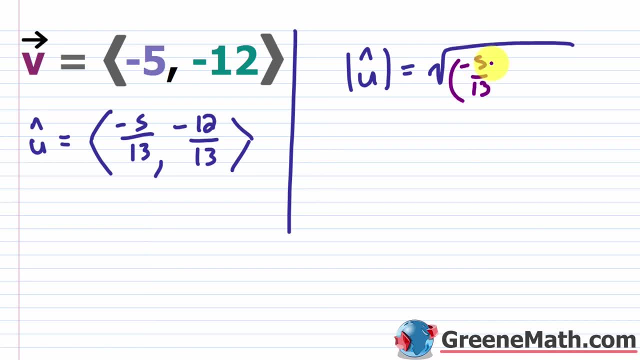 and say this is going to be negative 5 over 13 being squared. plus, you're going to have negative 12 over 13 being squared. Okay, So negative 5 over 13. if you square that, negative 5 squared is 25,. 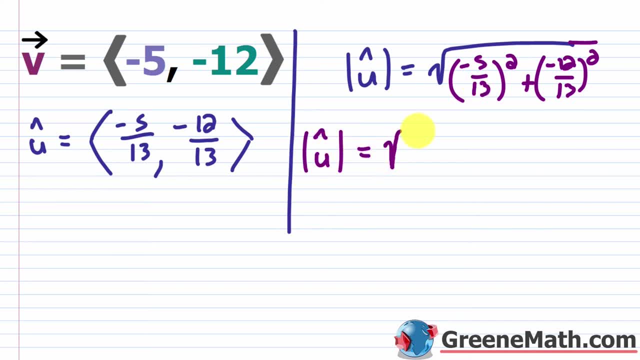 13 squared is 169.. So let me write this down here. The magnitude of this vector U is going to be equal to. the square root of this would be 25 over 169, plus 12 squared is 144, and then 13 squared. 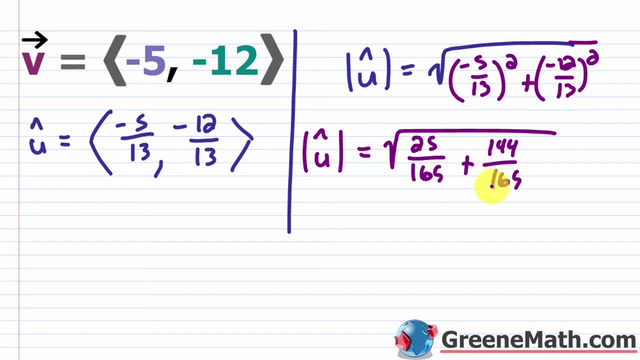 again is 169.. Okay, So if you add these guys, you have a common denominator. 25 plus 144 is 169.. So you get the square root of 169 over 169.. This is obviously 1, and the square root of 1 is 1.. 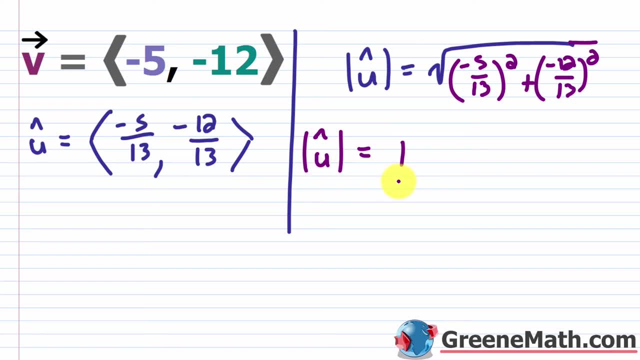 So you can see the magnitude of this unit. vector U is 1.. Okay, So that part works out. Now, what about the direction angle? Okay, You're going to see that. basically, if you think about the direction angle, remember the tangent. 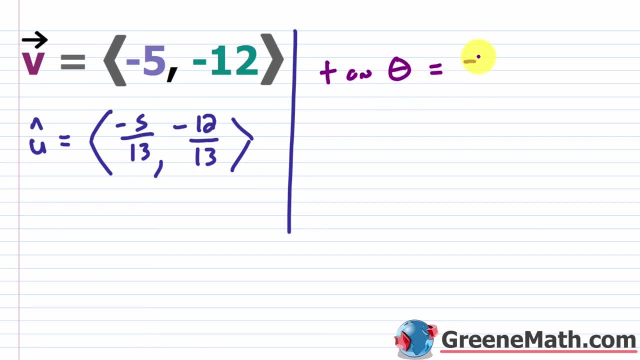 of theta is going to be equal to this negative 12.. Okay, Over this negative 5. Right, Which in this case you might as well just say it's 12 fifths Right. But again we have to think about what quadrant we're in. 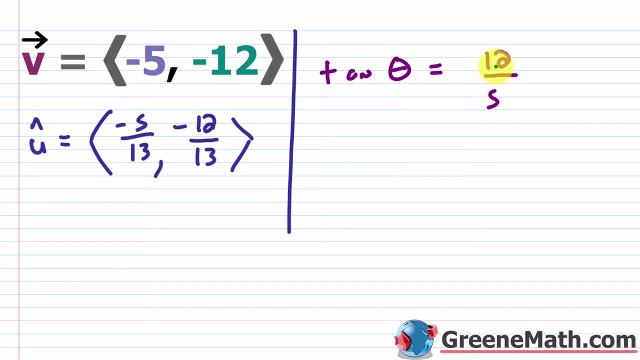 because if we do the inverse tangent- Okay, We're going to. in this case, because this is positive- we're going to get something in quadrant 1.. Okay, But this is in quadrant 3, because we have a negative x value and a negative y value. 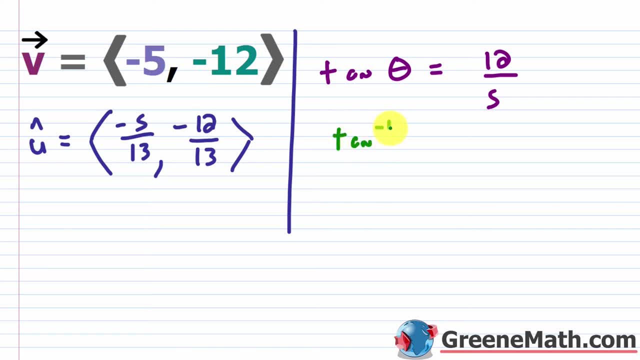 So I go to the left and I go down, so I'm in quadrant 3.. So what I want to do here is I'm going to say that the tangent of this 12 fifths here would be equal to- or let's say approximately, because we've got to. 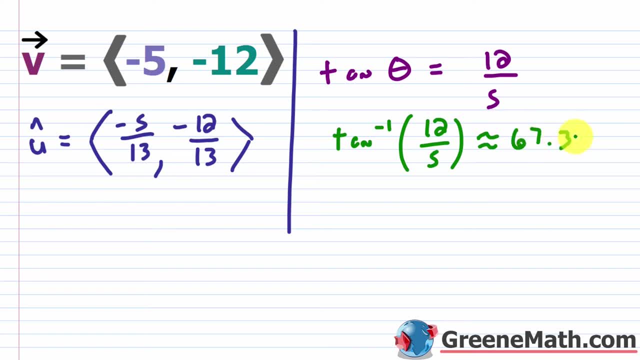 punch this into a calculator, I get about 67.38 degrees. Okay, And because we're in quadrant 3, we want to add 180 degrees to this. Okay, To get our measurement for theta. Okay, So we'll say theta. 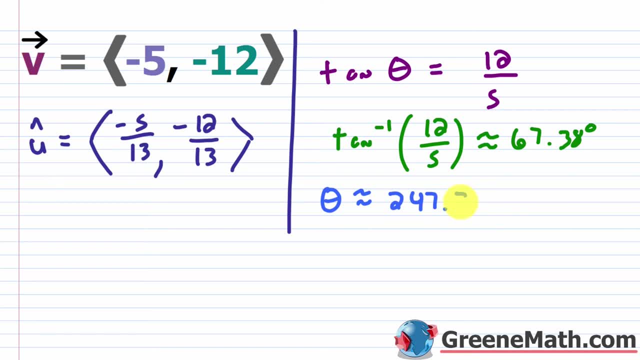 is approximately, I'll say- 247.38 degrees. Okay, So this is your direction angle. You already know how to find that. Now, if you look at it for this unit, vector u, you'll notice you're still in quadrant 3.. Right, 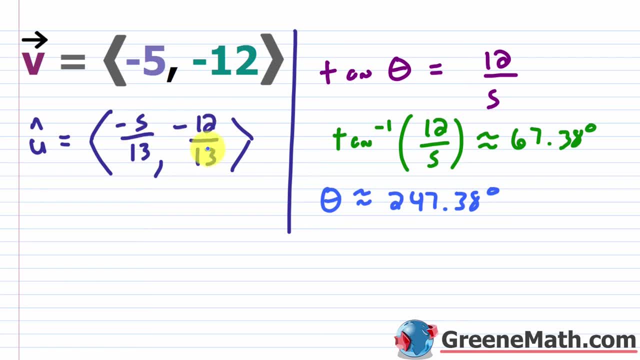 This is negative and this is negative. Okay, So you're still in quadrant 3 and I want you to think about the fact that you still have. tangent of theta is equal to now. it would be negative 12 over 13 divided by negative 5 over 13.. 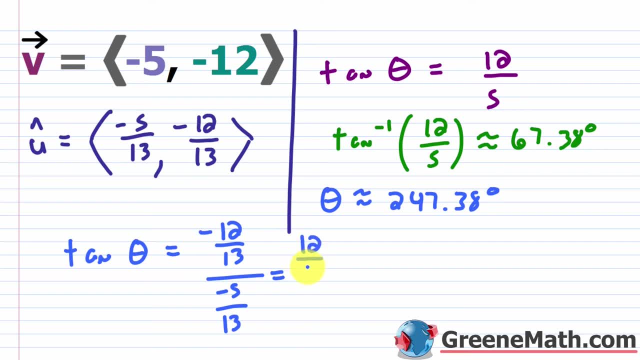 Well, the negatives are going to cancel, Right, So you'd have 12 over 13 times. flip this guy: 13 over 5. Okay, And the 13s are going to cancel. so I'm back to this. so the tangent of theta. 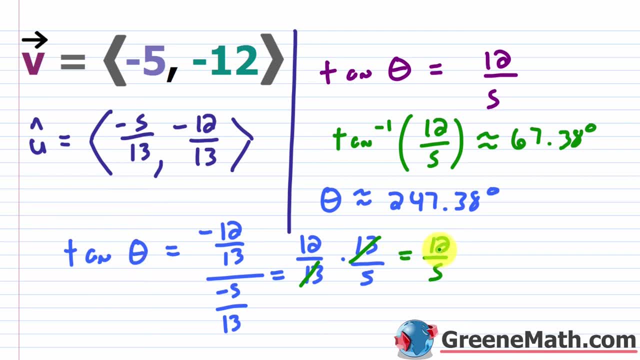 is equal to 12 fifths. and again, I'm still in quadrant 3, so I go through the same steps and I'm going to end up with a theta here. okay, my direction angle, which is again approximately 247.38 degrees. So you see that. 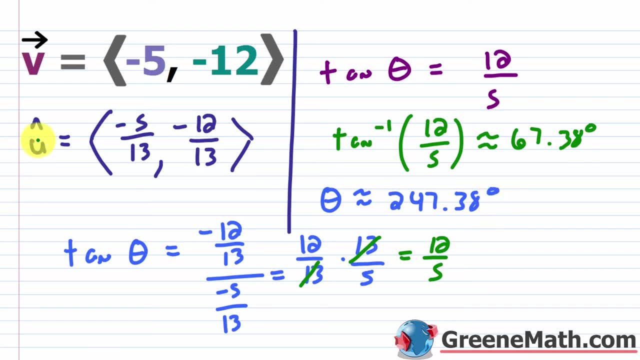 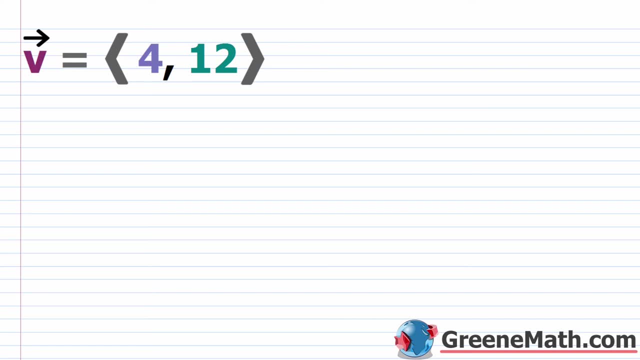 we've set up this unit vector u that has a magnitude of 1 and it's in the direction of our vector v. Alright, let's change our problem up just a little bit. So sometimes you'll be asked to find a unit vector u, basically. 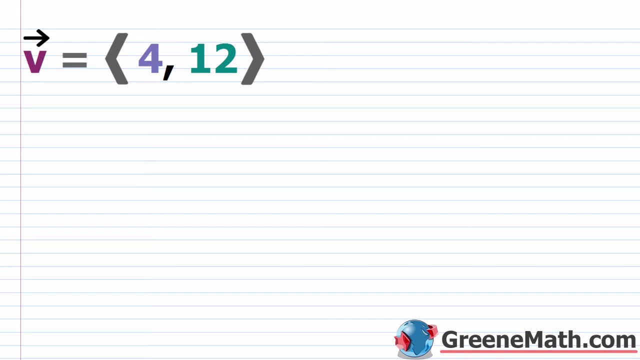 in the opposite direction of some vector v. All you really need to do here is think about the concept of: well, if I multiply a given vector by negative 1, it's just that vector that has the opposite direction. Okay, Same magnitude but in opposite direction. 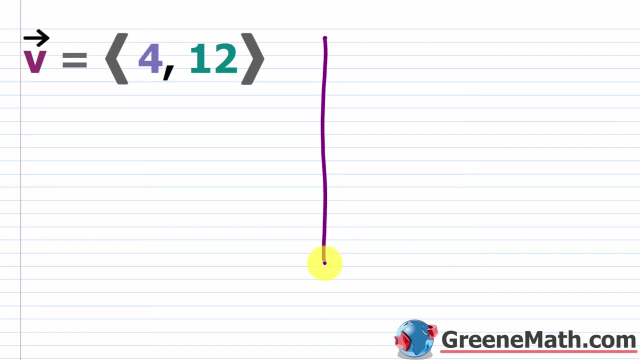 Okay, So we're going to use that concept here and just multiply our regular answer by negative 1.. So in other words, I would have my unit vector u is going to be equal to. we'll have this vector v times what I'm going to do here. 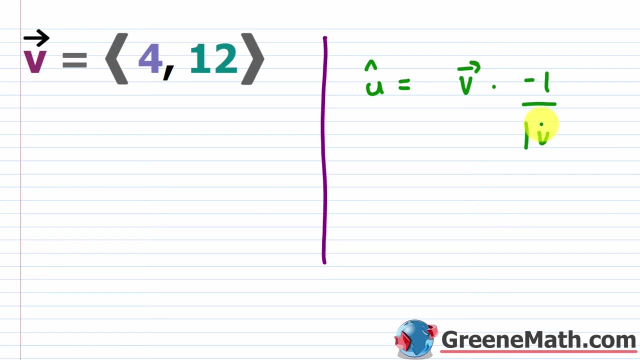 is put negative 1 okay, over the magnitude of this vector v. So let's go ahead and find the magnitude of our vector v. So the magnitude of this vector v is going to be equal to the square root of. so 4 squared is 16. 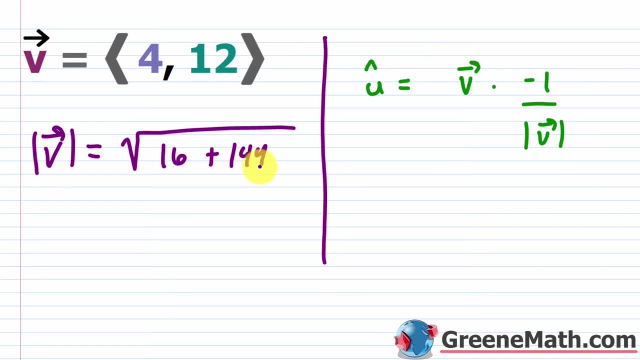 plus 12 squared is 144.. If you add these guys together, you get 160, and what I can do is I can factor this and say this is 16 times 10. okay, 16 is a perfect square, so this would be 4 times the square. 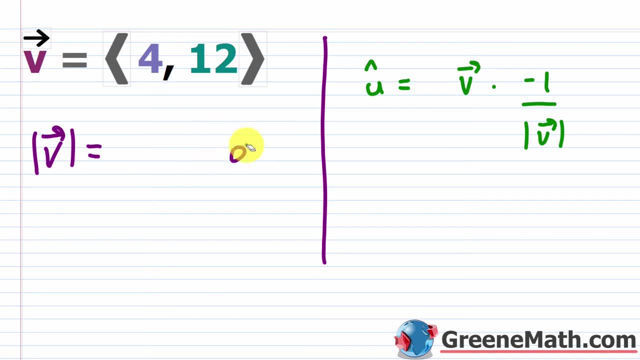 root of 10.. Okay, So I'll say this is 4 times the square root of 10.. Now, all I'm going to do here is either divide everything by the negative of this guy right here, or you can say multiply by negative 1. 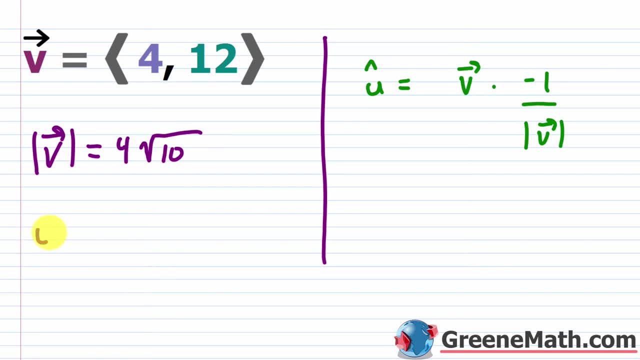 over that guy. whatever you want to do, I'm just going to make this a little bit quicker and say my unit vector u that I'm looking for in this case is going to be: I'll take the 4, okay, and I'm going to divide it. 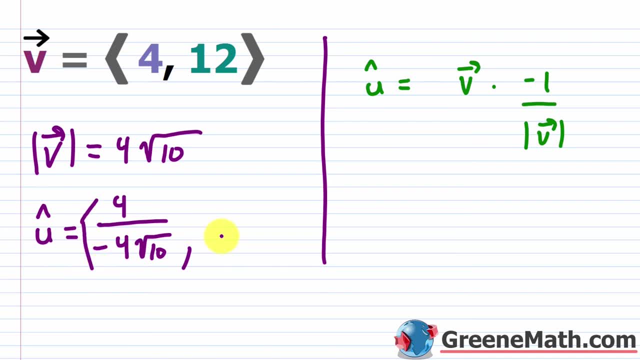 by the negative of 4 times the square root of 10. okay, and then let me put my angle brackets in here, and then I'll have my 12, and then I'm going to divide that by the negative of 4 times the square root of 10.. 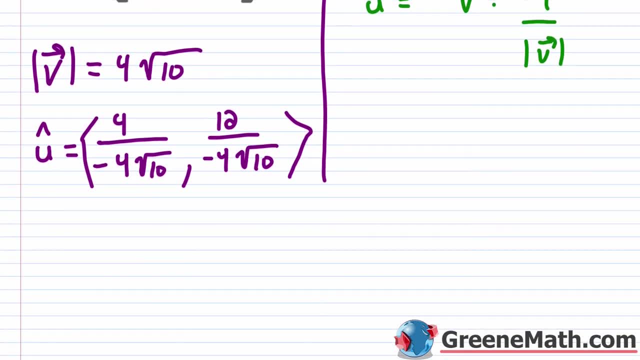 So what I did? it's a negative 1 there, so that's why these are negative here. okay, let me get some room going here, so let me go ahead and set this up as the unit vector u is equal to put my brackets there, so we know. 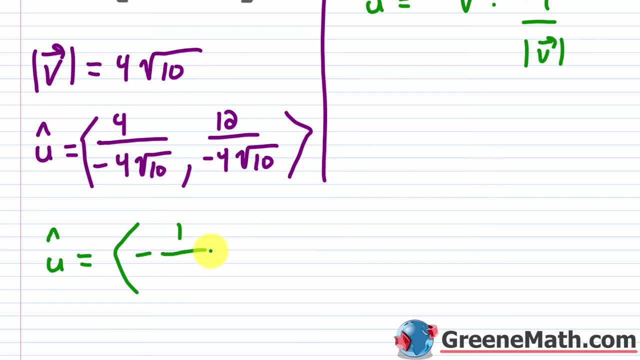 we're going to have to rationalize the denominator there. so 4 divided by 4 is 1. so let me put a negative out in front, let me put a 1 over the square root of 10 and I'll just multiply this by the square root of 10. 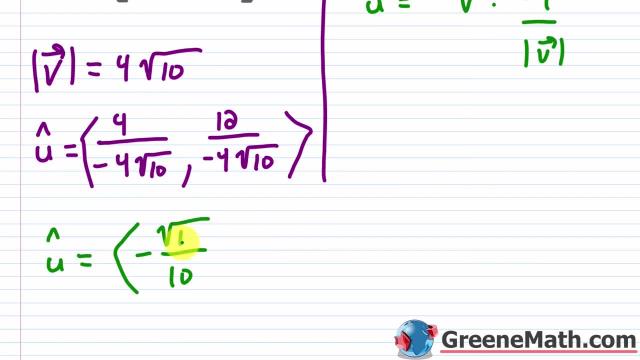 over the square root of 10 to get that out of the way. so this becomes 10 down here. okay, so it's common to not rationalize the denominator for these examples. it's really up to you or your teacher, just get with them and see what they want. 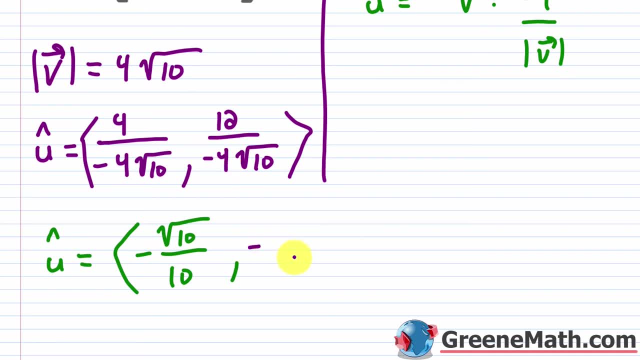 you to do. for this one, we have 12 divided by 4, which is 3, and of course you have the negative. so let me go ahead and put 3 over the square root of 10 and again I'm going to rationalize the denominator. 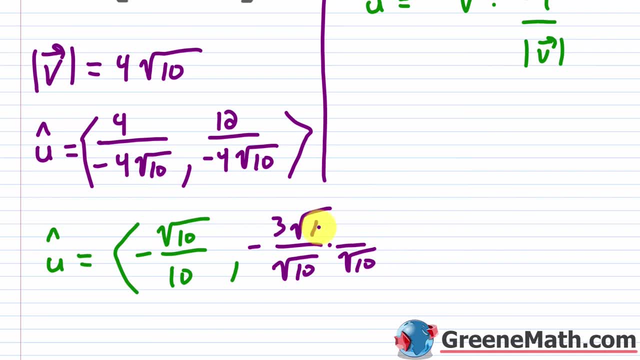 so times the square root of 10 over the square root of 10. okay, so I'm going to multiply by that. so in the numerator I'd have 3 times the square root of 10 over the square root of 10. so what would work? 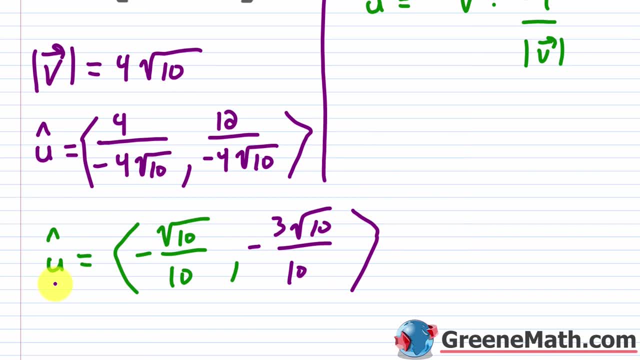 is, you would have this unit, vector u, which again is in the opposite direction of my vector v. the horizontal component is negative square root of 10 over 10 and the vertical component is negative 3 times the square root of 10 over 10. okay, 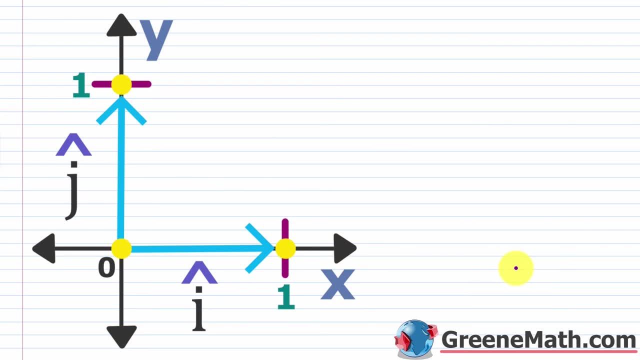 alright, so let's continue to talk about these unit vectors, and now you're going to see these two extremely useful unit vectors, which are defined using this i and also this j. okay, so you see on the screen, here we have this little graph, you have a directed. 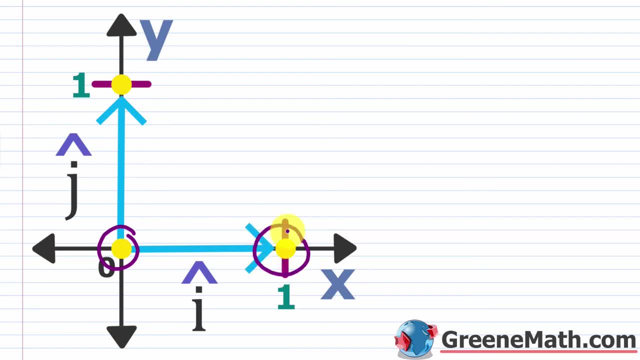 0, 0,. okay, and ends or terminates at the point 1, 0.. So the initial point is 0, 0, or the origin, the terminal point, is 1, 0.. So we have this unit vector i. okay. in component form, this is 1, 0,. 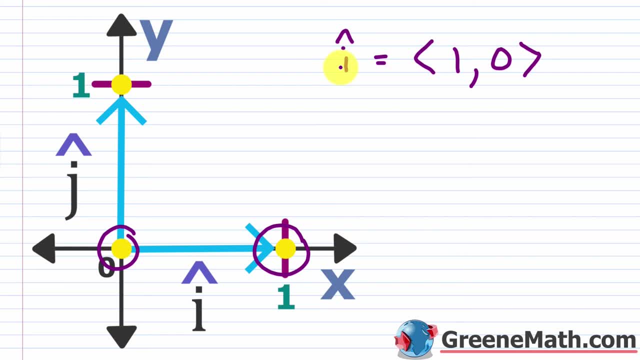 like this: okay, This is not the imaginary unit i, so please don't get confused by that. Then, similarly, we have this guy that is denoted with a j, So we'll say j here with my little hat. So this guy, it terminates at 0,, 1, okay, And basically we're going to use this guy. 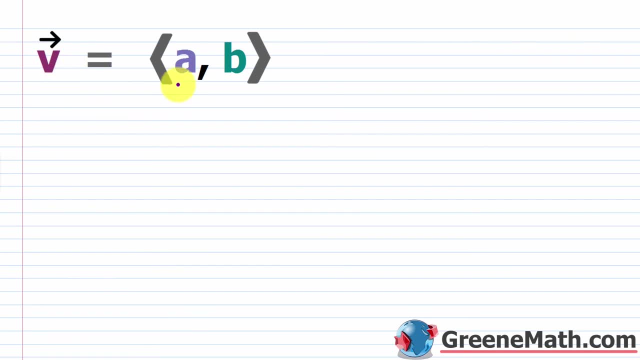 to rewrite something like this. So our vector v in component form, we have a comma b, okay, But using those two vectors, i and j, basically what you can do again, because the vector i in component form is 1,, 0, okay, and the vector j in component form is 0,, 1, you can take your. 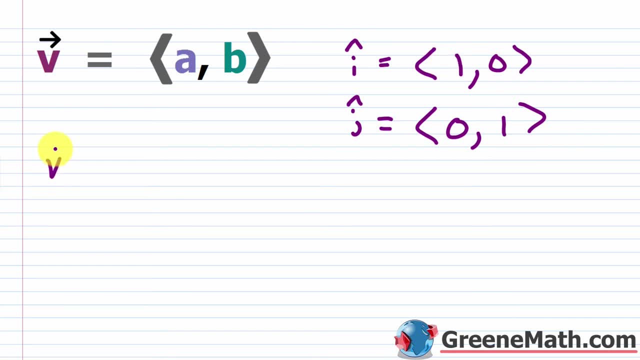 horizontal component and multiply it by this guy. So let's say the vector v. I could also define it saying it is this: a multiplied by this 1,, 0,. okay, Then plus- and I probably need to move this down a little bit- so plus this b here, multiplied by this guy. 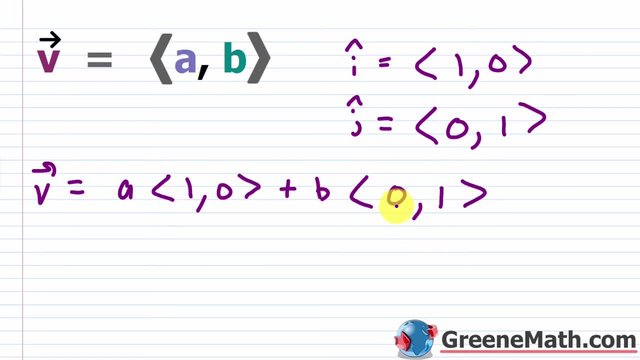 0, 1, okay. So you know that these are just scalar multiples. at this point, If I multiply through, this is basically a- 0, okay. Plus this is 0, b- okay. And then if I add these two together, 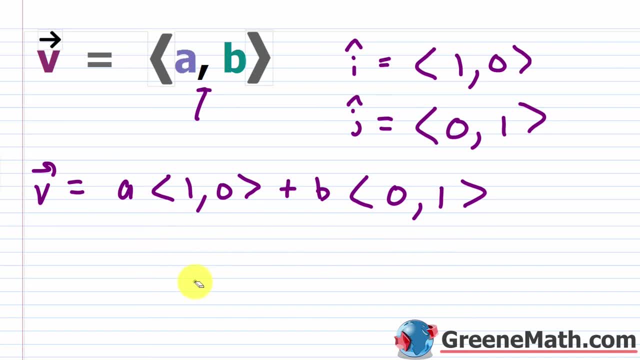 I'm right back to what I started with, So I just have to go back to what I started with. So I just have to go back to what I started with. So I just didn't do anything illegal. Now, what you can do at this point is just replace in each case. 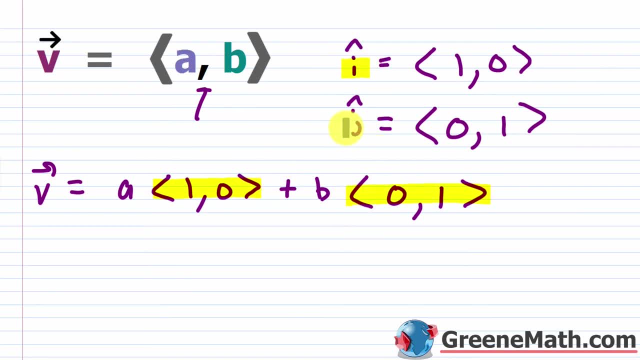 this with the unit vector i and this with the unit vector j. okay, That's all you're going to do. This is called writing it in the i comma j form, or you might hear it as a linear combination of the standard unit vectors i and j. okay, So I'm going to say the vector v now is going to. 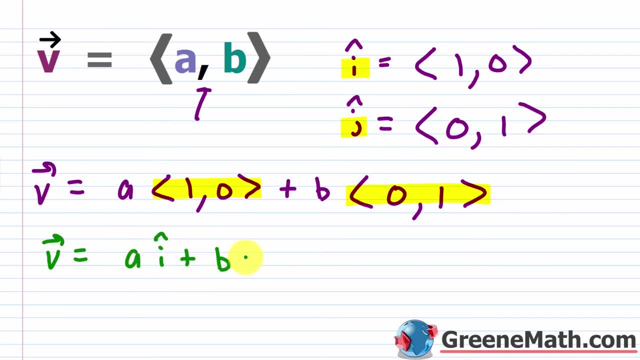 be written as a times the unit vector i plus b times the unit vector j. okay, So if you see something in this form, to put it in component form, basically again, the vector v is what It's, just in component form. this is your horizontal. 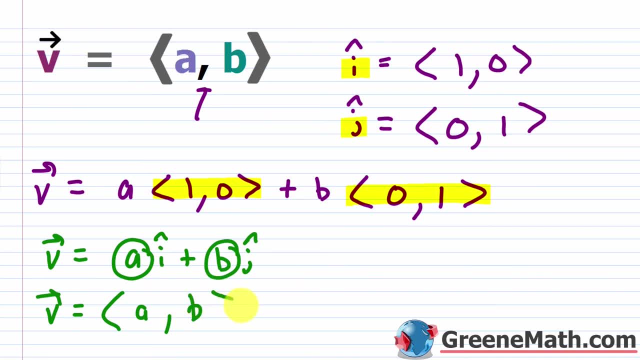 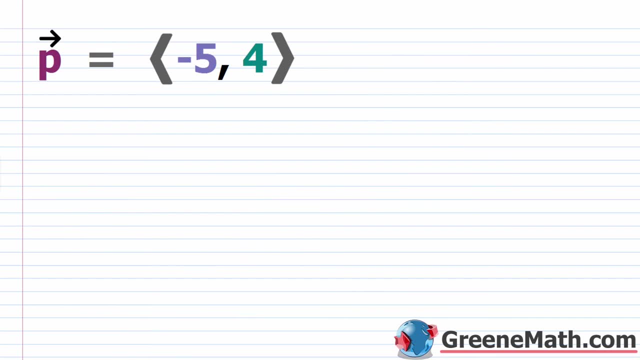 component right And then comma. this is your vertical component. That's all. it is okay. If we look at a little example here, let's say I have some vector p and I want to write it as a linear combination of those two standard unit vectors i and j. 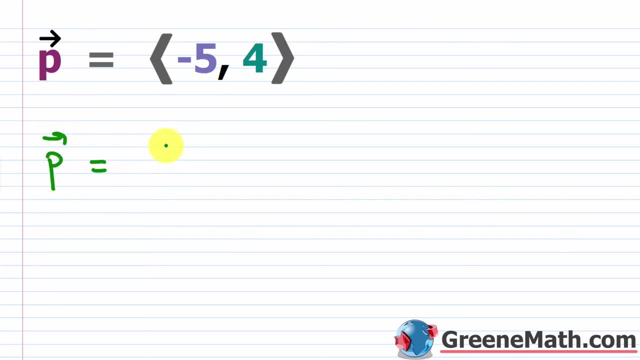 all I'm going to do? I'm going to say: this guy p, this vector is negative, 5, this is the horizontal component- multiplied by this unit vector i- okay. Then plus this guy 4, okay, Multiplied by that unit vector j. That's all it is. Again, if you go back through this, the 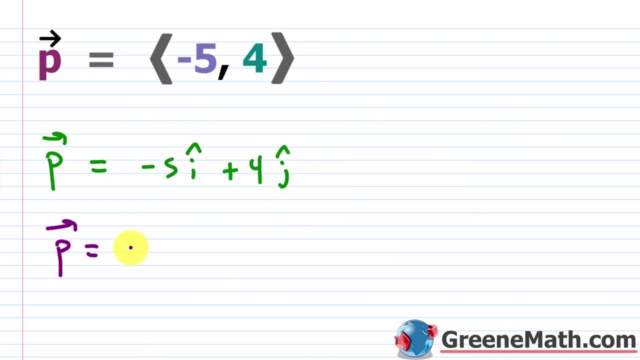 long way. all you're really saying is that this vector p is equal to. you'll have negative 5 times. this is what: 1 comma 0, then plus 4 times, this is 0 comma 1.. And again, all I'm doing is: 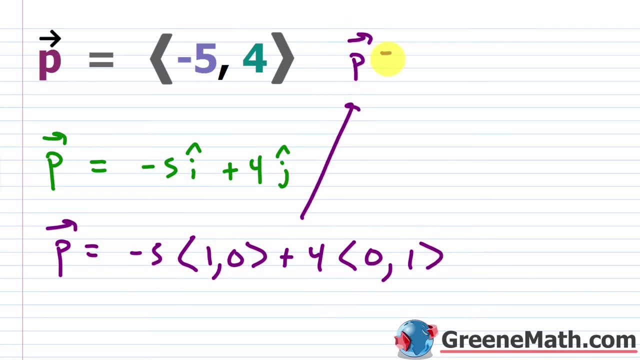 if I kind of move this up here because I'm going to run out of room, this vector p is what? Now it's negative 5, okay, comma 0, plus, and let me move this down a little bit so I can fit everything. 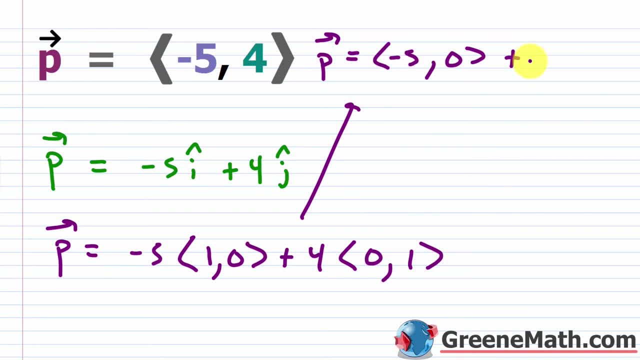 let me change this up a little bit. and then I'm going to write this vector p: okay, This vector p is going to be negative 5 plus 0, which is negative 5, and then comma 0 plus 4 is 4,. okay, So it's just. 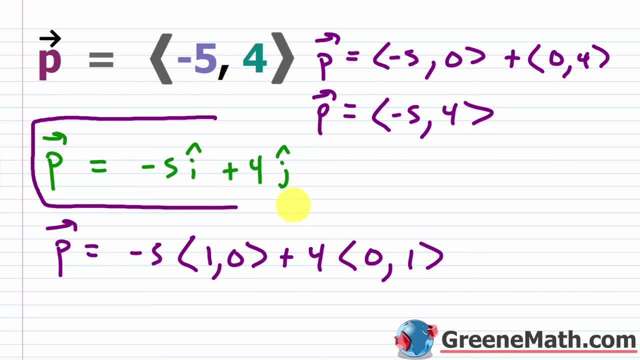 two different ways to write the same thing. This way, right here, you're going to see a lot okay, So you need to know how to go back and forth between the two. If you wanted to graph something like this, the terminal point is going to be at negative 5, comma 4.. So if we looked at this, 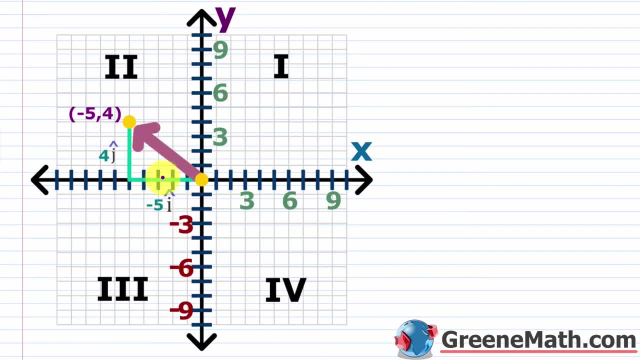 this on our little coordinate plane. here Again, the horizontal movement here is given by the negative 5 times this unit vector. i okay, It's just basically like if I said the horizontal movement here is given by this negative 5 comma 0, right, Let me make that a little bit better. 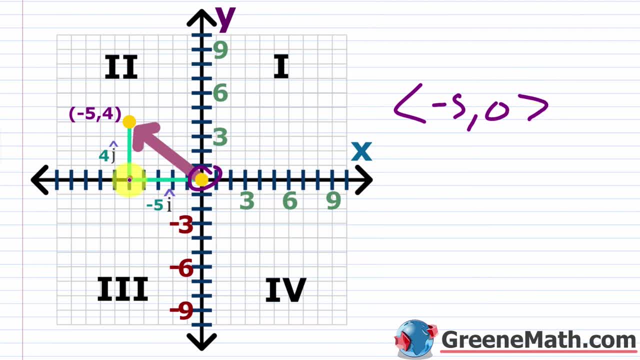 So, basically, if I started here and I went five units to the left, I end up right there. Okay, that's my horizontal movement, given by this negative 5 times the unit vector. i. Then for the vertical movement, if I'm starting here and if I go up, well, basically this is given by 4 times the 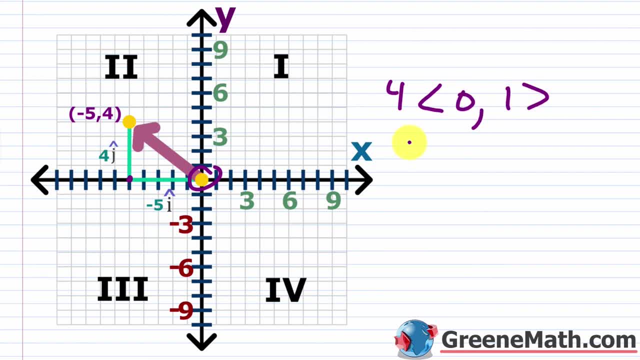 unit vector j right, 4 times the unit vector j right. So it's going to be the horizontal movement times that 0 comma 1, like this. So this is 0 comma 4, right, I'm just moving up four units. 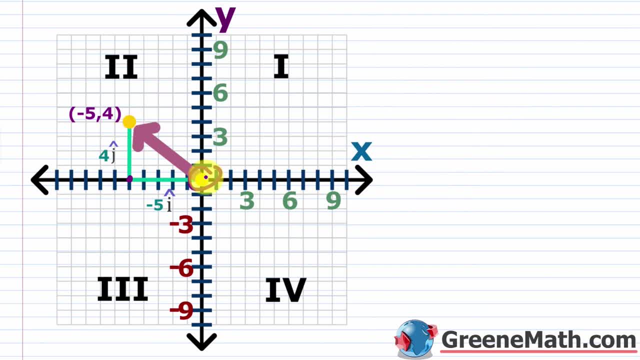 vertically. So when you put those two guys together, you end up with this directed line segment with a terminal point at negative 5 comma 4.. Five units to the left, four units up. So that's all. it is All right. let's talk about something called the dot product now, And this is going to 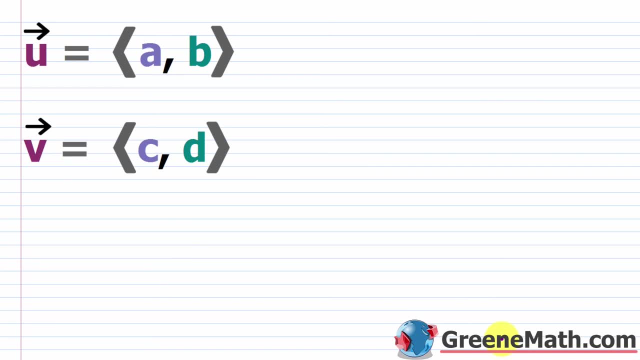 lead us into a topic called finding the angle between two vectors. okay, So we start with the dot product, and the dot product of two vectors is going to be a real number, So this is not going to be a vector. This is also called the inner product. okay, So someone might refer to it that. 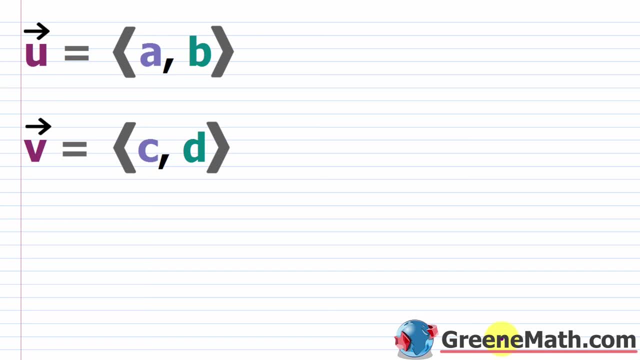 way. Now the dot product for us is going to be used to determine the angle between two vectors and we'll get to that shortly. So when you have the dot product of two vectors, let's say u and v. So I have u and v, those two vectors. I'm going to write the vector u, then dot the vector v. 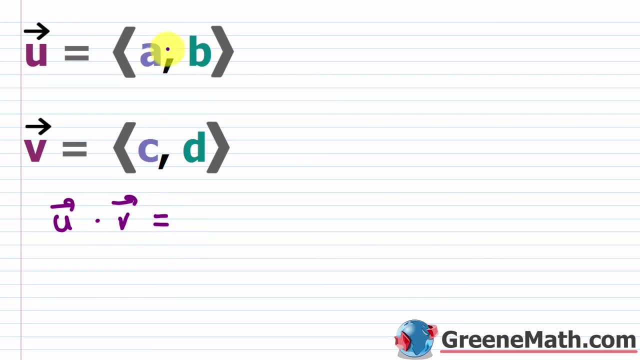 okay, So this is the dot product And basically all I'm going to do is I'm going to multiply the first component here by the first component here, So a times c. So in other words, horizontal component times horizontal component, then plus second component. 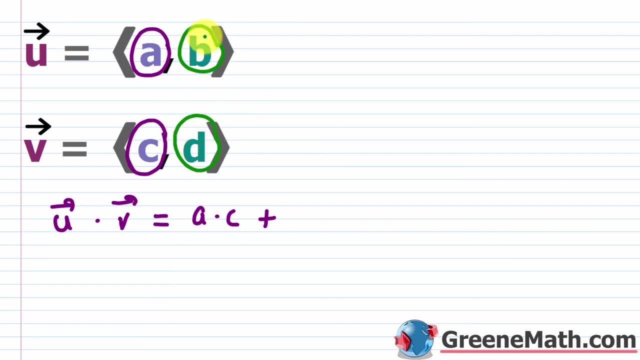 here times second component, here, So vertical component. here times vertical component. here, So b times d. It's a very easy pattern to remember. Once you do a few examples, it just becomes second nature. okay, So let's look at an example. So we want to find the dot product. 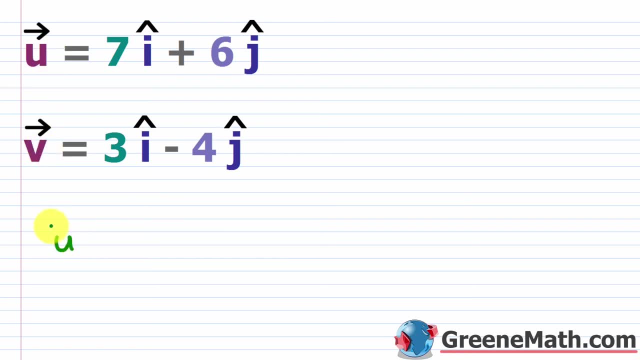 of this vector u and this vector v. So you're going to do the vector u dot the vector v like this. And again, if this is confusing for you, because again it's as this linear combination of the unit vectors i and j, you can always put it in component form. So the vector u 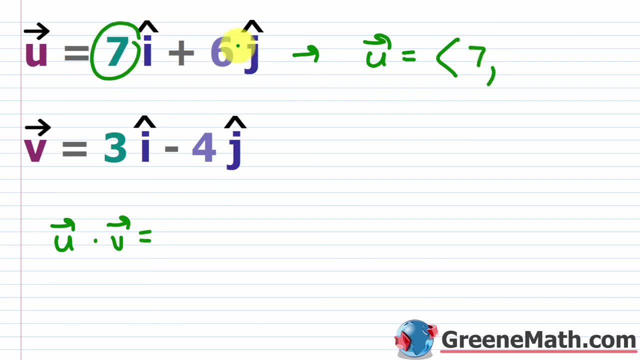 is again in component form. This is my horizontal component. This is my vertical component. okay, Do this a few times and then it becomes very easy, right? So the vector v: this is my horizontal component. this and the whole thing with the negative. So let me make sure I do that properly. 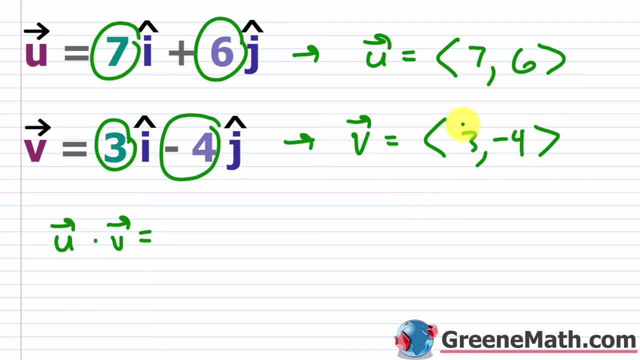 This is your vertical component. okay. So either way you want to do it, but all I'm going to do here is I'm going to say seven times three. So seven times three, So first times first. then plus six times negative four, So second times second. So six times negative four. That's all you're. 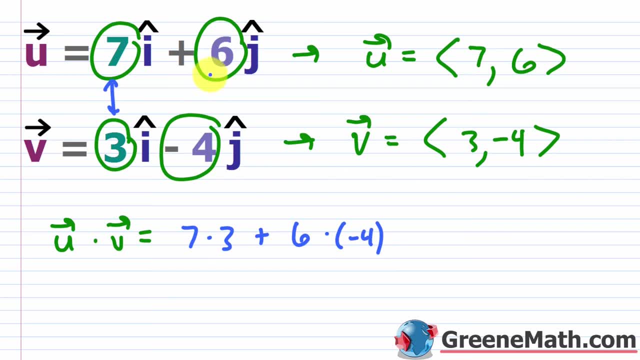 doing. okay. Just match things up and say these guys are being multiplied, and then these guys are being multiplied. That's all you got to do. So once you have this set up, seven times three is 21.. Then, basically, plus six times negative four is negative 24.. So this would be negative. 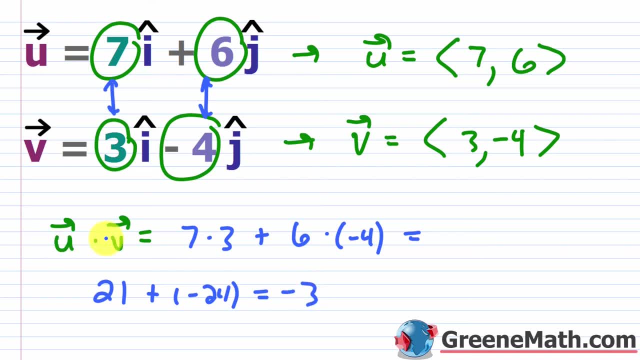 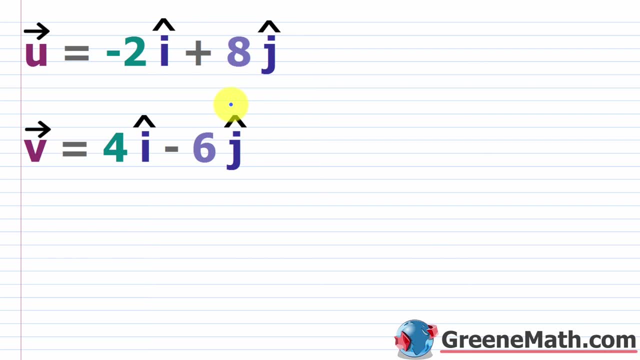 three. So that's your dot product of this vector u and this vector v. Okay, let's look at another example. If you want to pause the video and put these in component form, that's up to you. I think this. So the vector u is negative two times the unit vector i plus eight times the unit vector j. 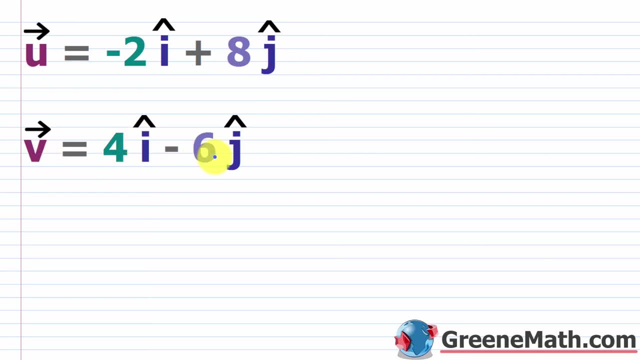 Then this vector v is four times the unit vector i, minus six times the unit vector j. So the dot product of this vector u and this vector v, so u dot v would be what You're going to have. this guy times this guy right. So first times first Negative, two times four, Then plus this guy times. 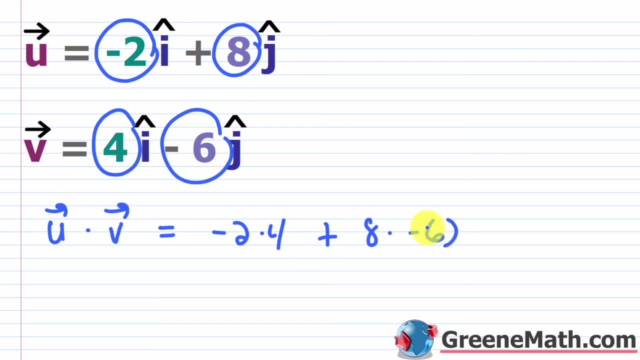 this guy. So eight times negative six, Eight times negative six, And again, if something's negative, make sure you take that with it, okay? So let's put equals here: Negative two times four is negative eight, And then plus eight times. 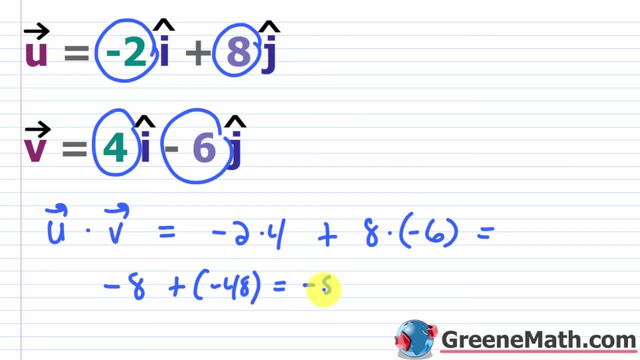 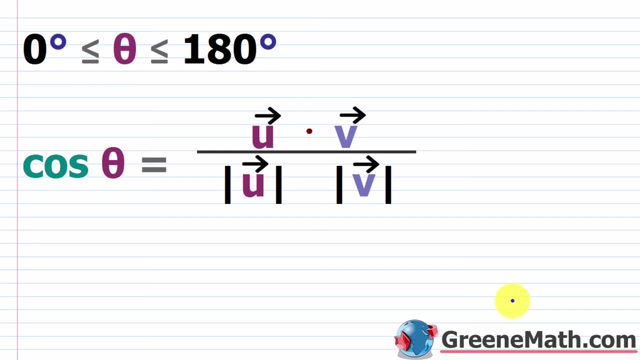 negative six is negative 48. And of course, this is really easy- This is just going to be negative 56.. All right, so now that we understand how to find the dot product of two vectors, we're going to use this now to find the angle between two non-zero vectors. So let's suppose 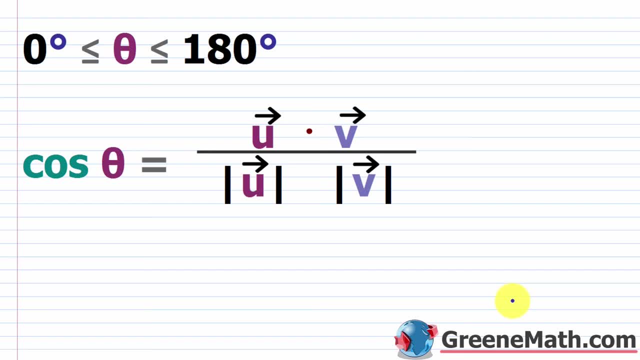 we have these two non-zero vectors, Let's call them u and v, okay, And we want to find the angle between them and we'll call this angle theta. So we'll say that theta is greater than or equal to zero degrees, and also less than or equal to 180 degrees. Or we could say theta is greater than. 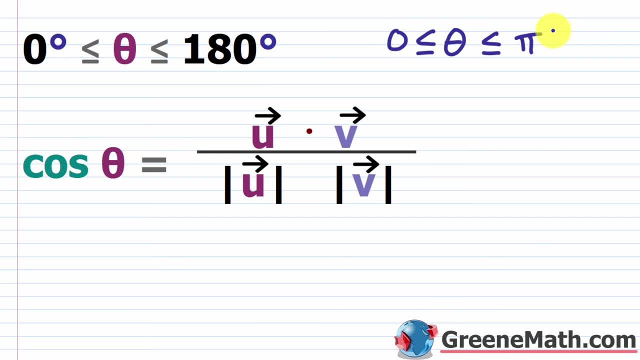 or equal to zero and less than or equal to pi if you want to work with radians. So we can come up with this little formula here. This is derived from the law of cosines, So we have the cosine of this angle. theta is equal to the dot product of this vector u and this vector v over you have. 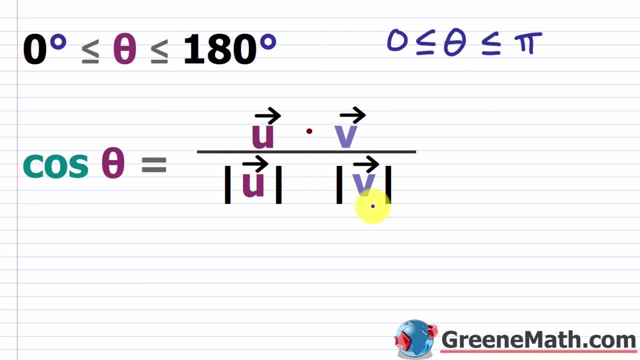 the magnitude of your vector u times the magnitude of your vector v. okay, So that's all it is. If you you're going to use your inverse cosine function, okay, you're just going to be punching this stuff into a calculator, So really really easy. All right, let's look at the first example We have. 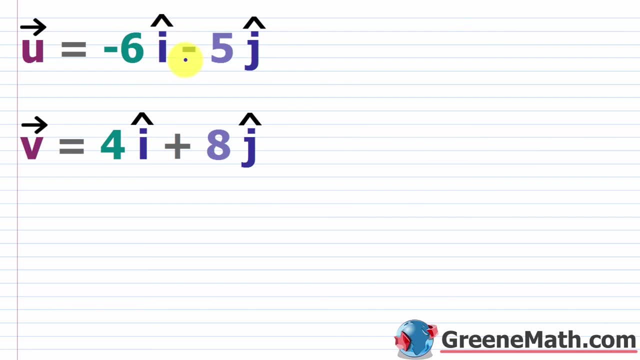 a vector u- okay- which is negative, six times the unit vector i minus five times the unit vector j. Then we have this vector v, which is four times the unit vector i plus eight times the unit vector j, okay. So if I want to basically set this guy up, first and foremost, if you're still confused by 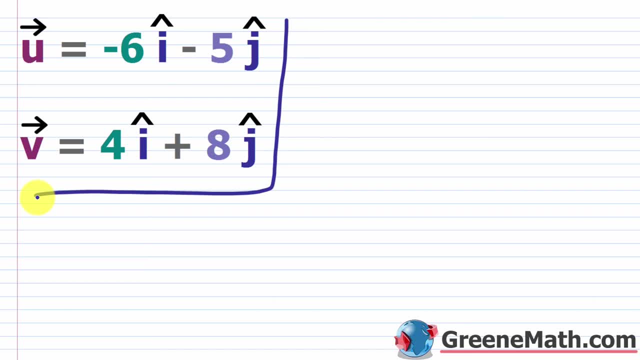 these linear combinations of the unit vectors i and j. you can always write this in component form to ease your confusion. Again, all I'm going to do to do that is take this guy as a horizontal component, okay, And then this guy is the vertical component. That's all I'm going to do. So if you're, 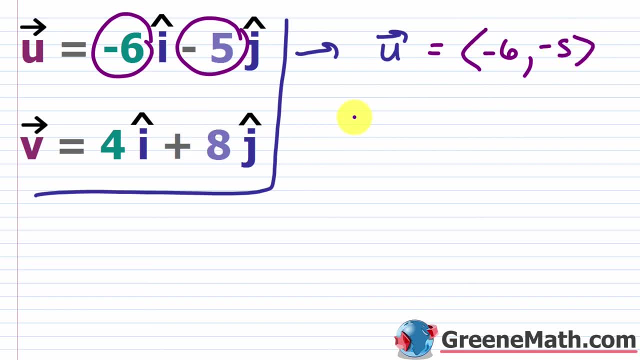 confused at this point. just do that for a little while And then eventually this will click for you. So then this guy, for the vector v in component form, it's going to be four comma, then you're going to have eight. okay, That's all it is. So if I want my dot product, okay, so the dot product. 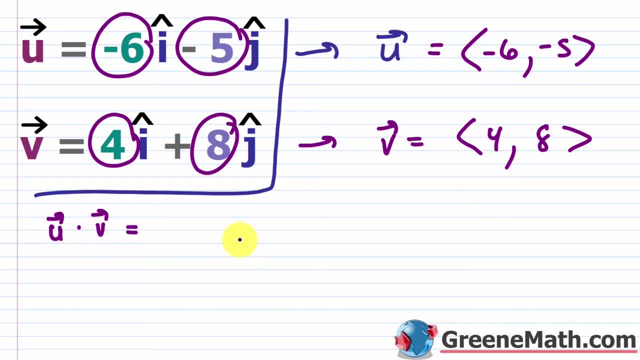 of this vector u and this vector v, this is going to be what Negative six times four, that's negative 24, then plus negative five times eight, that's going to be negative four. okay, So this gives me negative 64. Then, if I want the magnitude of this vector u, okay, this is going to be the. 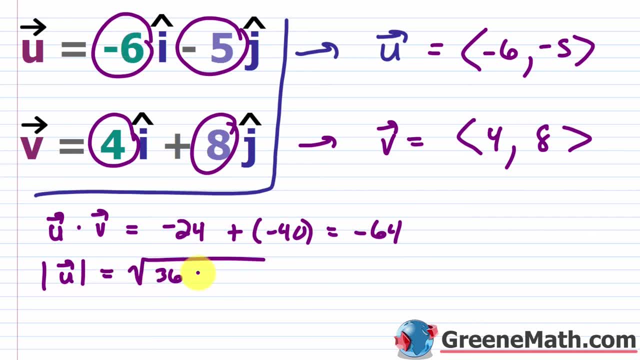 square root of. so I'd have negative six squared, that's 36, and then plus negative five squared, that's 25.. So this would be the square root of 61,. okay, Then the magnitude of this vector v- let me change my ink color here- this is going to be the square root of four squared is 16,. 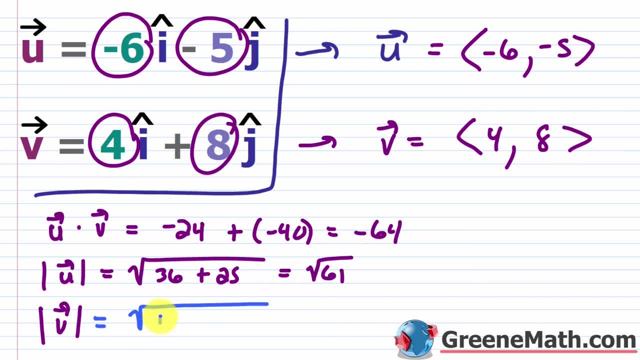 and then eight squared is 64. So 16, 64 would be the square root of 80. You could simplify that if you wanted to. Again, you're punching this stuff into a calculator, so if you're trying to save time, I wouldn't even worry. 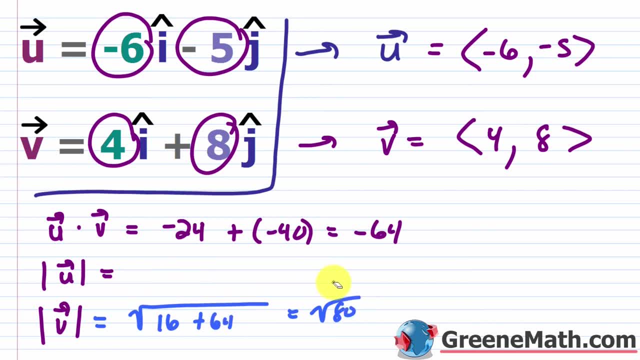 about it, But since this is a math tutorial, I'm going to take the extra step and write this down here. Let me just put this as a square root of 61.. Let me write this instead of the square root of 80,. 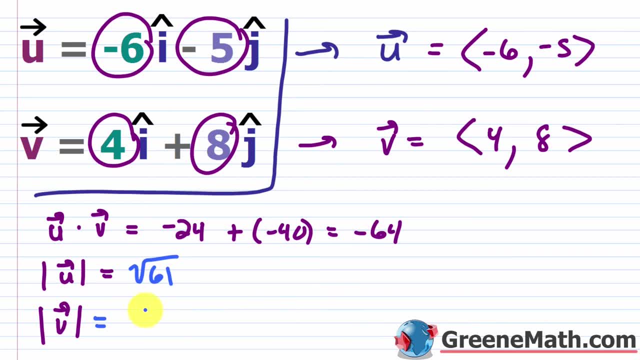 let me say that 80 is 16 times five and 16 is four times four, right? So I'm going to say this is four times square root of five, right? Because 16 is just a perfect square. Okay, so now we have. 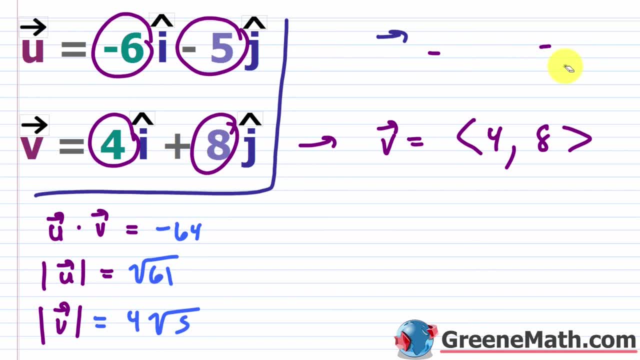 negative 64 here. Hopefully you have this copied down- I'm going to get rid of it because I need the room- And I'm basically going to write my formula here. So the cosine of theta is equal to, again, the dot product. so of this vector u, so the vector u dot the vector v, And then this is: 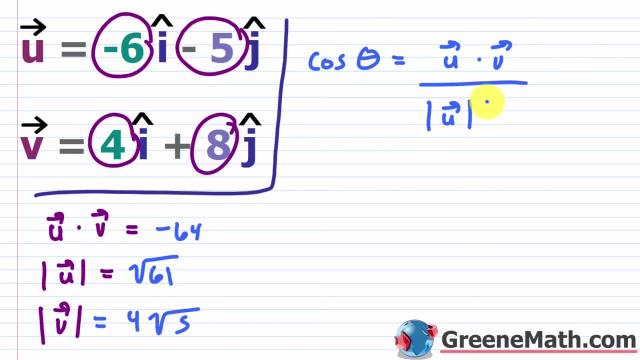 over the magnitude of this vector u, And then this is multiplied by the magnitude of this vector v. okay, So what I would do here is just plug in to the calculator And essentially you're going to say that theta is equal to the inverse cosine of theta, And then you're going to say that theta is. 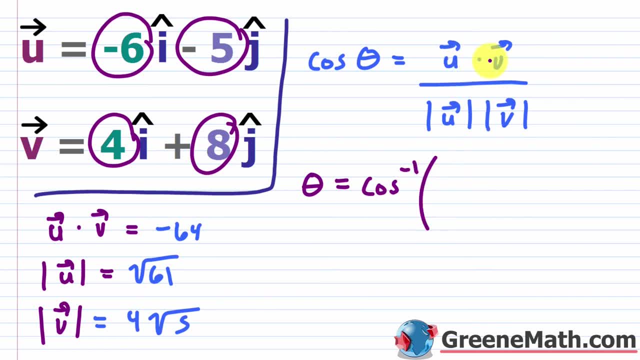 cosine of all this right. So your dot product of the vectors u and v. so this is going to be negative 64. Then over you're going to have the product of these two magnitudes. So the magnitude of vector u is square root of 61. And then the magnitude of vector v is four times square root. 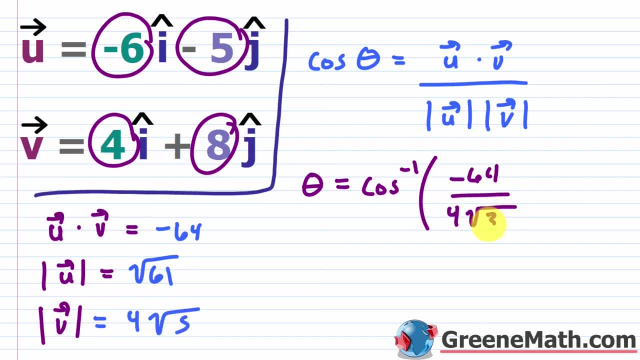 of five, So that would be four times the square root of 305,. okay, And again, you don't have to write all this out. If you're using a calculator, just punch it into it and you're done. But you might want to consider the fact that you should put parentheses around this. 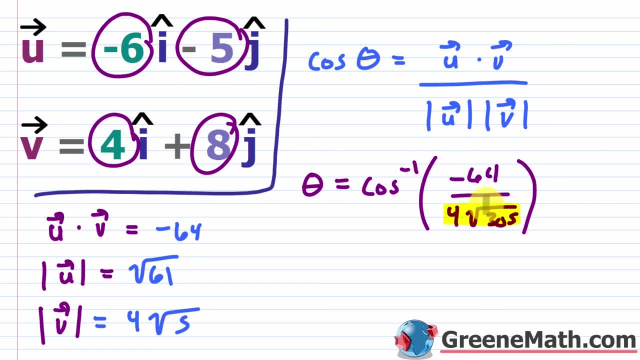 when you punch it into your calculator. If you keep getting the wrong answer, that's usually what's going on. It just depends on your calculator, okay. So what I would do is punch this guy into the calculator as the argument for the inverse cosine function, And I'll say theta is approximately: 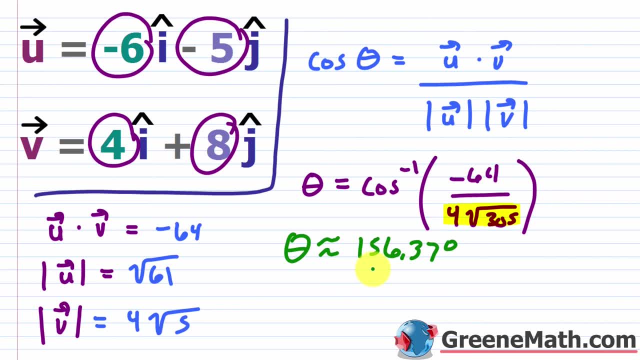 156.37 degrees. okay, So that's basically all you're going to do. And again, if you keep getting the wrong answer with your calculator, if it says something like domain error or something like that, then make sure you wrap this part right here inside of parentheses, and that should clear that. 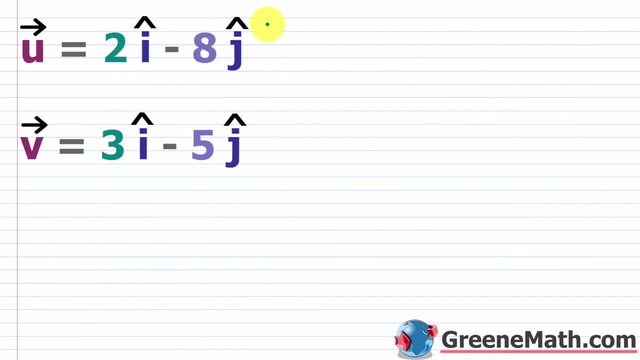 for you. Okay, let's take a look at another one. We should know the formula at this point. Let me go ahead and do the dot product first. So the dot product of u and v. so u dot v here is going to. 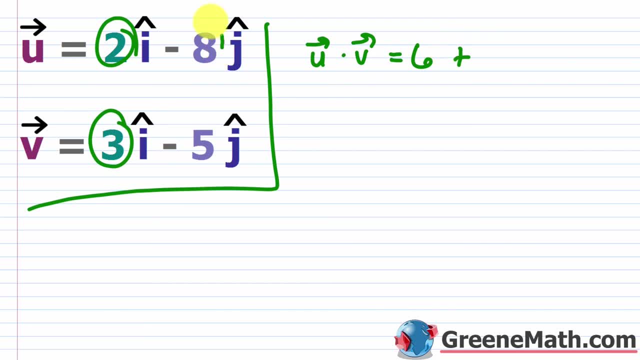 be what? Two times three, which is six, plus negative eight times negative five, which is going to be 40.. So this is 46,. okay, And then basically the magnitude of this vector u is the square root of you have two squared, which is four. then, plus, you have negative eight squared. 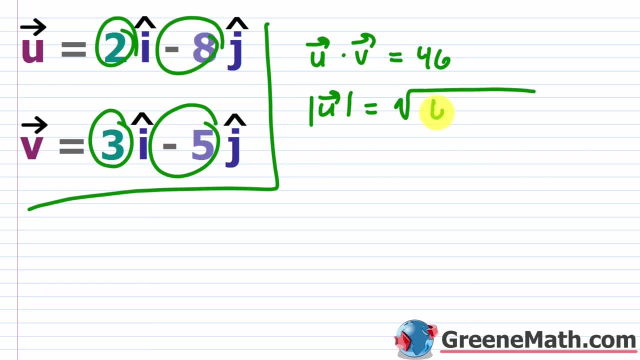 which is going to be 64.. So four plus 64 is 68, right, So square root of 68,. again, you could simplify that: It's 17 times four, So it's technically two times the square root of 17.. Now 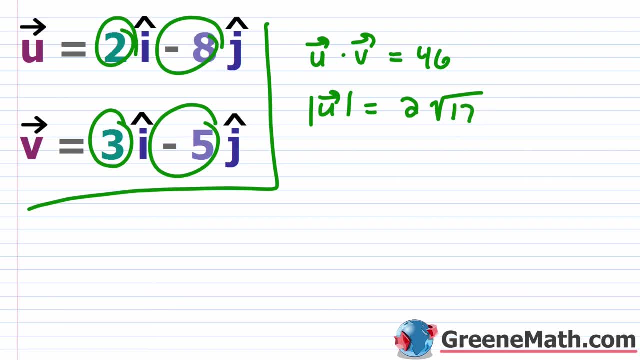 again, if you punch this into a calculator, you know who cares. But I'm just writing this down for the sake of our tutorial. okay, Now the magnitude of the vector v. we're going to have what You have. the square root of three squared is nine. then, plus negative five squared is 25.. 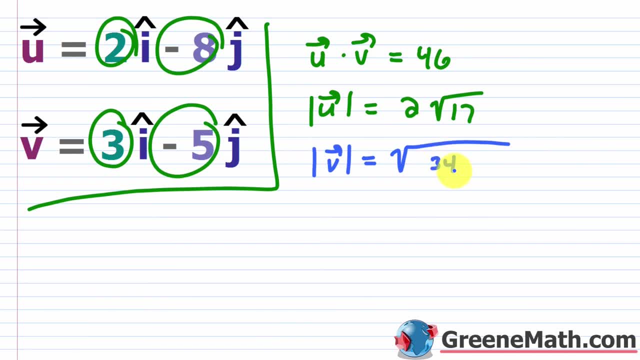 So this is going to be the square root of 34.. Now, you can't simplify the square root of 34, so let me erase this. I'm going to write this as the square root of 17,. okay, Let me write this like: 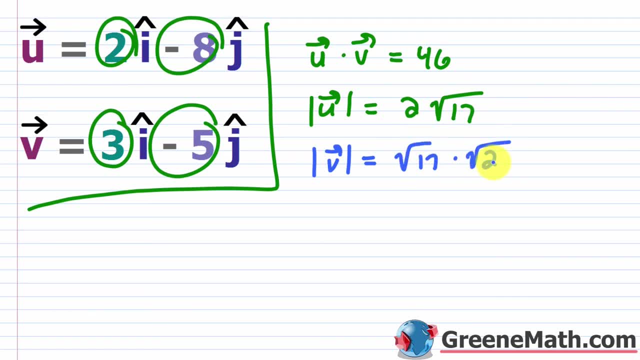 the square root of 17 times the square root of two, like this: okay, So let's punch into the calculator. First, let me do this: cosine of theta is equal to. again, you've got your dot product, which is the u dot v. okay, So the vector u dot the vector v over, you've got the product of these two. 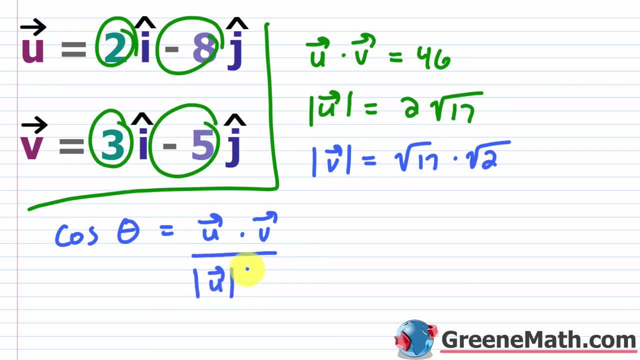 magnitudes. okay, So the magnitude of this vector u times the magnitude of this vector v. okay, And then if I plug in to my calculator, what I want to do is say theta is equal to cosine inverse of all of this. okay, So the dot product of u and v is 46 over you're going to have the magnitude. 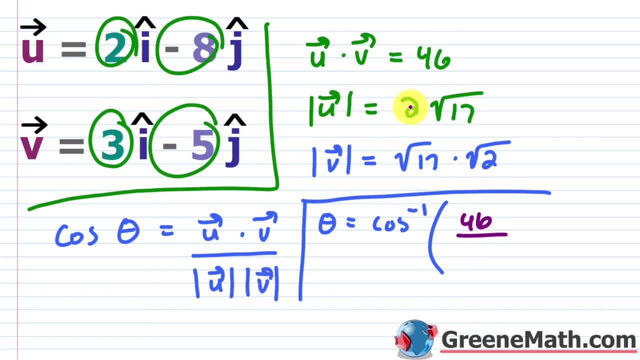 of u times the magnitude of v. So essentially what you have is two okay, times square root of 17. times square root of 17 is 17, okay, So that's just going to be 34, okay. And then times the square. 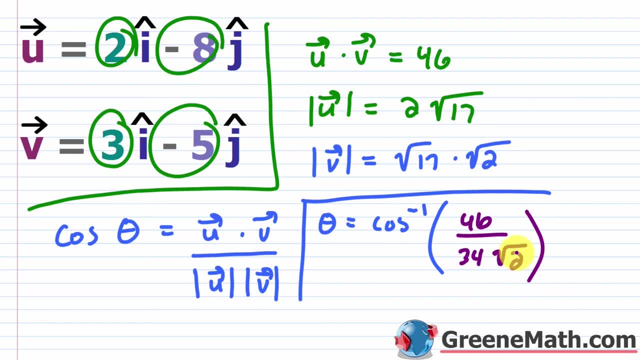 root of two. Now again, you don't have to go through all this. If you were writing this out on a test, you might want to. If you were writing this out on a test, you might want to If you were. 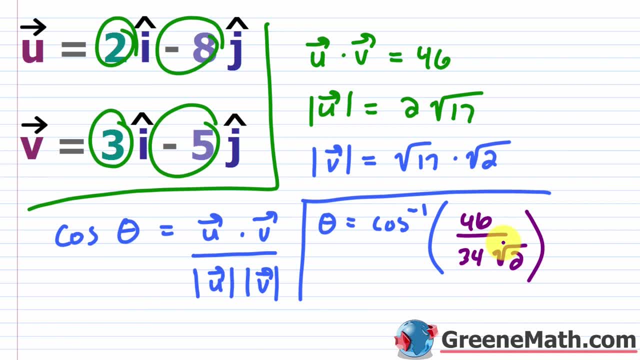 writing this out on a test. you might want to, But for the purposes of punching it into a calculator. who cares right, It's just going to work either way. So again, if you're having problems with this, wrap this in some parentheses, And if I punch this into my calculator, I get a. 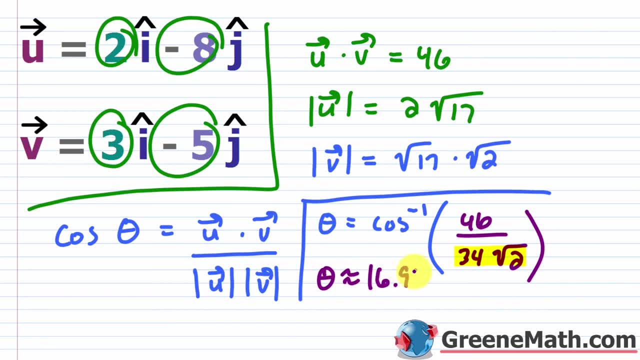 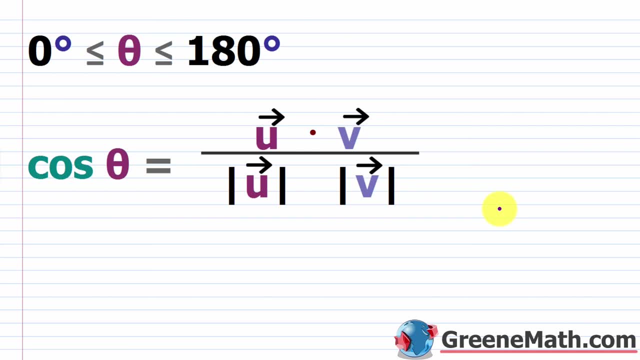 theta, that's approximately 16.93 degrees. All right, so before we wrap up the lesson, let's talk about the concept of orthogonal vectors. And this is just a fancy word to say that you have perpendicular vectors. okay, So they're going to meet at a right angle. So when the dot product for 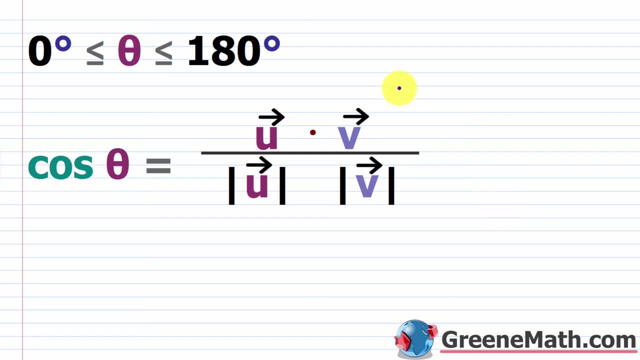 u and v is 0, then what's going to happen is the top part of this formula here is 0. And because you have non-zero vectors down here, the bottom part or the denominator will not be 0. So 0 divided. 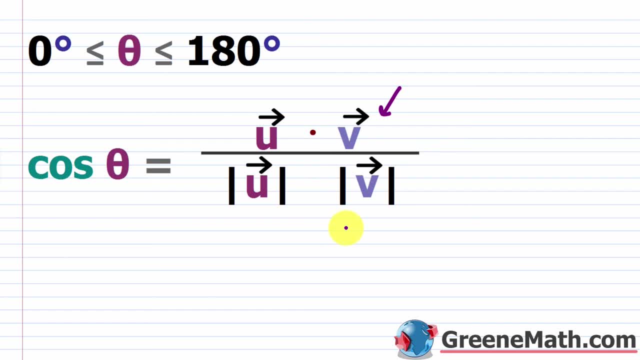 by something that's not 0 is always going to be 0,. okay, So then you could say: the cosine of theta is going to be equal to 0. And where does this happen? Again, if theta is greater than or equal to 0 degrees and less than or equal to 180 degrees, well, it must be true that theta is equal to 90. 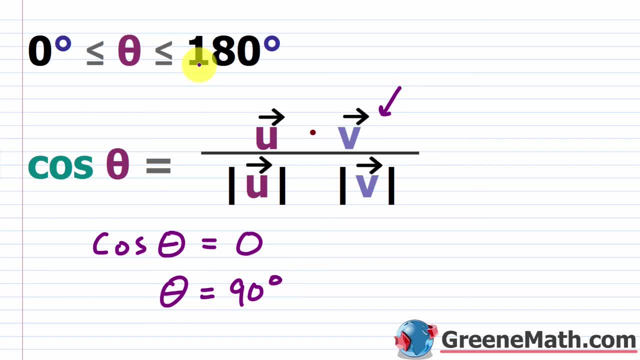 degrees. So the cosine of theta is going to be equal to 0.. So the cosine of theta is going to be: the angle between these two vectors, u and v, is going to be 90 degrees, meaning these two guys are perpendicular vectors or in the language of vectors we say they're orthogonal vectors. 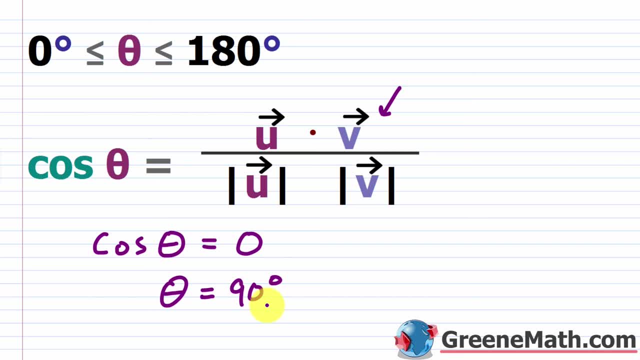 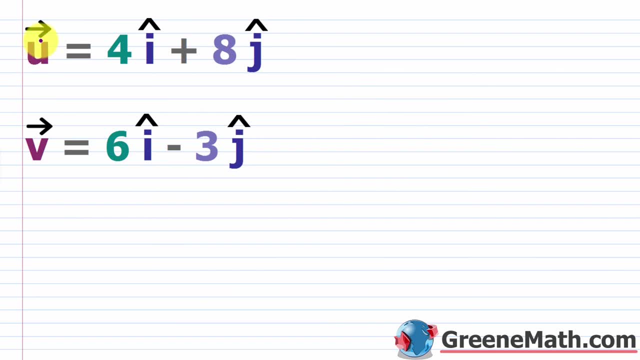 okay. So all you need to do if you want to check to see if you have these orthogonal vectors, is just do the dot product and see if it's 0, okay, That's all you want to do. So to start out this problem, I have this vector u, which is going to be 4 times the unit vector i plus 8 times the. 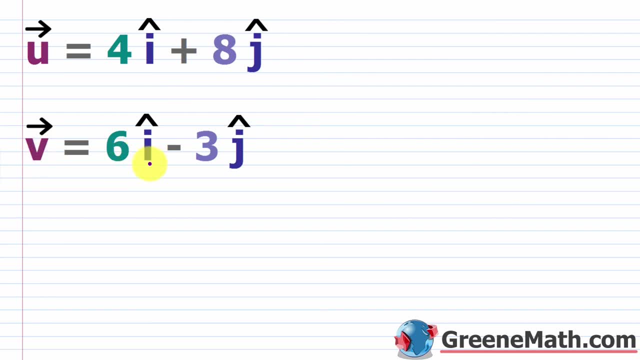 unit vector j. And then I have this vector v, which is going to be 6 times the unit vector i minus 3 times the unit vector j. okay, So if I wanted to find out if these two vectors were perpendicular or again, if they were orthogonal vectors, I can just find the dot product and see. 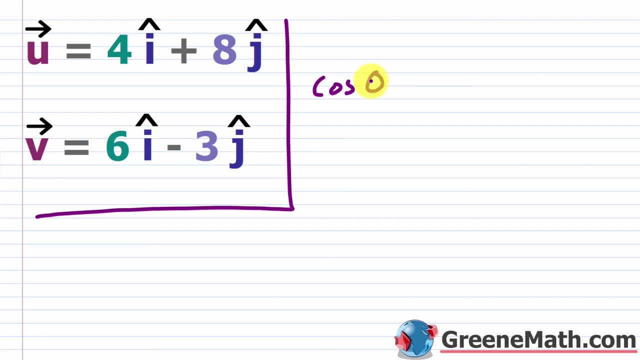 if it's 0, okay. So in other words, with your formula, cosine of theta is equal to, you've got your dot product okay, which is the dot product of u and v. so u dot v, okay. over the magnitude. 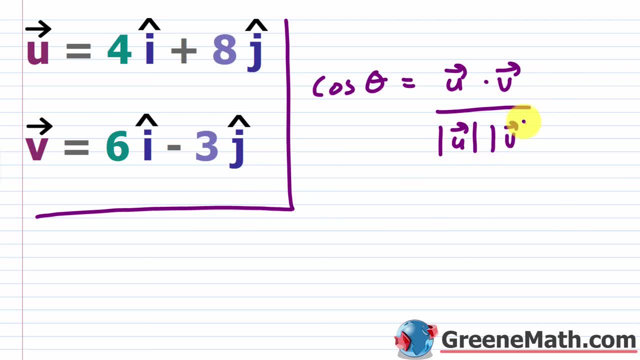 of this vector u times the magnitude of this vector v. okay, So we know this formula. at this point, Again, if this top part ends up being 0,, then we're going to have to do the cosine of theta 0, and these guys down here aren't 0,, which they won't be- well then the cosine of theta will be. 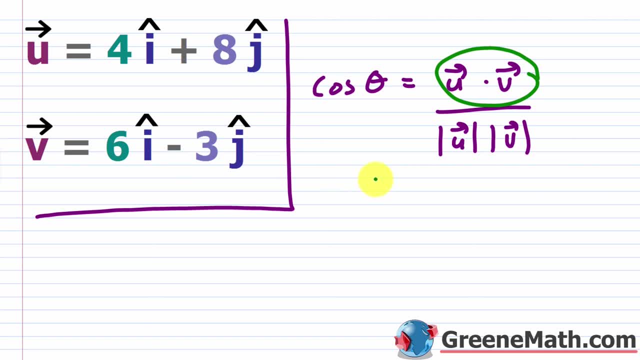 equal to 0, and theta is 90 degrees, right? So these guys are going to be perpendicular. So the dot product here- okay, we do u dot v- is equal to 4 times 6,, that's 24, and then plus 8 times. 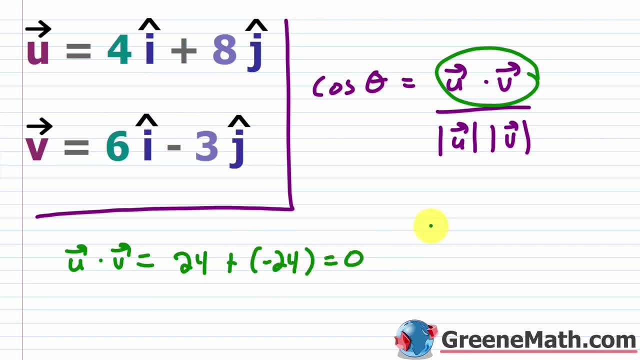 negative. 3 is negative 24.. So of course this is 0, right. So again, this top part would be 0, the bottom part wouldn't be 0, you can go through and find the magnitudes multiplied together. 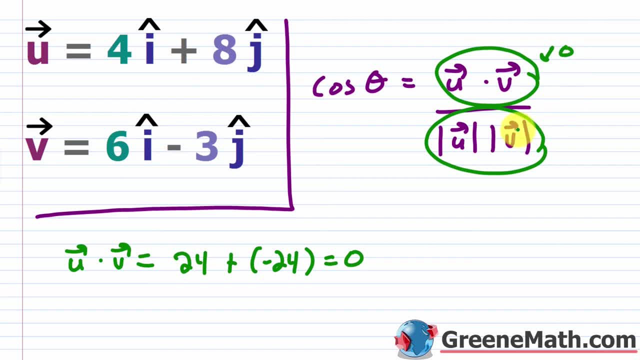 and you'll see that you're still getting 0, right in the end. So 0 divided by something that's not 0, you just get 0, right. So the cosine of theta is going to be 0, so theta equals 90. 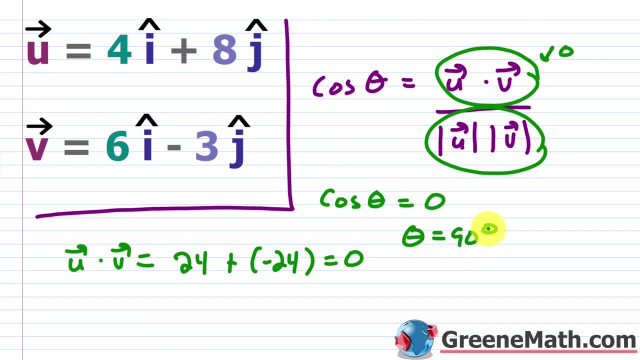 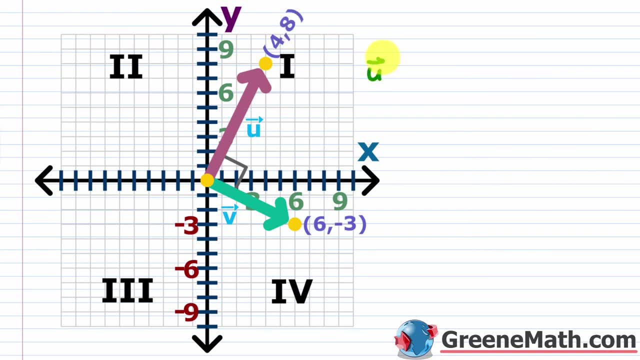 degrees and, of course, we have perpendicular vectors. If you want to see this, your vector u- okay, which we have right here. the terminal point is at 4 comma 8, right, Because, again, this vector u was set up as 4i. okay, that unit vector. plus. we had 8j, that unit vector, okay. 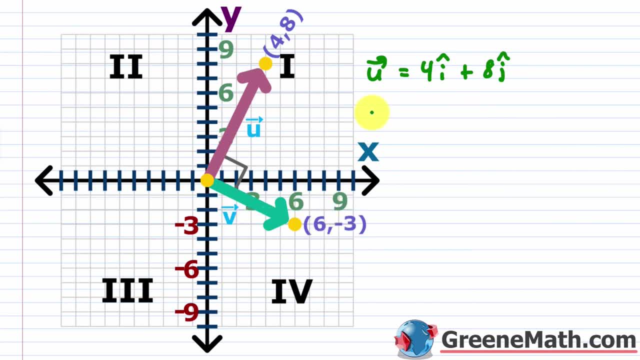 And then for the vector v, the terminal point was at 6 comma, negative 3.. So here's the vector v to have this 6 times the unit vector i plus, you're going to have this negative 3, or might as well. 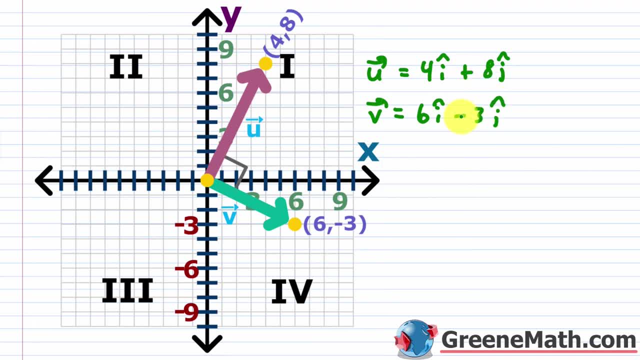 just write minus 3 times the unit vector j. okay, So this is how we set this up. So this guy has a terminal point at 6 comma negative 3,. this guy has a terminal point at 4 comma 8.. You can see this. 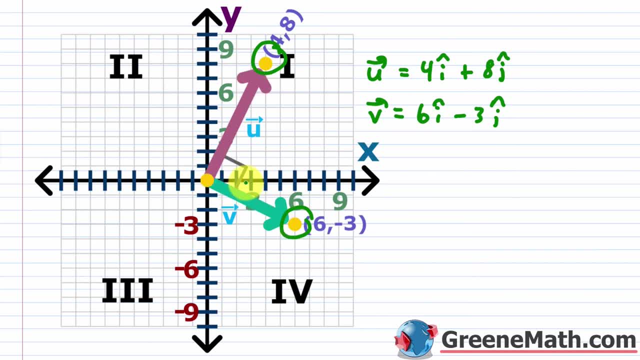 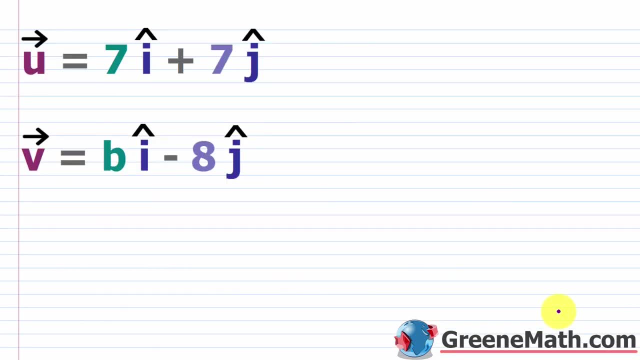 graphically that they're going to meet at a 90 degree angle and therefore, by definition, these guys are perpendicular, or you could say they're orthogonal vectors. All right, as a last example, what if you had something like this? So we have our vector u. 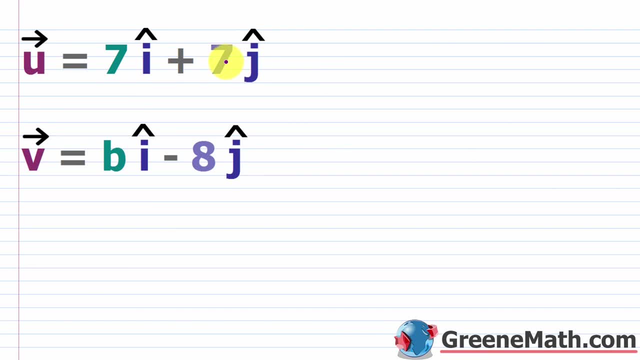 and it's equal to: we have 7 times the unit vector i plus 7 times the unit vector j. Then we have this vector v and it has b okay some unknown times- the unit vector i minus 8,. 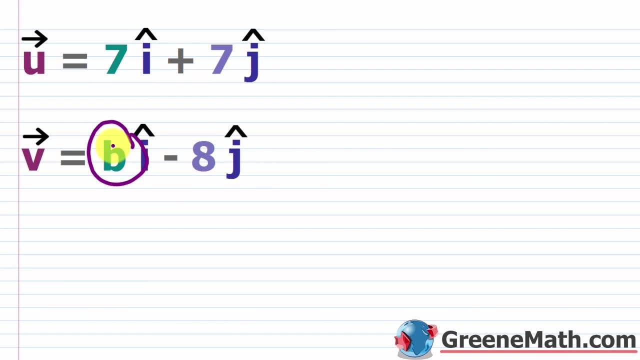 times the unit vector j. How can I find a value for b such that the two vectors, u and v, would be orthogonal, or you could say perpendicular, vectors? Well, all you'd want to do is just set up your little dot product. okay, So the dot product of u and v is going to be what? 7 times b? 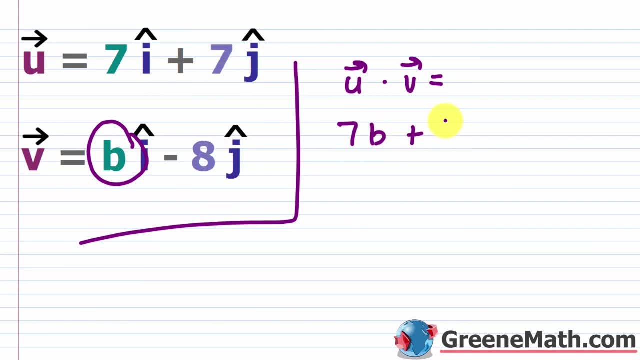 and then plus you're going to have 7 times negative 8, which is negative 56. So you really need this guy right here. you can just substitute this with a value here. You really want this to be zero. let me just do this down here. So you really want this to be zero, so that those guys